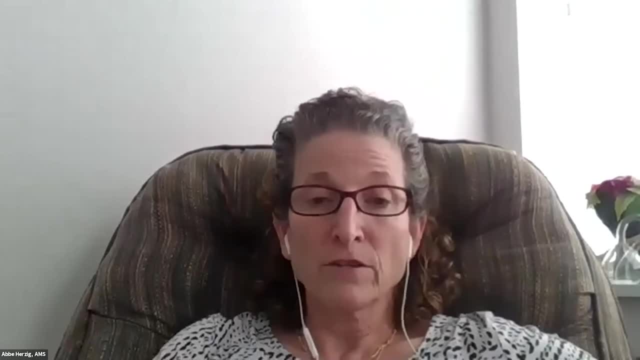 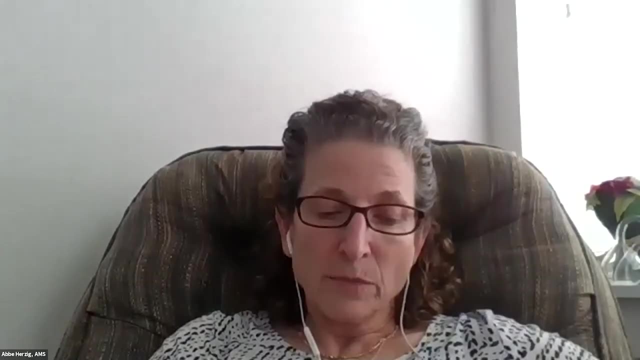 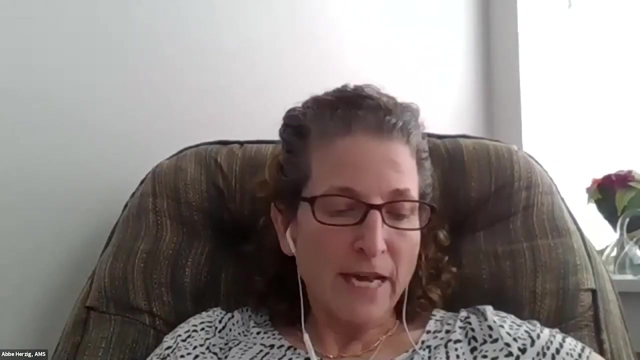 design since 2005,, but she's taught learners of all ages and in all modalities. Tonka specializes in faculty development, online course accessibility and motivation in online education. She has co-authored and designed several MOOCs through the Coursera and Canvas platforms. She considers 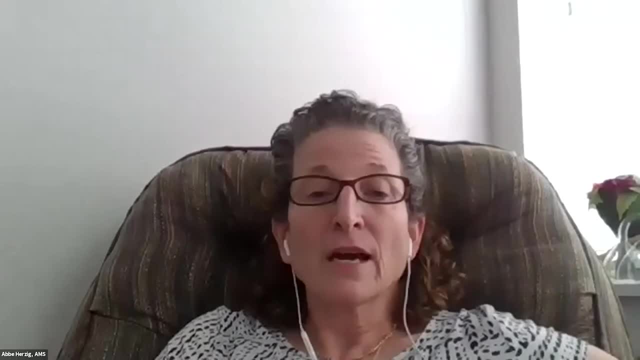 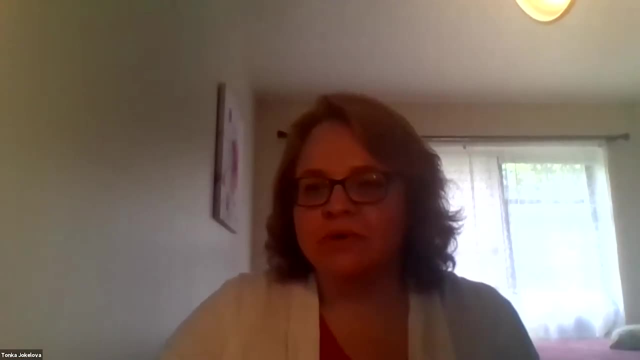 education, her profession and her passion. And with that I will turn it over to Tonka, Thank you. Thank you, Abby, for the introduction. Good afternoon everyone. Just like Abby said, my name is Tonka Yokolova and I am the Director of Center for Learning Design Innovation. 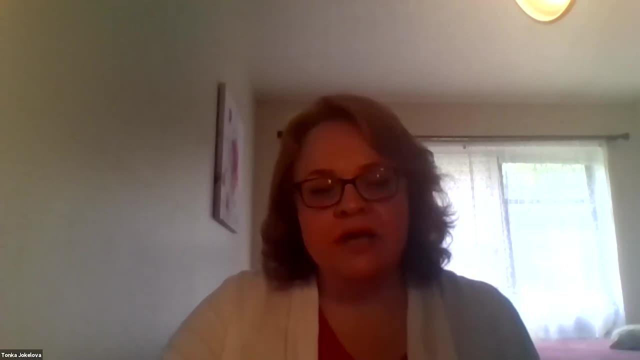 and Online Instruction at Canton. Today we will talk about engaging students in online classes. I know many times I hear instructors saying: well, it's an online class, We can't really have interaction, We can't really have social engagement, We can't really have all. 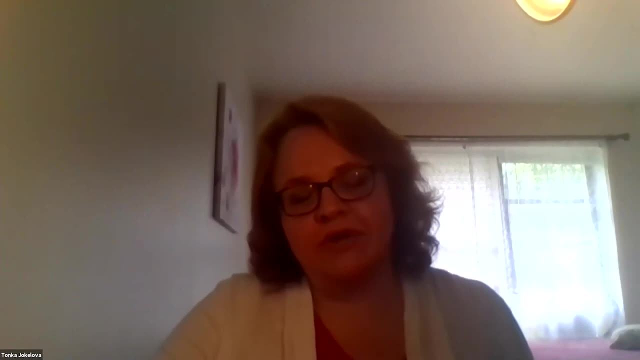 that social fluffy things that we usually have in regular courses. So hopefully, before we leave today, or hopefully before you leave today, you'll be convinced otherwise And hopefully I will be able to give you some practical strategies that you can take into your courses today and use them with your students And, hopefully, the strategies that 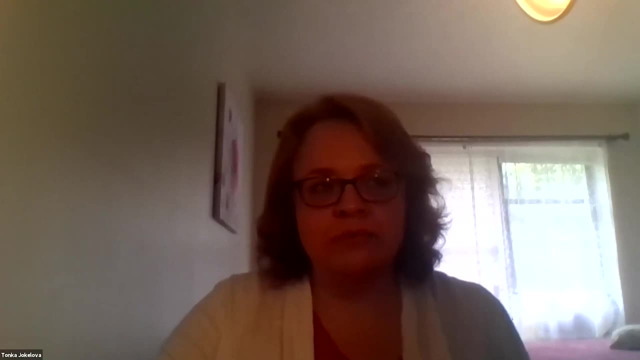 I'm going to talk about or we're going to talk about. hopefully they're not too time consuming and easily understandable and easily memorable so that you are able to just jump right in and start your design, your course design concentrated or focused on student. 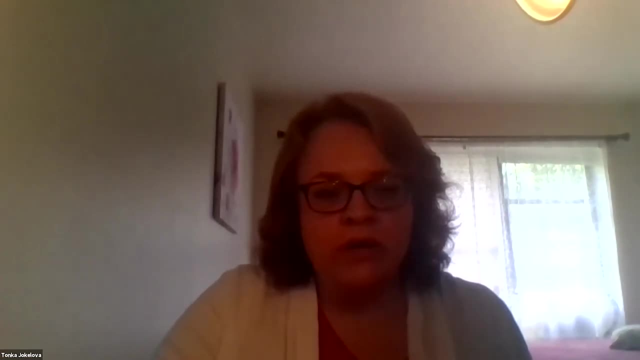 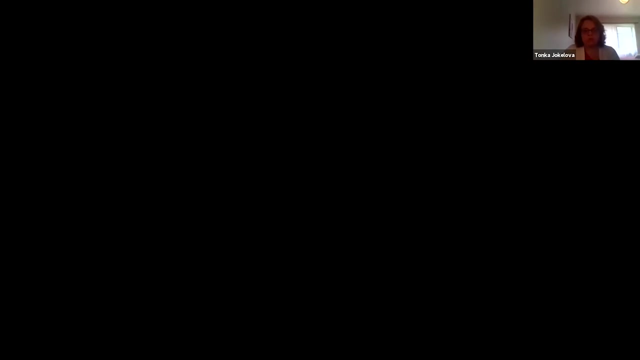 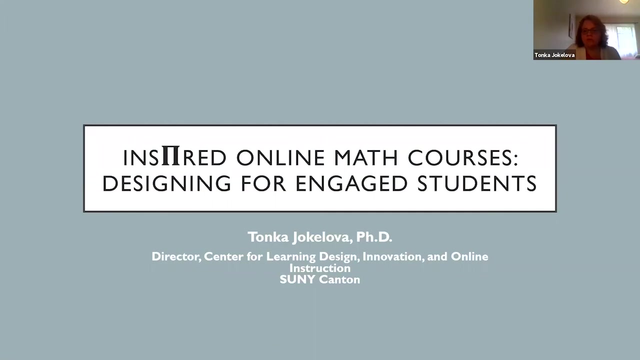 engagement, So let me share my screen with you and we'll get going. Give me just one second please, All right. Okay, Screen two: All right. Are you able to see inspired online math courses designing for engaged students on your screen? 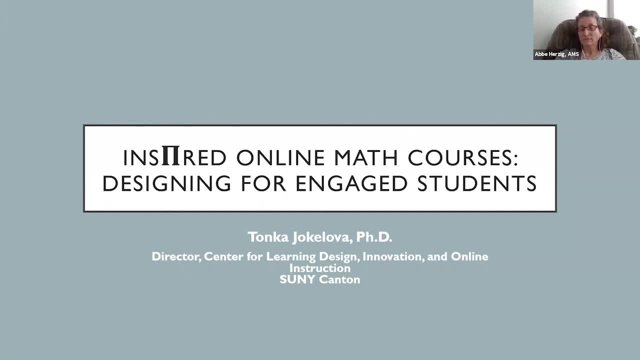 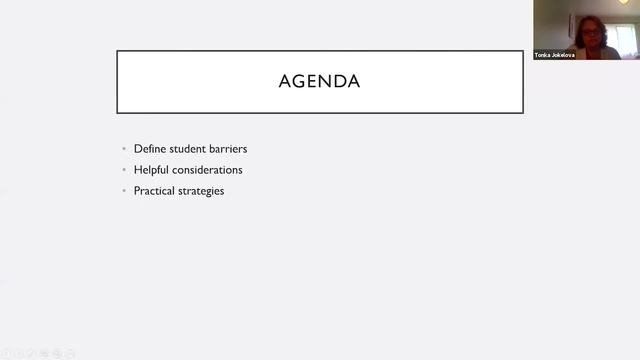 Yes, Wonderful, Thank you, And I'm trying to get myself back into Zoom because I have several windows open and I lost you in my windows. Okay, All right, Very good, So let's go on and start with the agenda today. 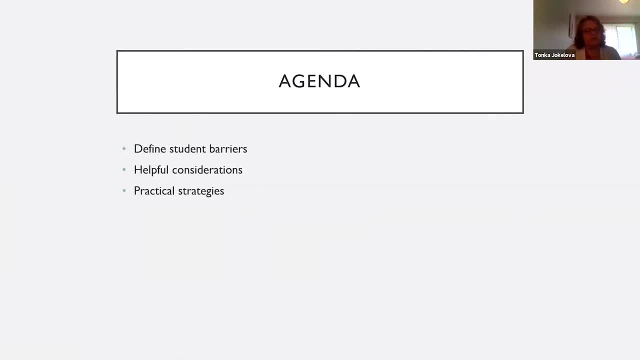 We will define some barriers that our students have or have had, and hopefully will not have, but probably will have, when it comes to teaching in fall and when it comes to teaching in this whole new world that we are living in. We will 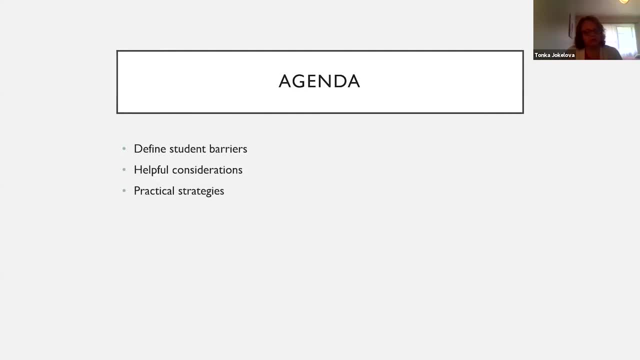 also talk about some considerations that we can think about as we are designing our courses, and we will also talk about some practical strategies, just like I shared. So let's move on. Before we do, though, give me just one second, Let me. I'm trying to. 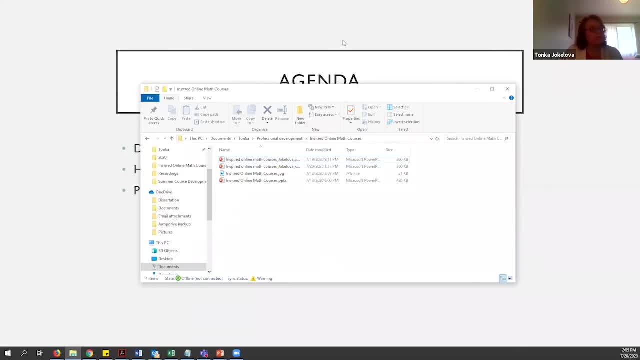 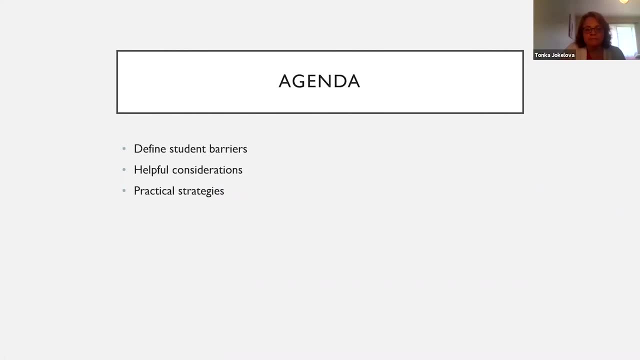 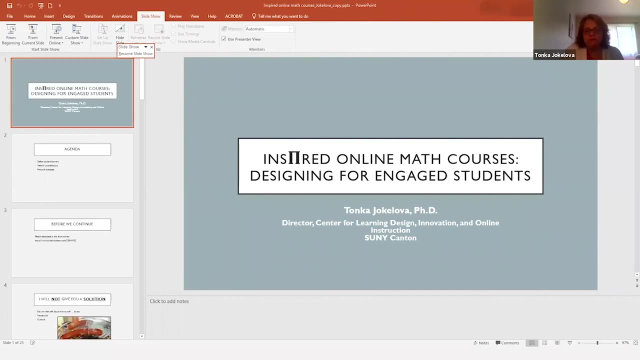 that's not running me. Give me just one second. I'm trying to get us a survey link into the chat area, so give me just one second. There we go. All right, I have a survey link. I have a survey for you that I would like, I would like for you to take. Let me get into the. 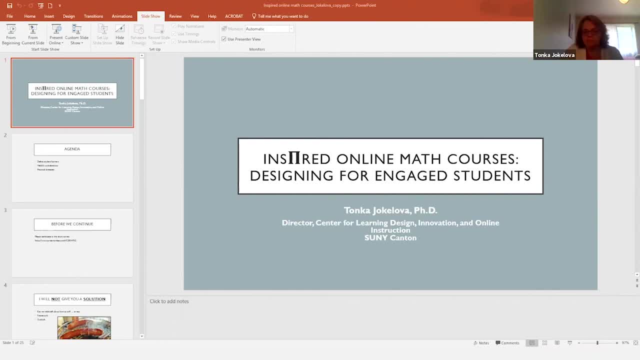 chat area. We're not able to get into the chat area. I wonder If you hover over the bottom. All right, Let me stop sharing or post-sharing right now and see if I can. if I can do it that way, All right. 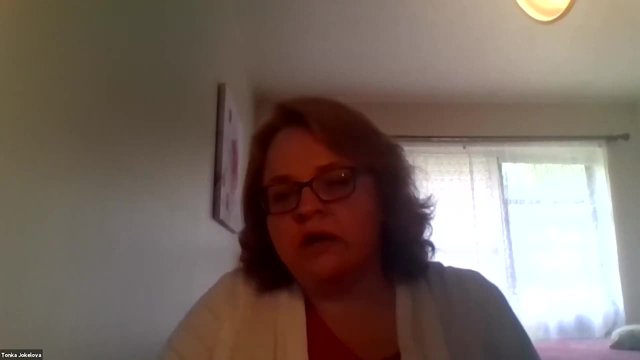 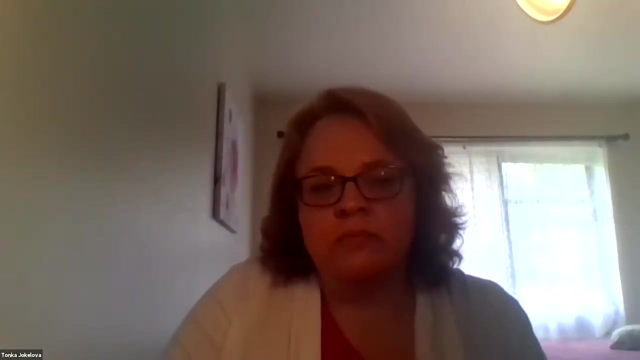 So here is the link and let's take maybe- I don't know- a minute or so to to take the, to take the survey, to take the questionnaire. I'm going to pause for a minute and then we'll come back. 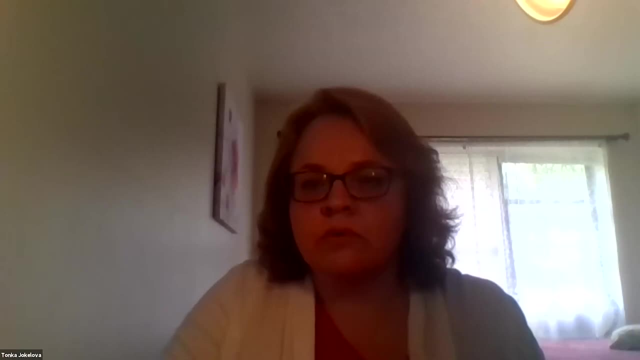 Oh, okay, Give me just one second. Thank you for all attendees. There we go. I posted it to the wrong chat. You should be able to see it now. It's the SurveyMonkey link. Yes, it should be out there for everybody. 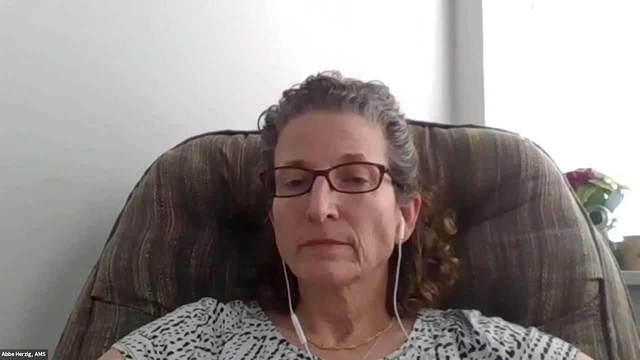 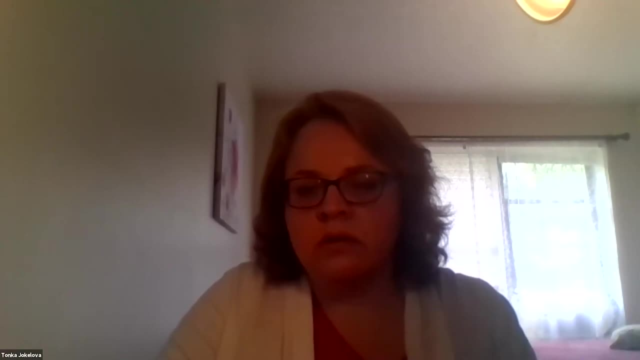 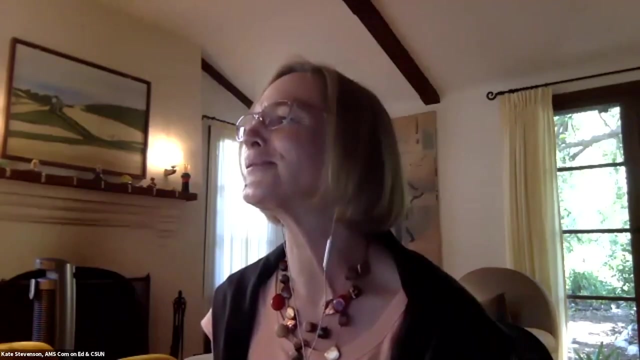 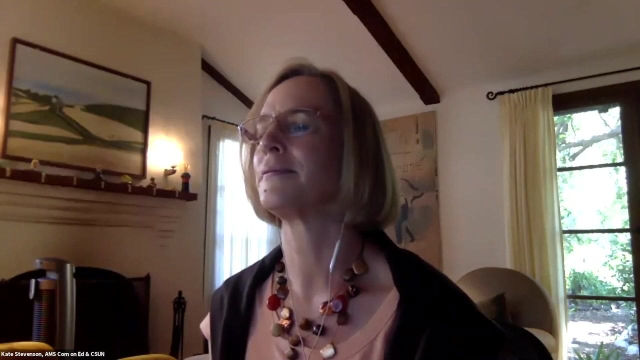 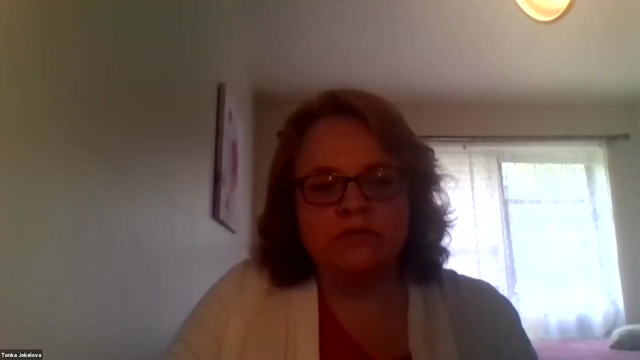 Okay, thank you, Perfect. Thank you, Heather. I can see that it's filling in. Okay, good, All right, so I took the survey as well and I'm going to share my screen. I waited, I waited a couple of minutes, a couple of seconds after you, so that we're seeing, hopefully, one of the one of the final results. 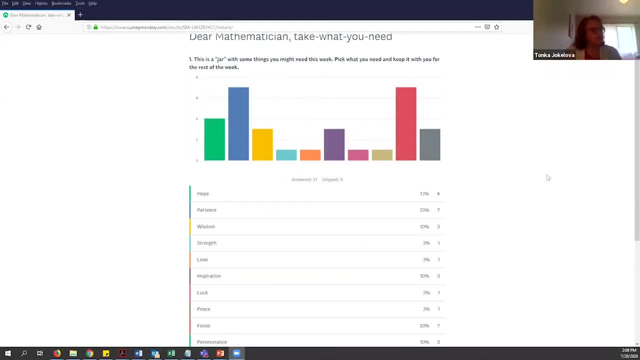 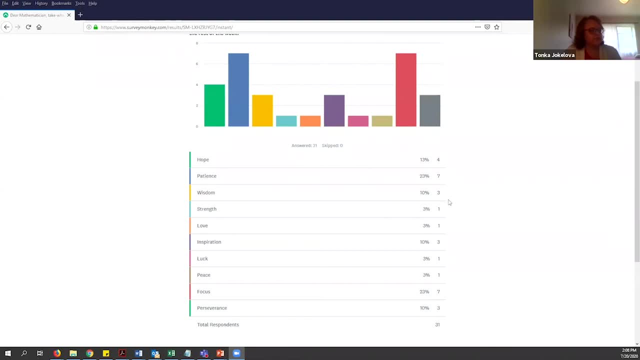 of the survey. So we're seeing that we- most of us- need focus and patience, And then the next what we need is hope. Okay, so I'm wondering: focus and patience. why do we need patience? and in this time? is it because all that is happening at our colleges and we are not quite sure how the fall will be, and we need to be patient because of that? 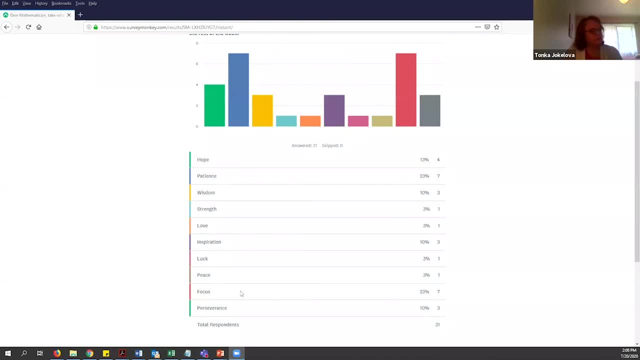 Is that what you want? we need patients. Why do we need focus? Do we need focus because we need to get the courses ready and we have summer going on and we have pools and ice creams and walking outside and just enjoying summer. Do we need focus because of all the all the priorities that are kind of tugging on our 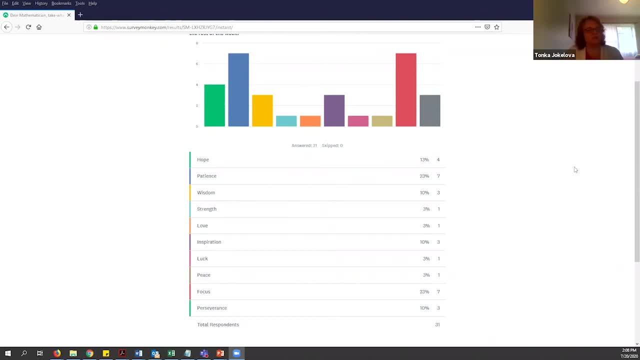 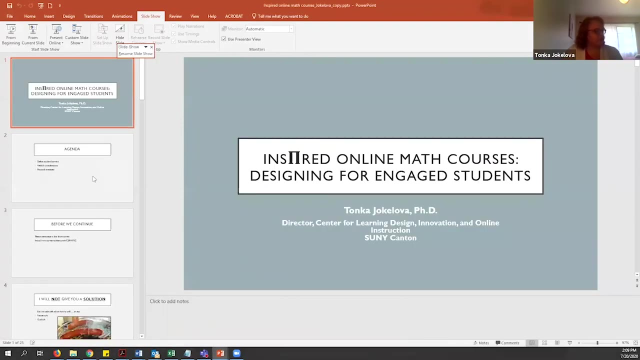 time. I wonder: why do we need a lot of focus and a lot of patience? I don't think we're going to analyze this a little bit more right now, but keep that talk in the back of your mind and we'll come back to this, to this question, a little bit later. So let me go back to to sharing the the presentation. 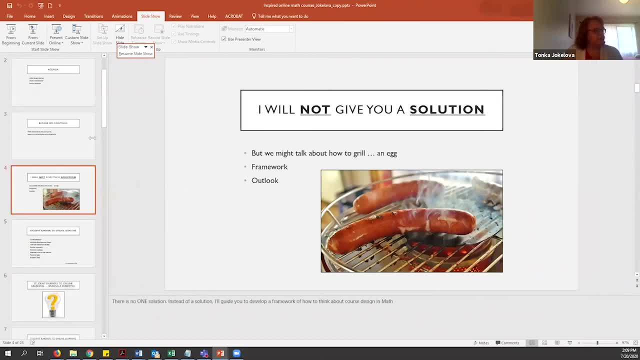 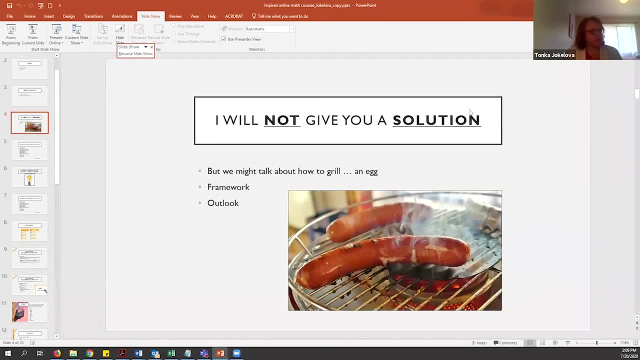 and we'll talk about. I'm going to keep it this way, I'm going to make it larger, So I will. today, I will not give you. are you seeing? are you seeing my grilling uh picture that says I will not give you a solution? okay, good, thank you, Kate. so yes, I will. 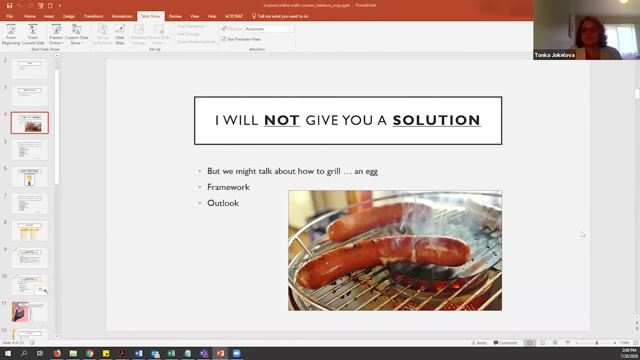 not give you a solution today. I will, because there is not one single solution that I, anybody, can give you, but what I will give you is I will give you some framework of how to think about course design. I will have you, hopefully, different outlook on how to think about course design when it comes. 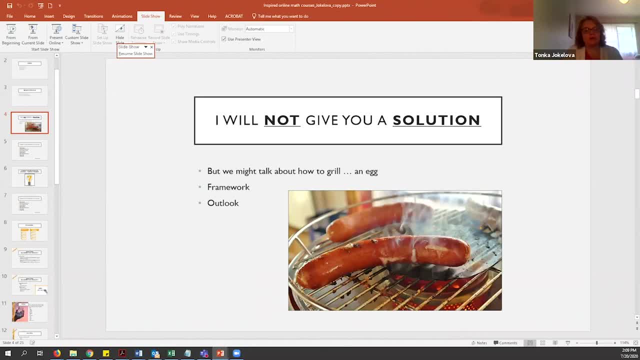 to student engagement when it comes to designing items and elements that will give the student that that push just to, just to try a little bit harder, just to be more, a little bit more in the course. and also I will not, um, I will not deny or admit that we will talk about, uh, grilling and grilling. 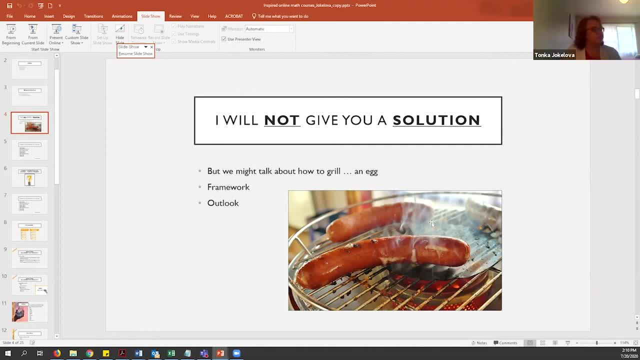 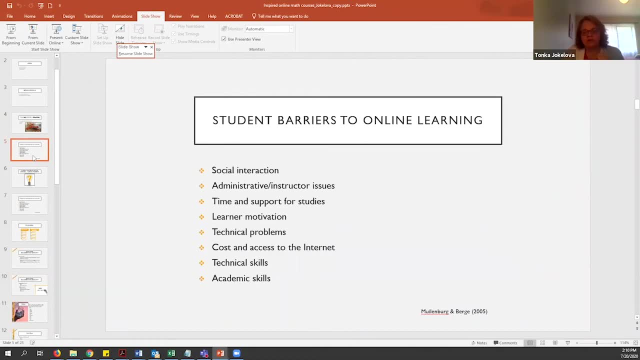 an egg. so just think about that and we'll come. hopefully we'll come back to it later as we as we go. all right, so, um, there was a study in 2005 and it was. it was replicated in 2015. um, uh, there was a factor analysis of student student barriers to online learning and they found out. 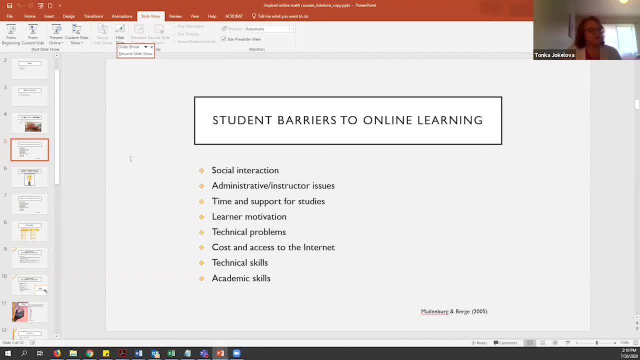 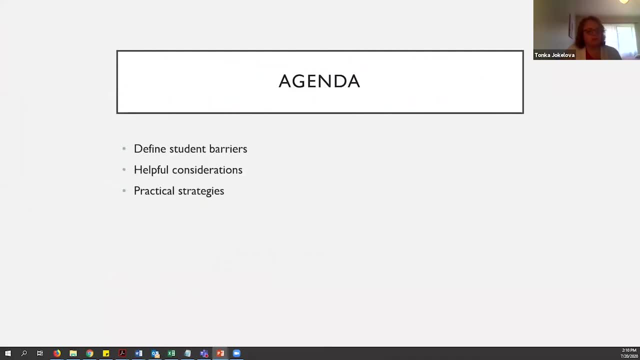 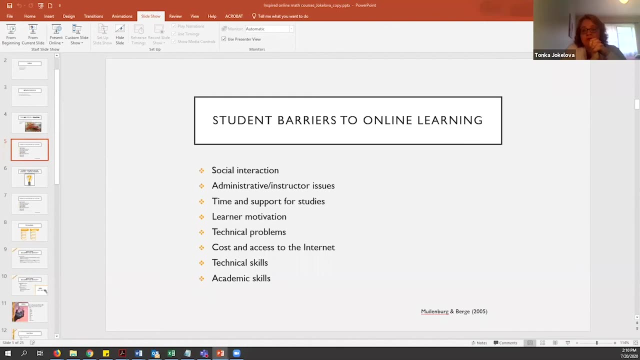 interestingly enough, that number one barrier to online studying or students completing online courses is, um, oh, okay, hold on, give me one. second- is a lack of social interaction. so I thought it was. it was quite interesting because you would think that probably, uh, internet being slow, or 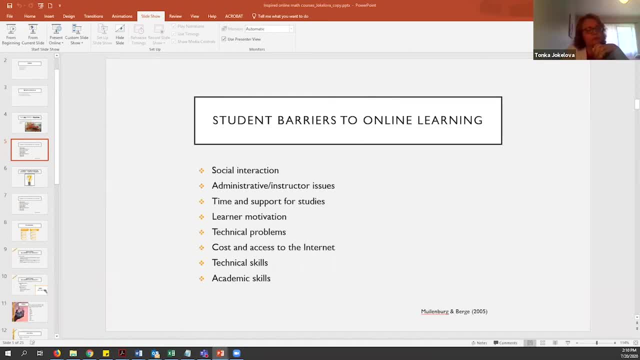 not having good time management skills would be number one, but no really social interaction was cited was found to be number one barrier to students completing online courses. some other barriers, interesting enough, where instructor issues, meaning a structure might not be present- administrative issue- I could not get into the course- and all the technical stuff. time and support for studies. do we, do I have time if 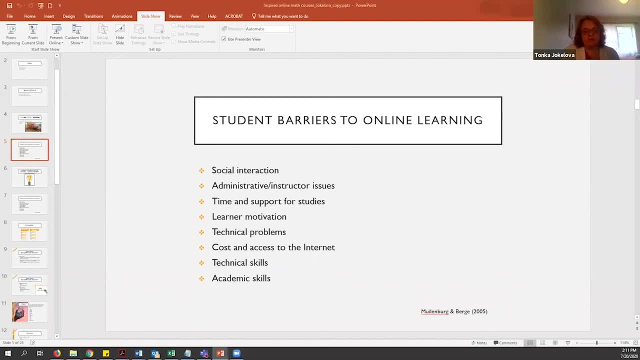 this is a non-traditional student. I probably have several other priorities that are that are competing for my time. I think the need for the student is to have a level of learning or in the course structure, or a level of communication, and it should be the first thing that ships in the class. 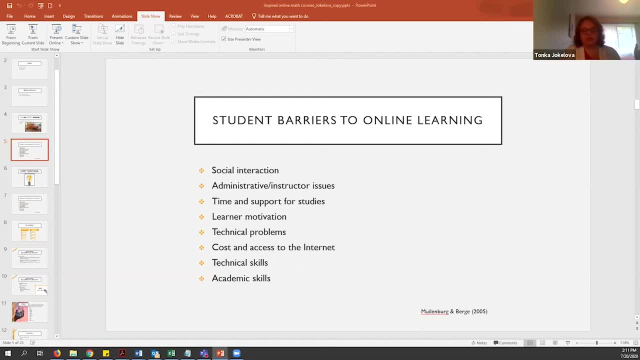 um, it has to be the topics of the class, it has to be the subject matter. they have to be not only the subjects that become the subject matter, but also the course subjects. the subject matter allows them to be the subject matter. so you want to have some interaction and um, but um. 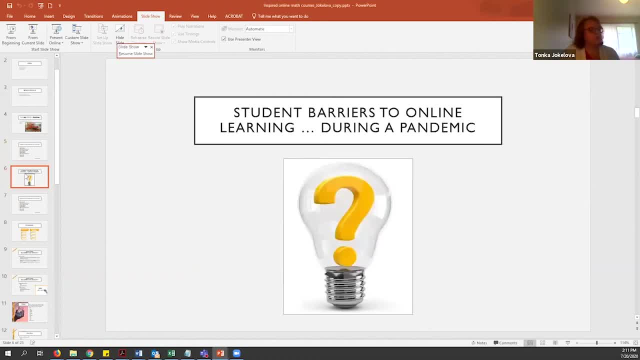 maybe those barriers that we mentioned about things like learning, motivation. number four: that was really interesting as well. I was really surprised with number one and really surprised with the same. Do you think they will move around? Do you think there will be new barriers that come to? 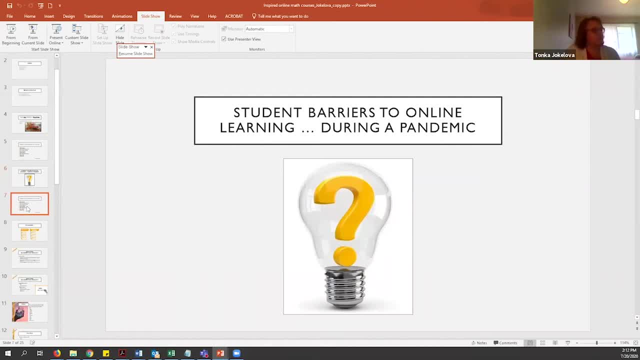 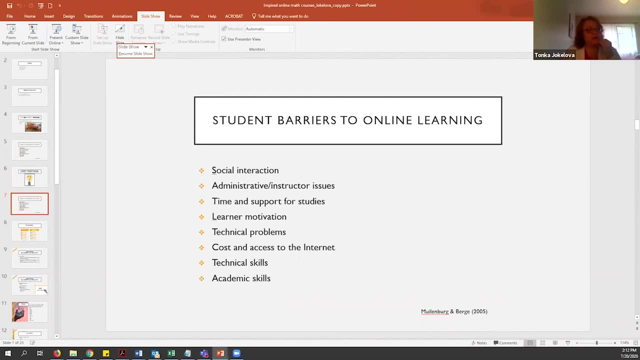 play. Where do you think we will be in the fall? There's a question in the chat about whether those are in order. Yes, they are. Thank you for a great question. Yes, they are. Number one is social interaction, Number two admin and all that. Yes, that is the number of significance. 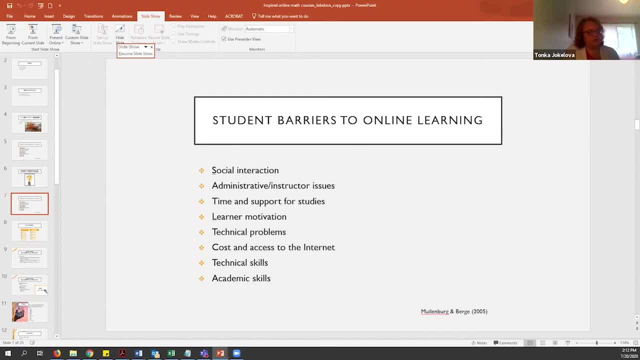 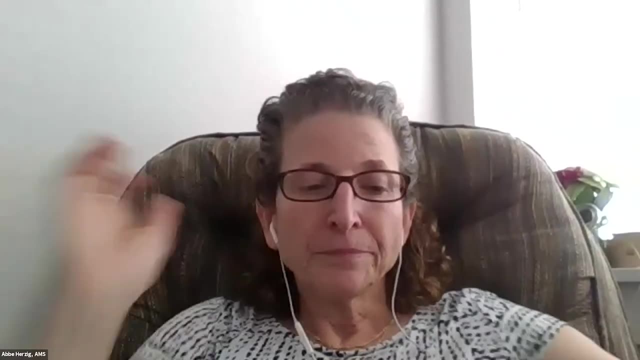 So then again, I'm having those barriers on the slide. Where do you think we will be? I'm going to stop sharing for a minute and go to chat so that I can monitor where you're thinking where we will be in the fall, Or we can read them to you if you'd like. Oh, okay, Either or 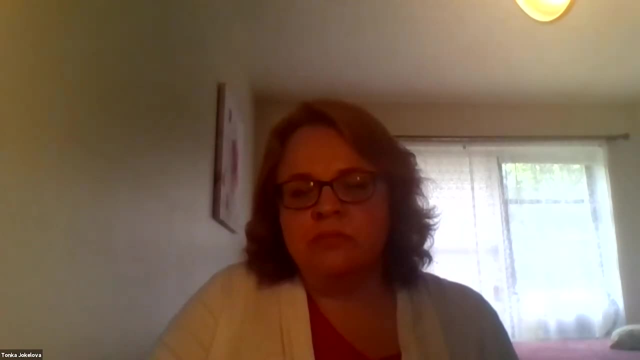 So in the chat, or grab your microphone if you're able to, you think that we'll have the same issues. Carolina thinks that we'll have the same issues: Learning, motivation, time management. Heather thinks we'll be probably more up top on the. 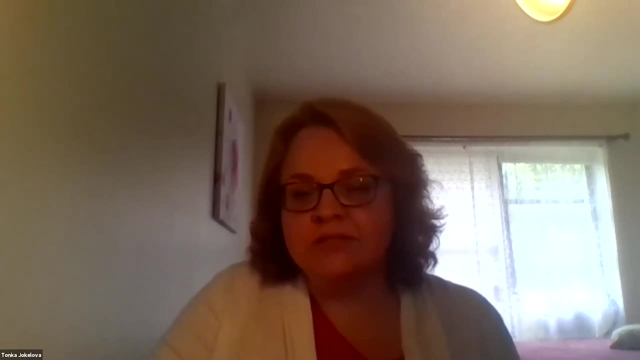 social interaction, We'll stay high on the list. Issues with COVID illness. for sure, Learning motivation will be number one. That's one of the things. Okay, Social interaction, for sure, I do believe I agree with you. I do believe that I'm going to start sharing again. So what I believe. 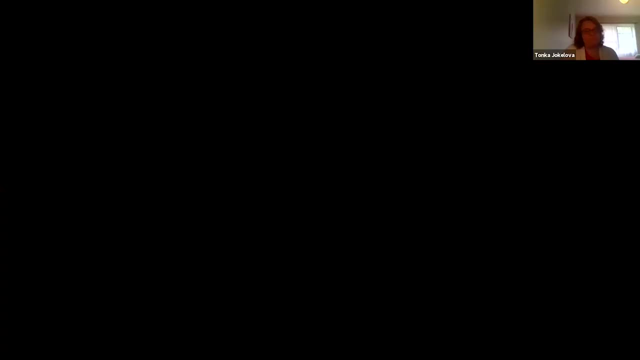 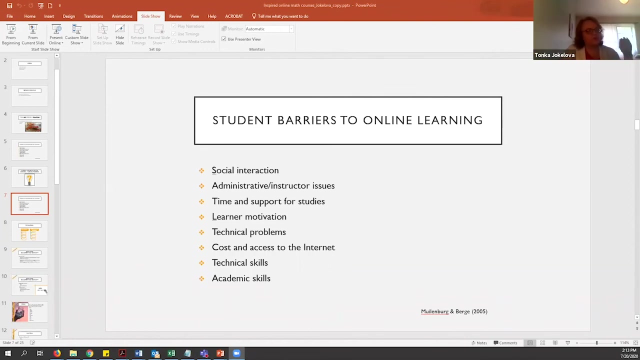 is that possibly the cost and access to the internet, technical problems might go a little bit up on the list. That's what I'm thinking, because for my own college I'm seeing that not everybody has good equipment, Not everybody has good access to internet. There are families that have one computer and three students that have to share. 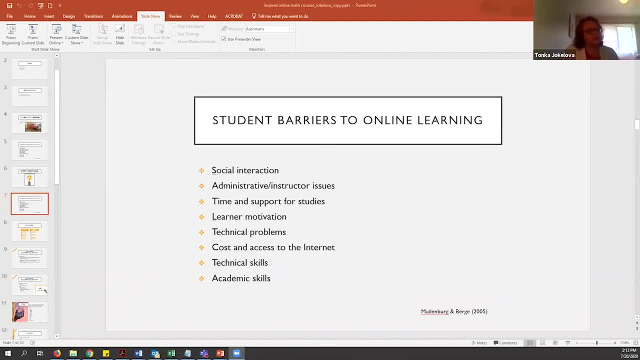 one computer at a time. So I'm assuming the cost and internet will go a little bit up. I'm also assuming technical problems will go a little bit up because there will be new, newly online courses that were not online before, So there will be technical problems associated with. 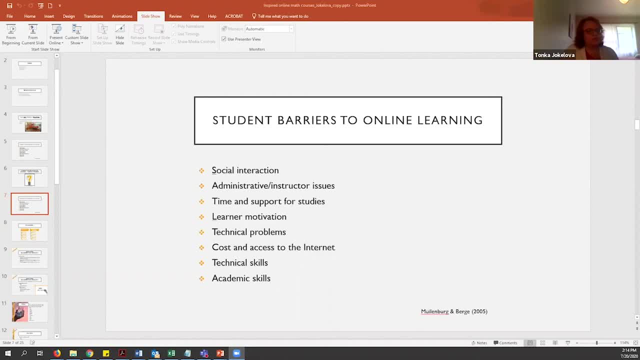 that. But just like somebody said in the chat, I do believe social interaction will stay number one. I do believe, now more than ever, social interaction is very important to students because I believe if the course is designed well, the instructor can take it to another. 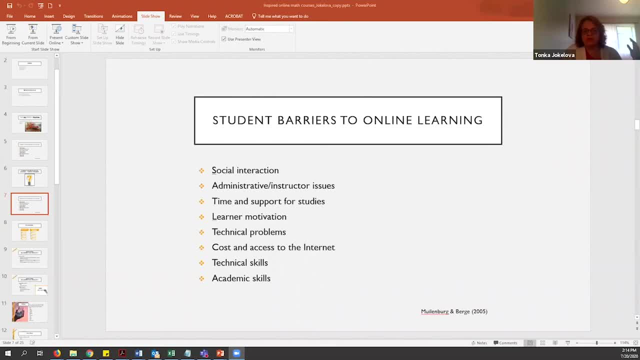 level. If the course is not designed well, the course is not going to go up. in fact, in course, instructor still can save the day. However, if the course design is fantastic and everything is just what, do they call it? Bells and whistles? Yes, bells and whistles If the instructor is. 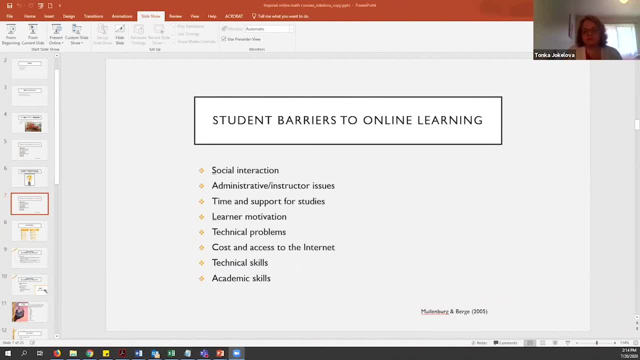 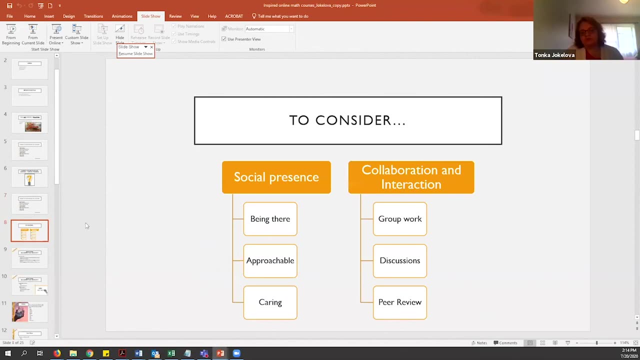 missing. the students still don't have the experience, The students still are not leaving with the knowledge they're supposed to be leaving with. So I do believe that social interaction and special interaction with the instructor will be number one, And so just to consider for that, 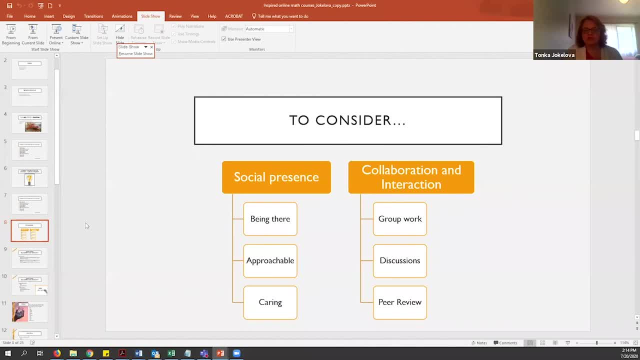 social interaction and learning motivation aspect. just to consider some of the aspects we will talk about today, I grouped them into two groups: social presence aspects and some collaboration and interaction, even though you can argue that collaboration and interaction is a subpart of social presence. but I kind of laid them out. 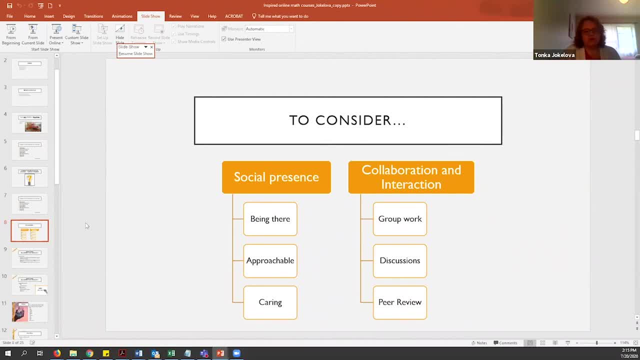 later separately. So for the social presence, we will talk about how you can be there and how being there for you as an instructor and, of course, developer, is very important. What are some strategies to make yourself look and feel and present approachable and caring, And also for 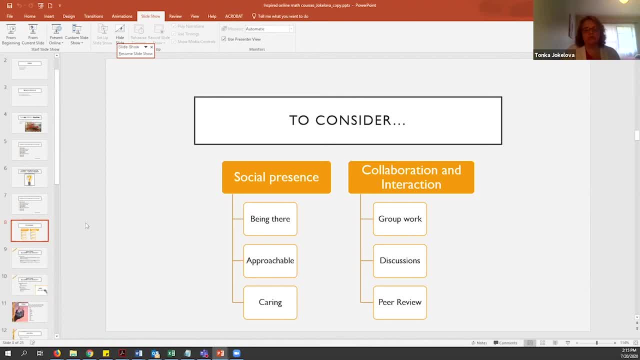 some of the strategies to enhance the social interaction and to make sure that students have opportunities to be engaged. those strategies we'll discuss, And they are group work, discussions and peer review. So, again, those are not the only elements that you, of course, should have under any stretch of imagination, right? Those are just something that can be an addition to what you are already doing. You already know that you are to meet. 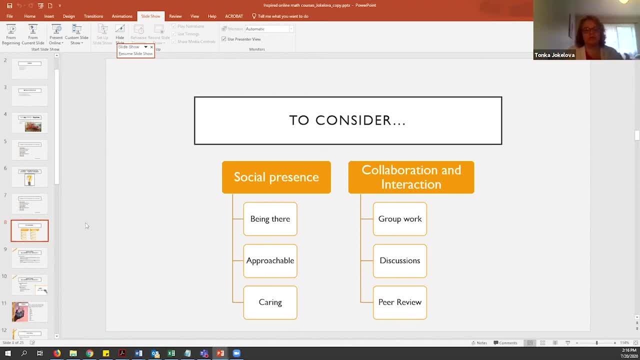 learning objectives. You already know what to design, what to teach. You already know all that. What I'm going to, What we're going to discuss today, is something that is that little bit of extra that your student can use to get a job. 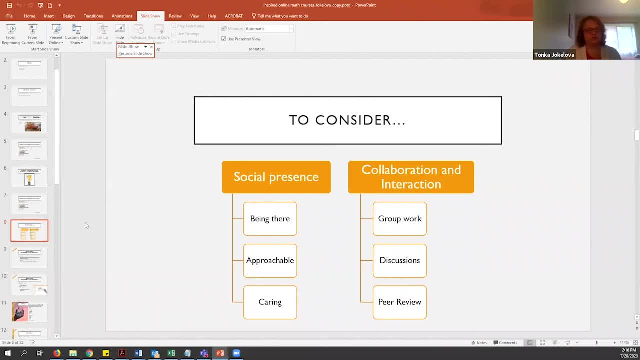 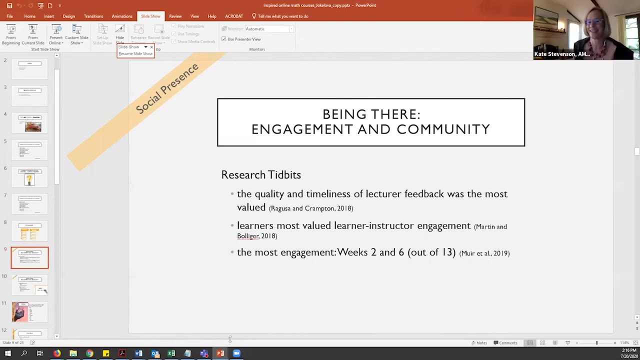 are looking for, especially now, in the era of this new teaching, that engagement, that interactivity with the student, that closeness, the sense of belonging, all of that All right, so let's talk about being there. Excuse me, Tonka, Go ahead, Kate. Now I've got the barking dog. 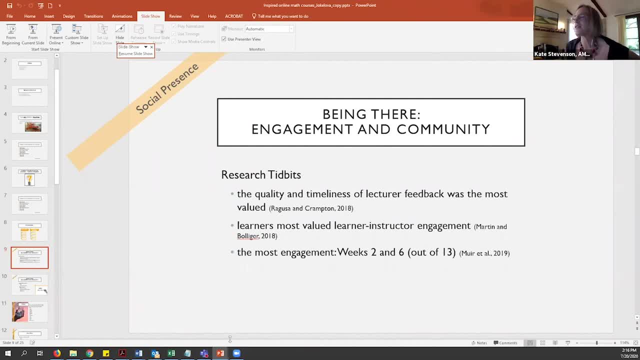 So there's a question in the chat that says: are you making a difference between online and remote instruction? I am and I'm not, because as long as you are not in the same classroom with the students, you are apart. So, whatever the apart is, you can be online and you can be remote. 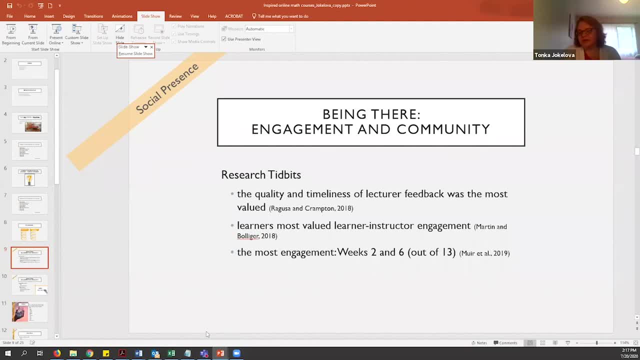 either or Somehow. I believe that, going towards the fall, we should be more of a, less of a remote. I know remote was a term used during the spring because it was such an emergent- emergent In transit into- not transit transfer, rather into online- and it was more of a. 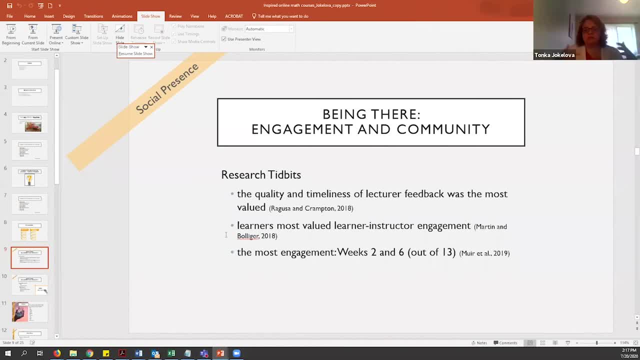 either fully online or it was synchronous online, or it was all kinds of combinations of modalities. So I know that's why we were using remote, and also remote was more of a emergency type of concept. I think we're moving from remote into the online, even though it's not fully online. 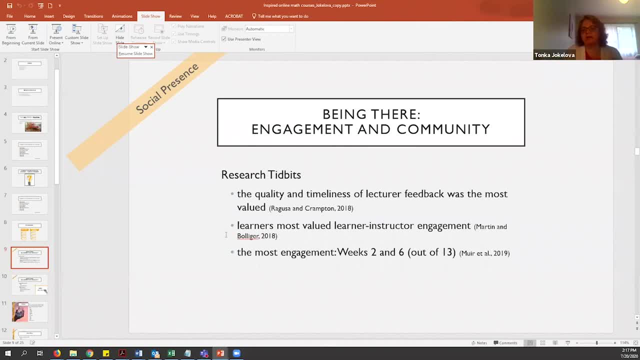 even though it's not fully synchronous. there is some kind of version of online And At SUNY, the whole system that calls that combined online. right, the online can be online synchronous live lessons or live sessions combined with some asynchronous modules. That's all. that's all what they call online. So 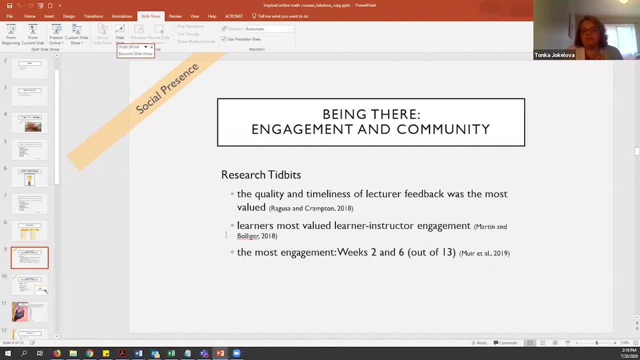 I don't think there is a. there is a. The topic today does not distinguish between remote and online. The strategies that we'll talk about can be used in both. So I'm thinking. I'm thinking yes and no, I'm not really. 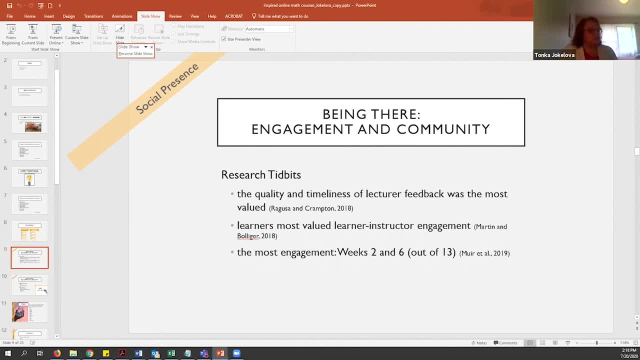 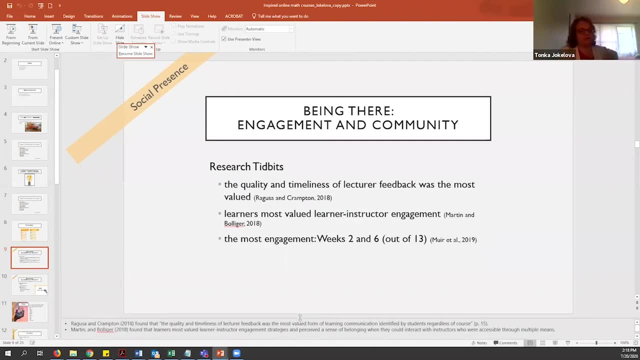 Not really distinguishing, even though you can Alright. so For the, for the research I thought you would find you would find it interesting, and I actually have the quote here, So I'm going to cheat a little bit. I'm going to read the exact quote. 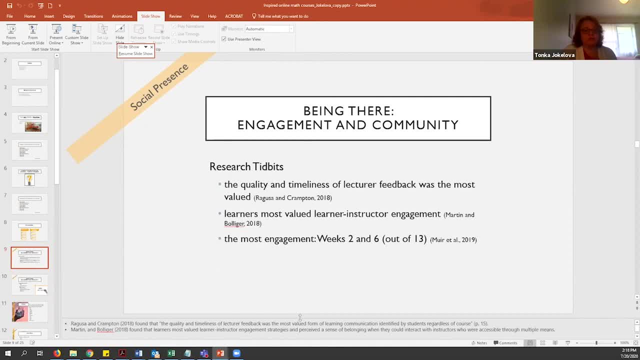 From from the studies that I found, which I thought was really eye opening to me. So, number one, the claim that I'm going to make is that you, as an instructor, are the number one, number one factor of students', number one, number one factor of students'. 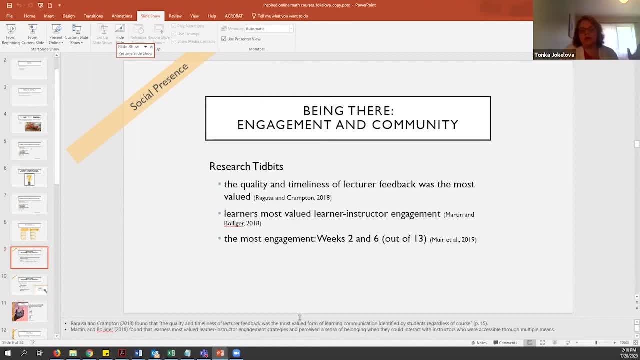 engagement. It is not a student to student interaction. It is not student to materials interaction. It is between you and the student, between the instructor and the student. And I have two studies to support that. So first study that I'm going to very briefly give you: 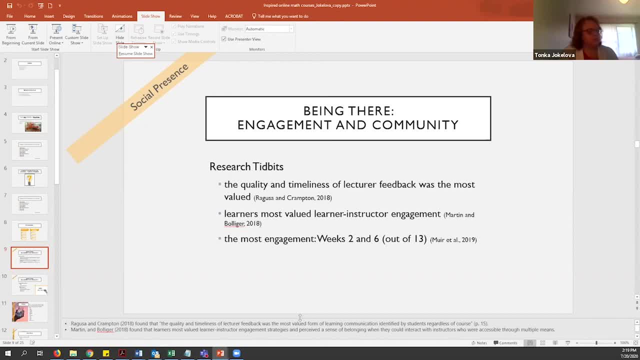 The quote from is a study by Ragusa and McRampton in 2018. and they're saying: they found that the quality and time of study of students is very different than that of students in the classroom. And they're saying they found that the quality and time of study of students is very different than that of students in the classroom. 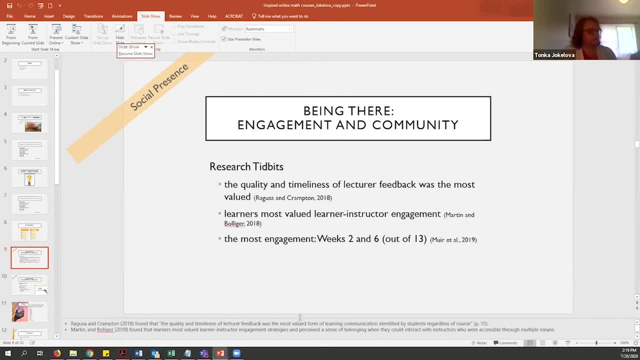 guess of my sugar feedback. This is, I think, Australian journal. so lecture, meaning instructor feedback, was the most valued form of learning communication. I did identify by students, regardless of course. so, again, anworth form of learning communication I did identify by students. 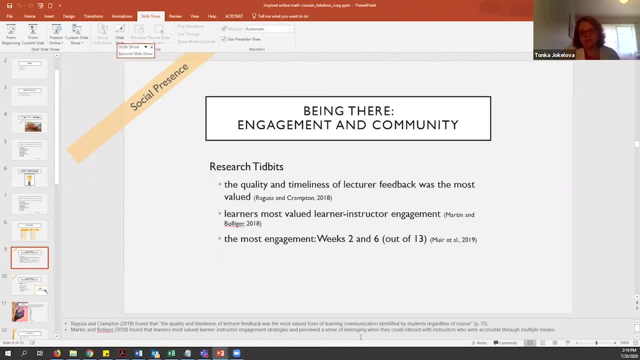 So again, anworth narratives, students. so again, lecturer feedback. instructor feedback is number one valued factor in students learning the course. So again, lecturer feedback. instructor feedback is number one valued factor in students learning. and the second study that supports very similar, has very similar quote or very similar statement is: who has paid it can achieve highgener level, high learning performance. 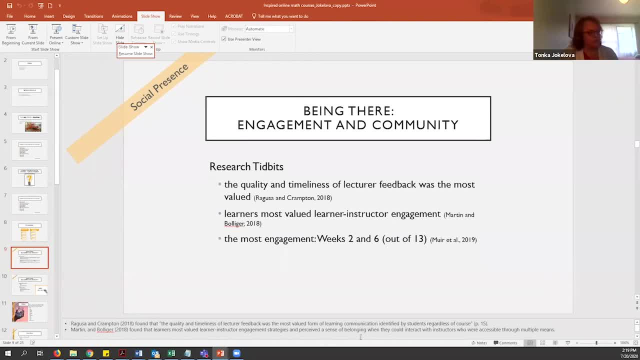 includes with także as being afat patrons. So again is number one valued factor from Martin and Bolliger in 2018, again, and they're saying that learners most valued learner instructor engagement strategies and perceived a sense of belonging when they could interact with instructors. 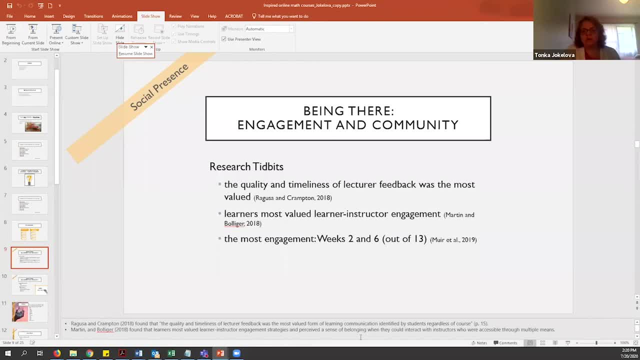 who are accessible through multiple means. So again, your interaction, your relationship with your student is number one thing that will make or break the student's experience In regular online course, in remote course, in coming into the fall and forward. So again, how you perceive your students. 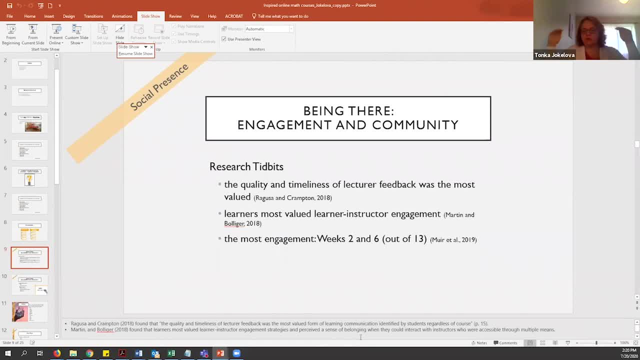 and how you interact with your students need to be very up on your planning list. So you should start thinking about some engagement strategies and how you're going to interact with your students Because, again, just like I said, it might make quite a bit of a difference. 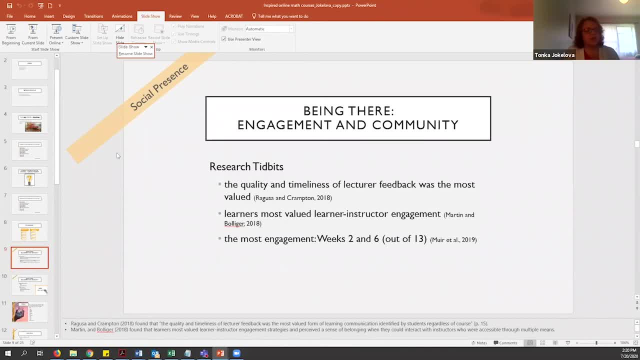 between how your students are perceiving the course And the last bit that I have here which I thought was interesting. but then I asked around and my colleagues kind of confirmed that the most engagement the students are most engaged out of 13 weeks in week two and in week six. 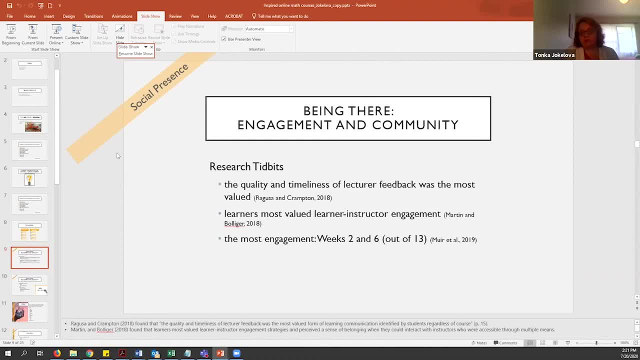 which is really unusual, especially for week two. In my courses my engagement is very high. in week one I do open my courses a week before the semester starts, just for the semester. So if I do have a meeting, I do open it a week before the semester starts. 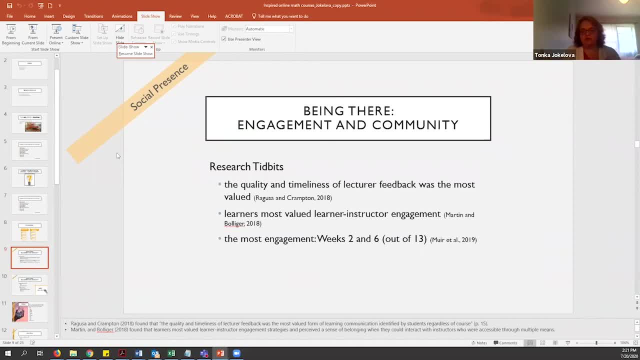 So I have a week to meet with the students and I have to be able to schedule my time and the time for the students to be able to look around and make sure that the scheduling is right and they know when the major assignments are coming, so that they are able to schedule their life. 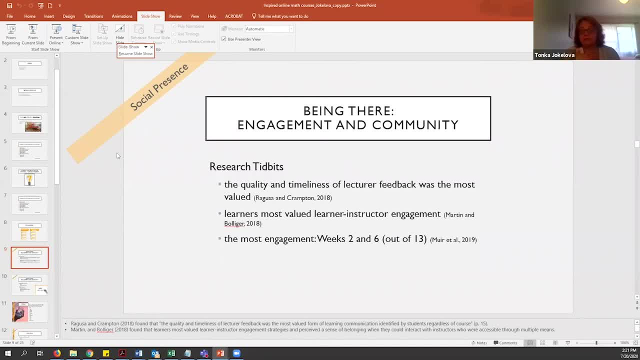 outside of school to be able to meet those deadlines. So I do have a lot of introductory materials- two for sure is more than week one in in their courses, and then, uh, week six, which does not really have to be six. i think what is important here is the mid section, the mid way through the course. 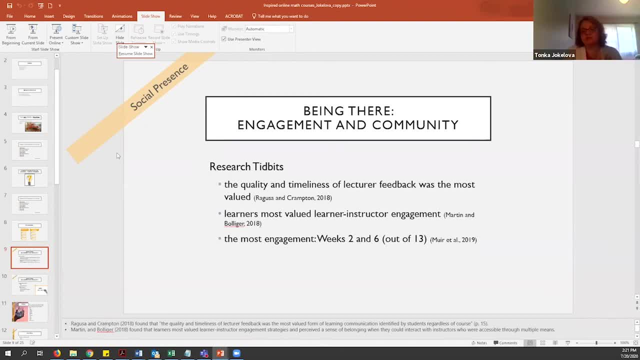 that's where a lot of engagement is, and i'm also assuming it's because there are midterms. i'm also assuming that there is a sort of um sort of urgency to finish strong. so that's why, that's why students come back into into the course and engage more with the, with the course. so i 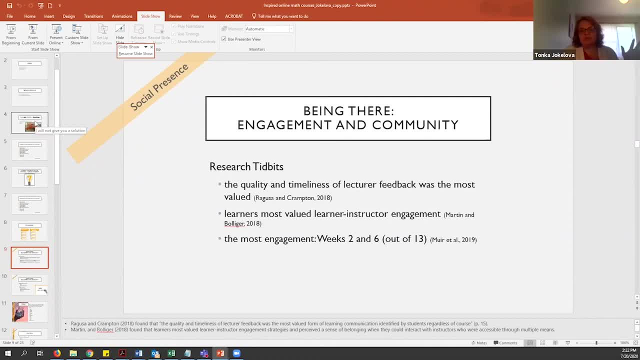 think you'll. you'll find it interesting and just again, summarizing: instructor role is number one role that you can have in an online course and the engagement is kind of at the beginning a lot of it- and towards the middle of the of the course. all right, can i just ask a quick question? is this: 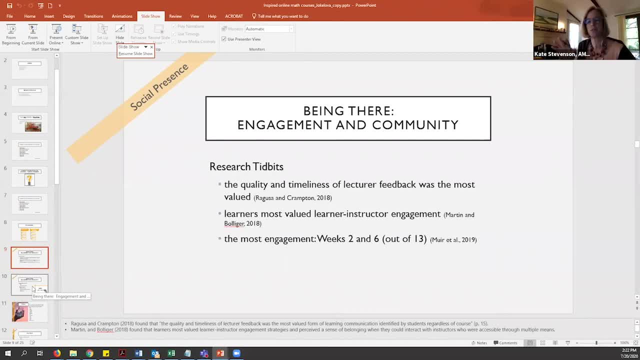 research across all online courses, or was it specific subject areas? do you know it was? i know the one of them was um biology, i want to say, and there were around 1800 participants, i think, in the ragusa and crampton, so, but i'm not sure if it was just biology or it was stem related, or 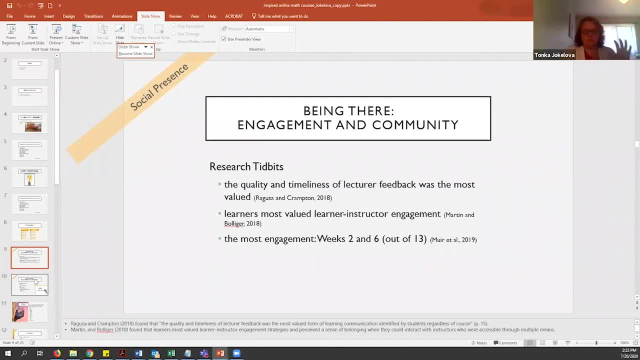 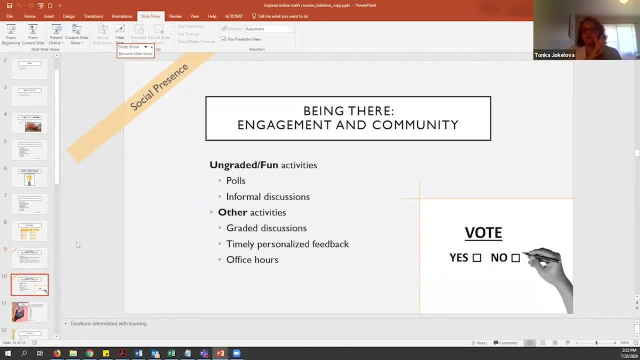 some something tells me it was biology. it's been a while since i read this and i don't remember exactly, but i think it was. it was more on the stem area. all right, let's go into the practical, uh strategies of of what we're talking about. so how do you, how do you, increase the social presence? 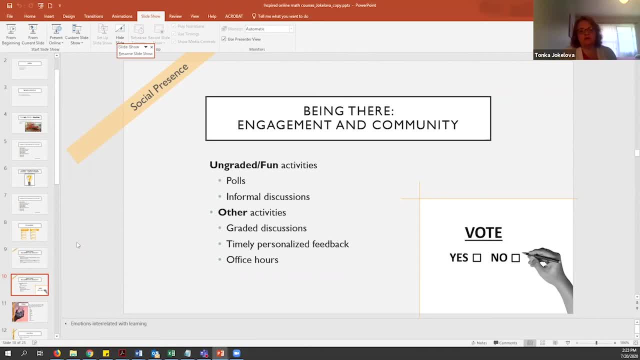 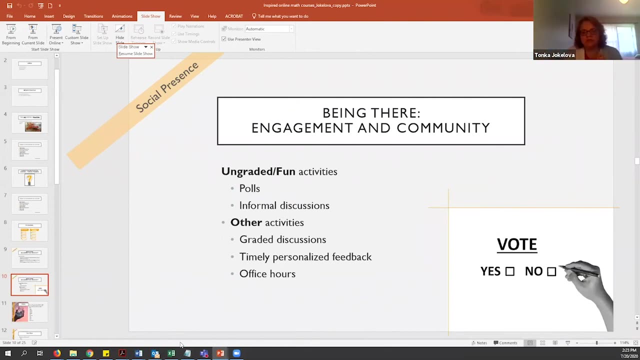 by being there. what i mean by being there is engaging with your students on formal and also informal level. and now, here, it is very important, uh, it is very important. the informalness is very important here because, uh, learning is associated with emotions, or emotions are associated with. 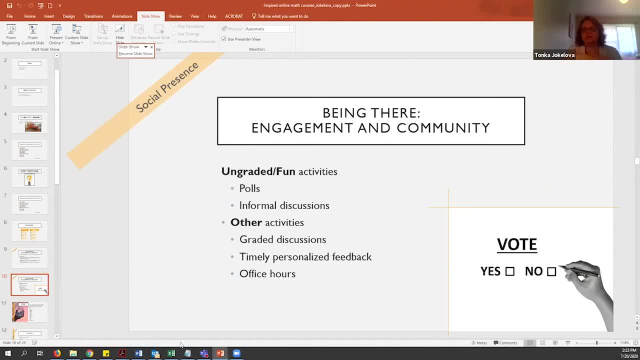 learning. so, if, if i am perceiving something as pleasant and desirable, i will be more engaged in it, and that's what we want. we want to engage students. so, um, you can, um, let's start with the. let's start with the graded or the more formal activities, right? so you have graded discussions that you ask your students. 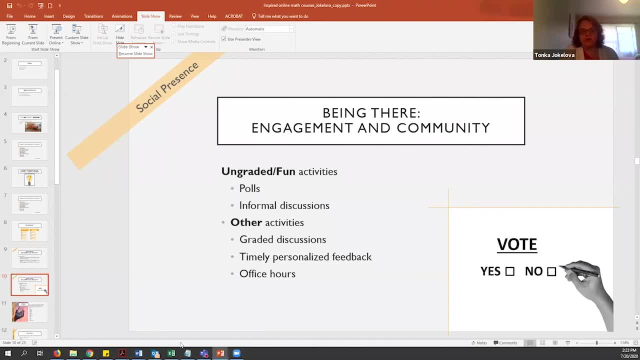 to participate in, and i know you're teaching math and i know you're probably thinking: well, how am i going to have a discussion in the math course? well, just stay tuned in a couple minutes later, where we're going to talk about the discussion, and i know that you're going to have some questions as well, so make sure, if you do have, 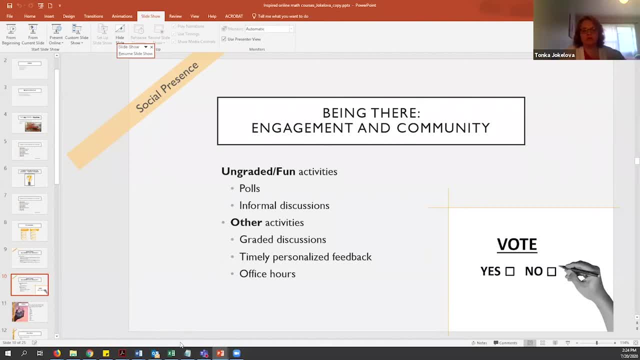 graded discussions, that you are in them, make sure you provide students feedback, make sure you're you're engaged with your students because, remember, number one interaction is the instructor: student interaction. when it comes to engagement, also personalized and timely feedback. many times when we have a lot of students, we just send out one blanket announcement and that is it for our 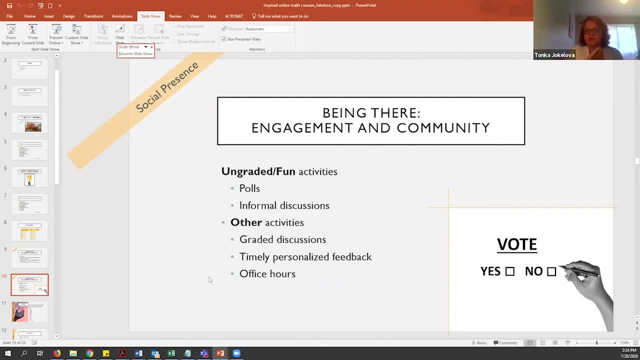 interaction, which, if that is the only thing you have time for because you're doing other things that you need to keep in mind, but think about other ways, how you can personalize that one mass announcement. can you maybe make it into a message? can you maybe say: hey, simone, i see that. 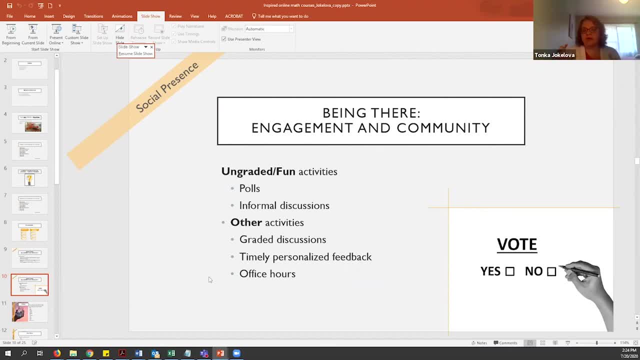 you're something or another and here's the message. you can have the body of the message pre-formatted, you can have it pre-written somewhere and just copy and paste. but everybody wants to see their name, and especially when the instructor knows your name. that's very, that's very, very meaningful and 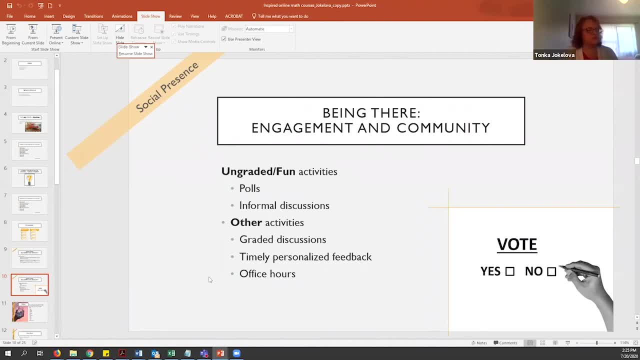 it creates that emotional, emotional connection and closeness between you and the class and the and your student. So if you are able to personalize messages, personalize always address your student by their name, if you are able to. I know the math classes are probably huge and it might take a lot. 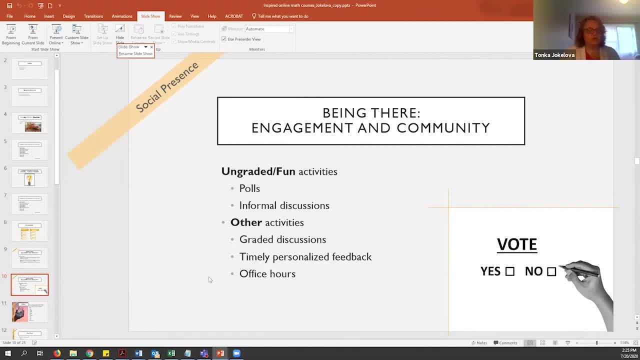 of effort and time to accomplish that. But again, if you're able to, it's very helpful and the student feels that emotional connection to you. And if you're able to- and sometimes it's even required in colleges- have office hours Even if we are all working from home and even if 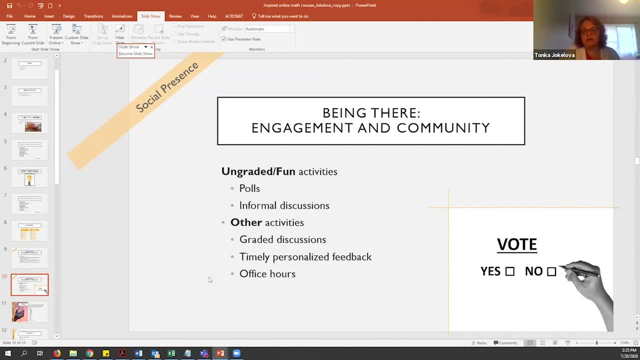 your courses are fully online. you can still have office hours, And you can have office hours, maybe one in the afternoon, one in the evening, one in the morning or however you want to. However, you want to spread it out so that you're trying to make sure that all of your students 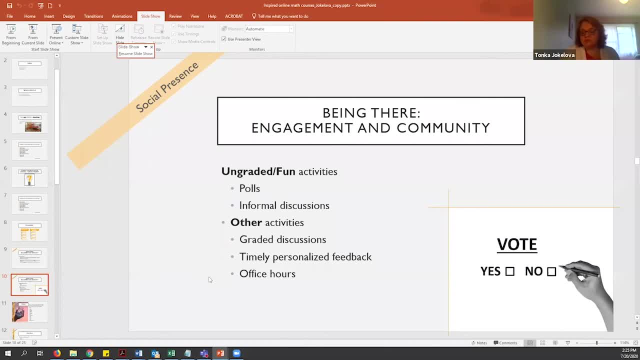 are able to take advantage, Sometimes what you can also do. you can ask: when is the good time to do this, When is the good time to do this, When is the good time to do this, When is the good time for most of you to be available, if you know you are able to do that? 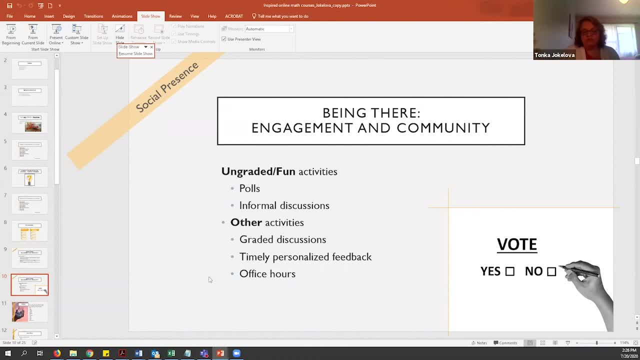 schedule-wise. So ask for, let's say, Monday's afternoon are the times when most of your students are able, if they have questions, to meet with you during the office hours. And again, office hours can be taken any shape, They can be done in Zoom, just like. 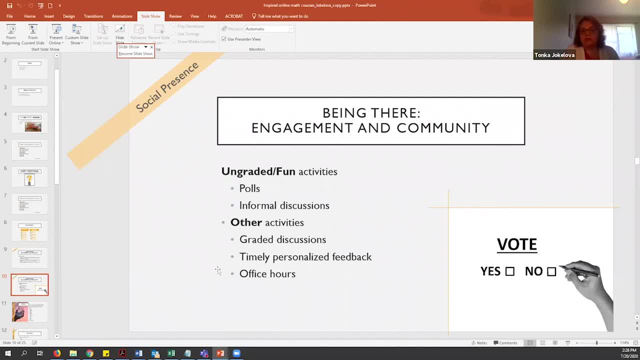 we are right now. They can also be in chat. They can be in email. Just say: okay, on Tuesday, between three and four, I am on email and I am waiting for your questions. So the student knows the second you get an email you're working on it, right? Because that's what you said you were. 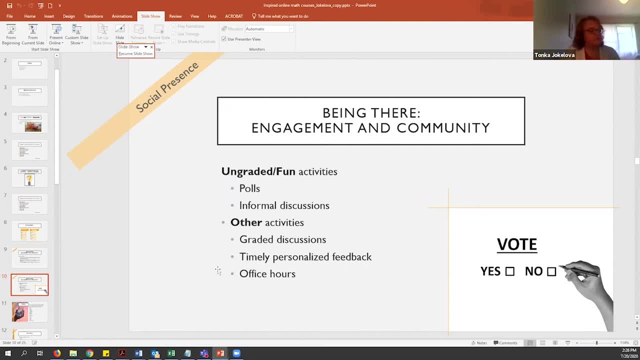 going to do So again. office hours can take different shapes and forms. You figure out as you go what is the best shape and form for you and your students. But having those even in online class is very beneficial for your students. And now let's go. 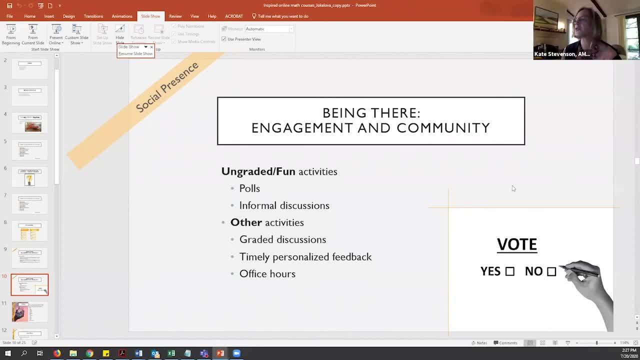 Pedro Morales is asking: what do you think about social media for social engagement? Is it advised, Is it dangerous? I do not do social media, but that is my personal choice and I don't. And if you are a social media type of person, I would, Of course I would. However, I would definitely be mindful. 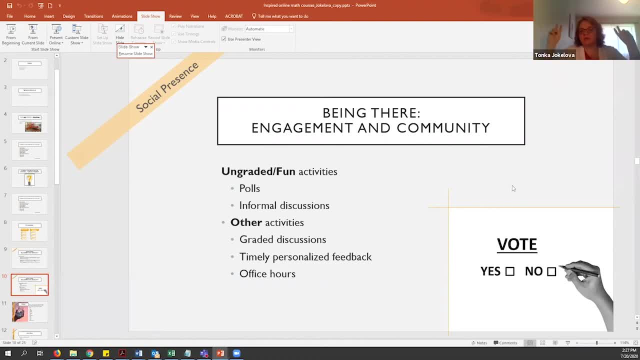 about the level of personal is shared in the social media. I would definitely make that. make those guidelines very visible to your students. If we are going to use social media, if we're going to create a social media group somewhere in one of the platforms, make sure that. 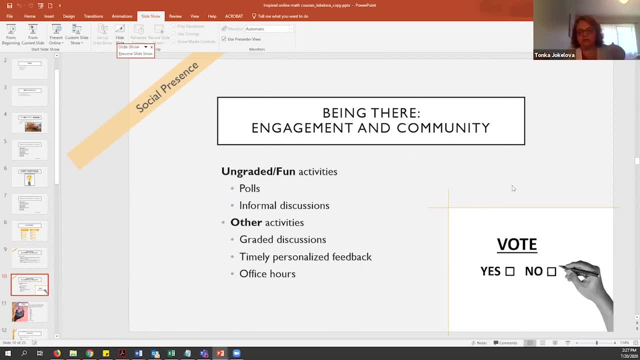 it is. if it's not academic, make sure that it's. the netiquette rules apply. no matter where you are, as long as you're with your, with other students, with your fellow students, you always have to be courteous. You always have to be polite. There is no disrespect that will be tolerated. There's. 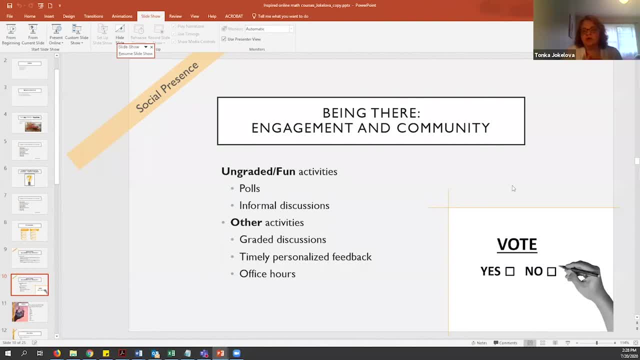 no disrespect, that will not be tolerated, So I don't use it. But if you, if you are a social media type of person with guidelines, I do recommend because it does engage students and students live on social students, live on social media- a lot of them these days. So that's. 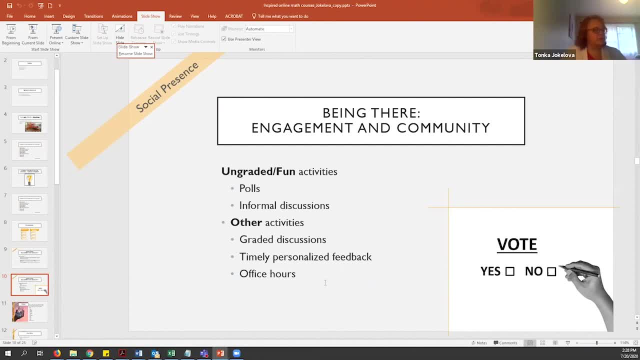 definitely a good way to to engage your students, Absolutely. I've heard some faculty that use it quite a bit. They welcome students to text them if they have questions, For many students helps them. I just think you have to be aware that, as surprising as this may be, 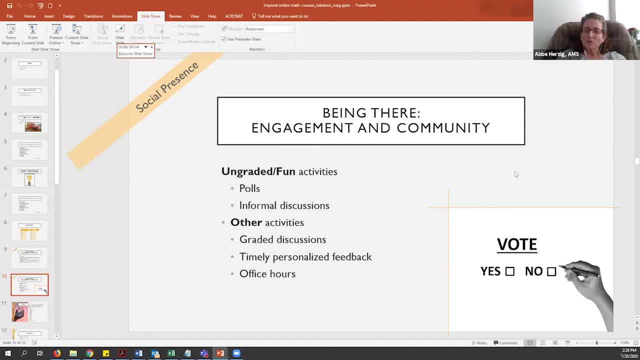 there might be some students who are not on social media or who don't have easy access to the technology. So Absolutely Can be required mode Right, Exactly, I always get somewhat mad when there's a voting over kind and you have to use. 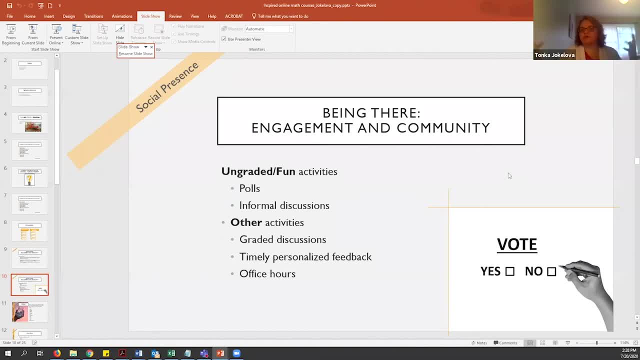 Facebook, but guess what? I'm not on Facebook, so I cannot vote on whatever concept it is right. So you always have to be mindful of what kind of students you're having You're looking for. your students might not be able to to be, to be using whatever it is you're using. So all those things for sure. 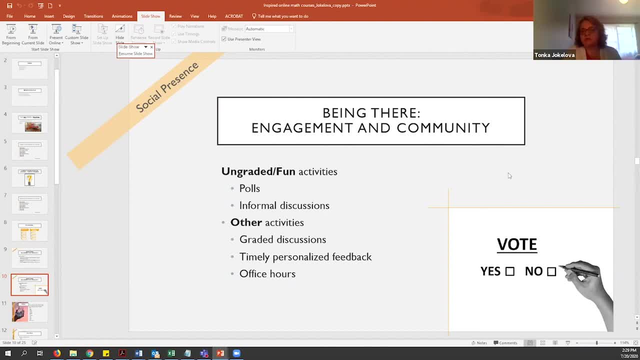 Have to be have to be by choice. And also, if you are providing your students with your cell phone, Make sure you have guidelines, Make sure you tell students you can text me. however, not after eight o'clock and before eight o'clock in the morning, right, because students live on different, different timezone. 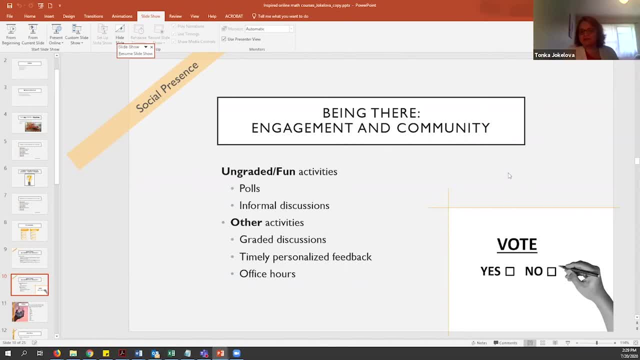 Many times and I think that's kind of a good opportunity. Yeah, Yeah, Yeah, you will get text three o'clock in the morning before the assignment is due, and it's just. you know, that's not where you want to live. usually i am my. i teach fully online course. 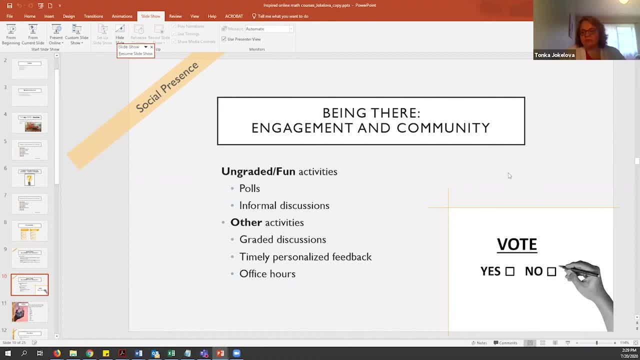 and i- i tell students- i'm going to respond to your email within 24 hours and i'm going to, i'm going to grade your assignments within a week. so i know this is an online course. however, i do not live on the internet. i have life outside of the internet, so don't expect me to respond to you within. 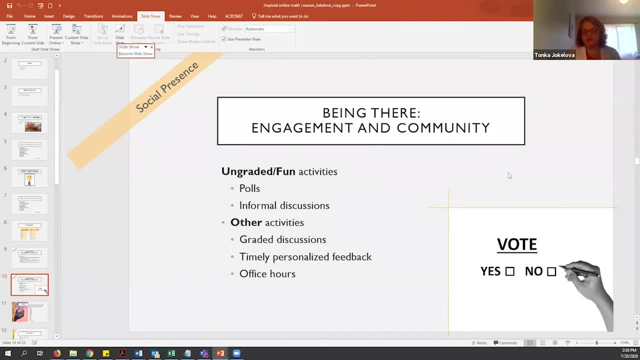 five minutes because it might not happen. it might, but it might not. so i always give myself this 24 hours. you can do 48. i think that's that's acceptable as well. just give them guidelines so that you are not just bombarded with um with stuff on your social media and you know your phone for. 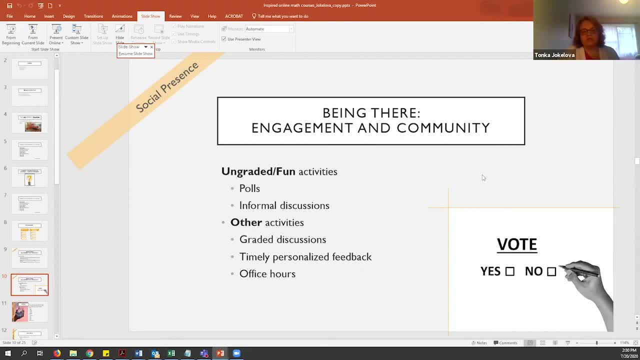 sure, all right, let's go to ungraded activities. and those are very important because when you come to class in person class before the class begins, you talk about anything. you talk about, oh, my goodness, that meal that i created yesterday for dinner. it was out of this world, or? or i went to whatever festival. 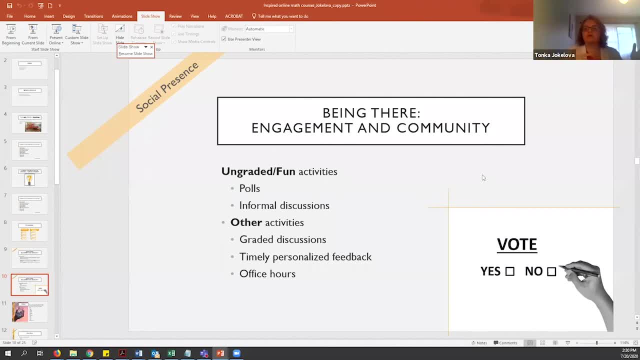 and whatever happened, and i saw whoever right. so they talk about all those outside of subject um topics and in online course. if you don't have that, it might feel very isolating. you might feel like, okay, i'm here for the math, i'm gonna do my hours of math and that's it and that's not what. 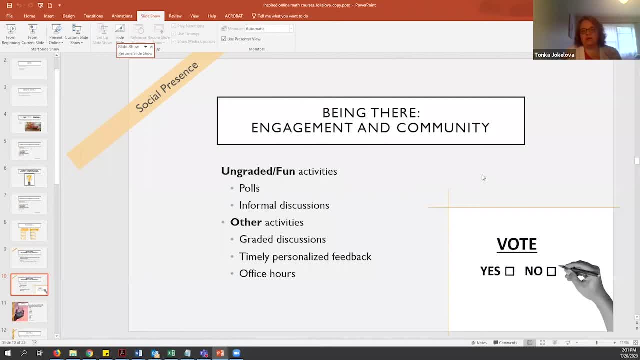 you. that's not only thing. you want them to be, uh, when they are in the course, they also want one them. you also want them to be students. you also want them to be social beings and if you give them that, that space in your course to discuss informal things, they will come into. 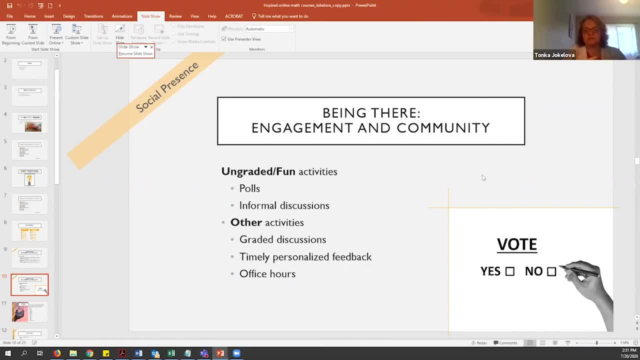 the course. they will engage with the course because they are looking forward to speaking to their buddies from the course right, and once they are in the course, they will look at your discussion, they will look at your uh assignment or they will look at the syllabus and see what's. 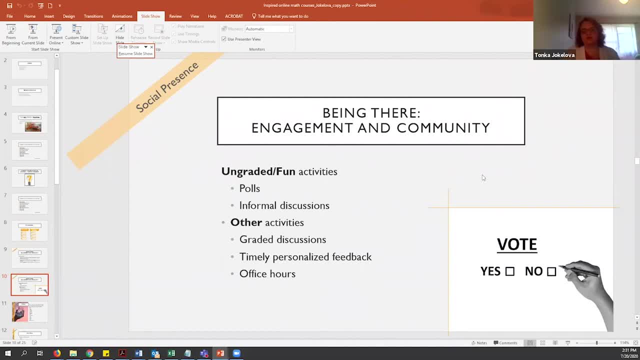 going on on course schedule right. so once they're in the course, they will stay in the course and- And I actually give you the next slide- I will give you some my observation from my own course and some percentages that I think you will like. 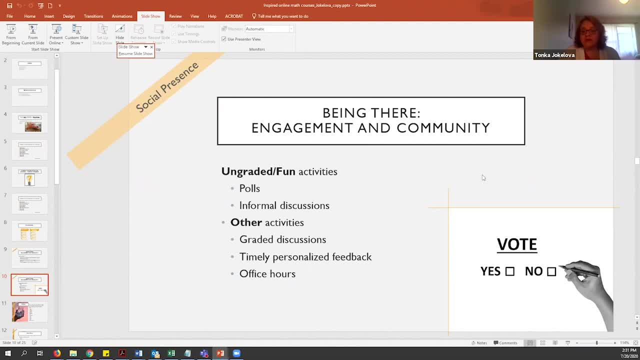 So you can create polls, just like the poll that we had before we started. We had a poll about how you're feeling right now, basically what it is that you need, And you can use that in your courses, and the poll takes maybe five minutes to create. 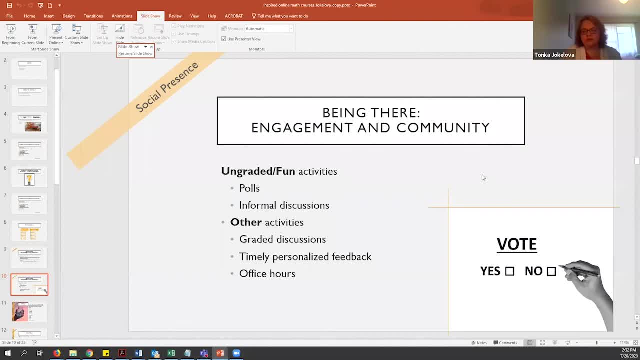 I know some LMSs have a poll tool, some LMSs don't. But if you don't have that tool in your learning management system, you can use SurveyMonkey, just like I used for this presentation. It's free and it's very easy to create and give the surveys out to your students. 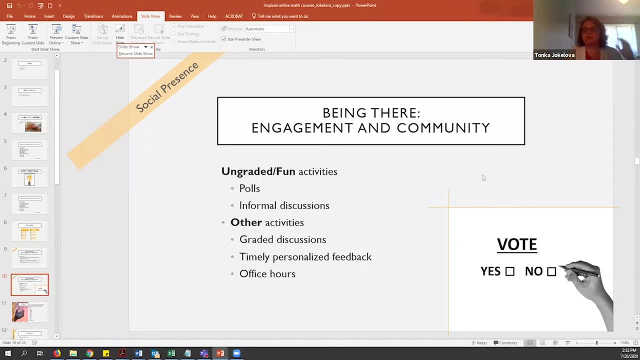 What is important in surveys and in polls is, just like you were able to see where you are at the end of the survey after you submitted survey, you will see, oh, six other people also need patience right now. And oh, three other people also need. 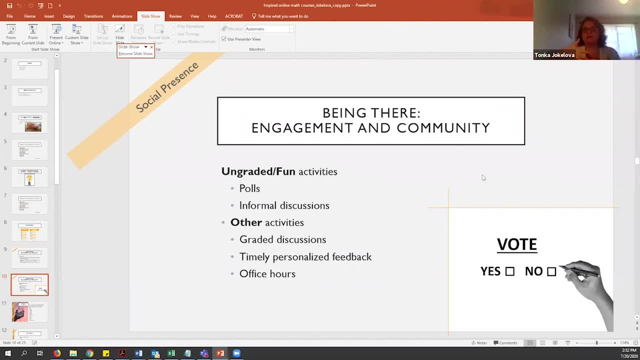 So that is, the ability to see the results at the end of the survey- is very strong, because that is what is connecting students to other students. That is what makes it feel like I'm not here alone, lost in the cyberspace. Other people have the same issues as I have right. 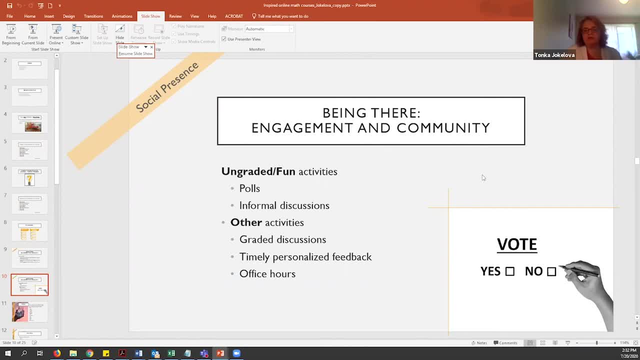 So we found out that a lot of us need patience And we can kind of pontificate on why that is, And we probably know why that is And that is because we're coming into uncertain times. So you, as an instructor, if you're seeing that there is a trend in one of the things that students need, 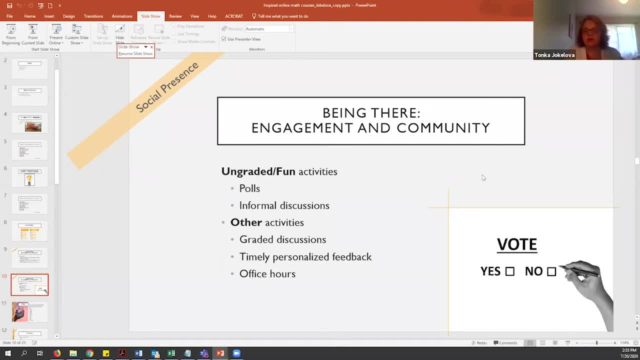 you can address that in an announcement. You can say: oh, I see a lot of you need patience right about this time, And I'm feeling with you here because, yes, I also don't know where I'm going when it comes to the teaching. 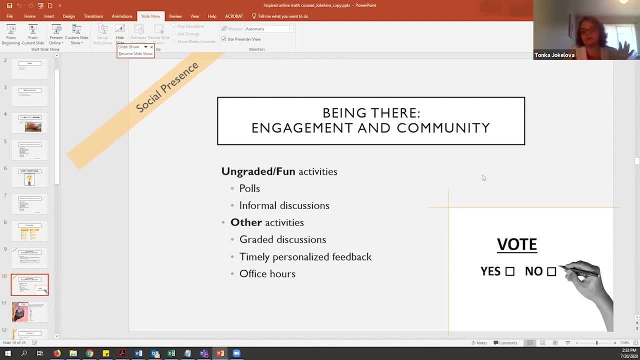 So we're in it together And here we go again. You're creating emotional connection with your students. They're emotionally connected to the rest of the class because they're seeing comparing to comparing themselves to others when it comes to the results of the poll. 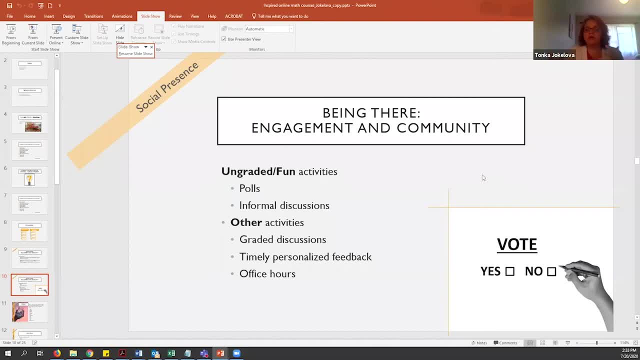 And you're also addressing it And you also let them know that, oh yeah, she cares, She knows, She's seeing that we are struggling, She's seeing that we need strength. So you are creating this impression of a caring, caring person. 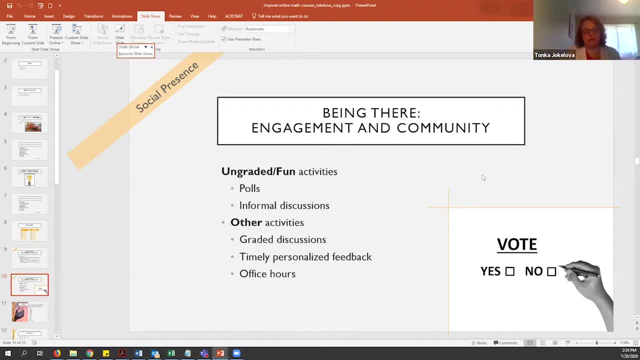 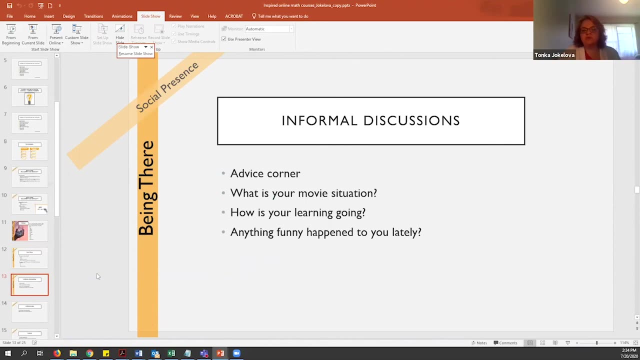 And we'll talk about it a little bit more as well in the caring, caring, caring- portion, Informal discussions: Again, we already talked about some of the informal discussions. I'm going to skip one slide. Some of the informal- oops sorry, some of the informal discussions you can use is advice core. 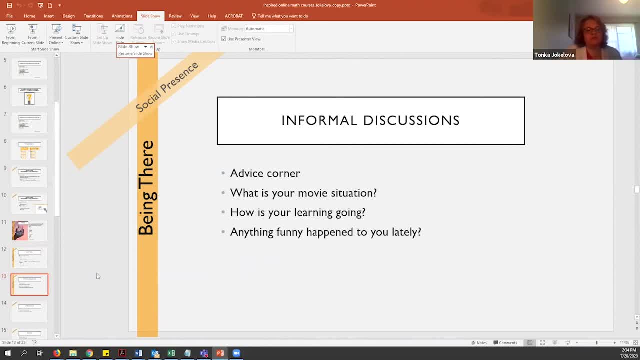 If you have an online course, let's say a fully online course, somewhere along the beginning of the semester you can say: hey, if you are new to this online thing, ask others what you want to know And if you are already seeing it. 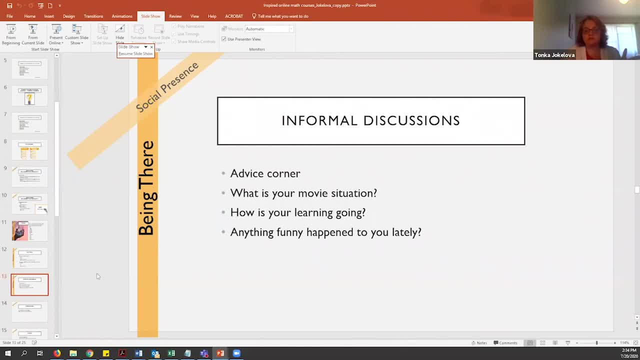 I'm going to skip one slide. seasoned online course taker, you can provide advice to your classmates. you can say um, what helped you in your first semester taking classes online. so we always have some mixture of of experience and inexperienced students and we can- we can provide emotional kind of advice to 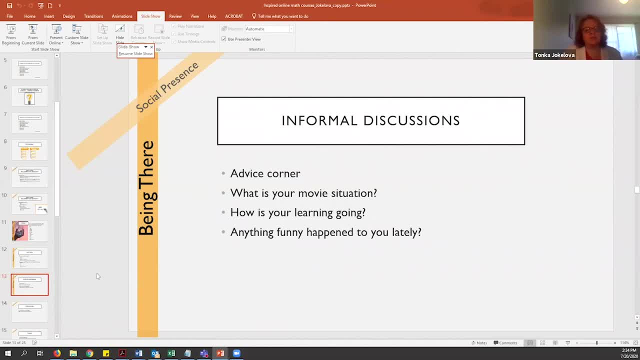 each other, not really emotional only, but it can be also time management: how to make sure that your- uh, your assignments are on time. is there any time management tip you want to share? you can share, and the students you would be. you would be surprised the students actually do share a lot. 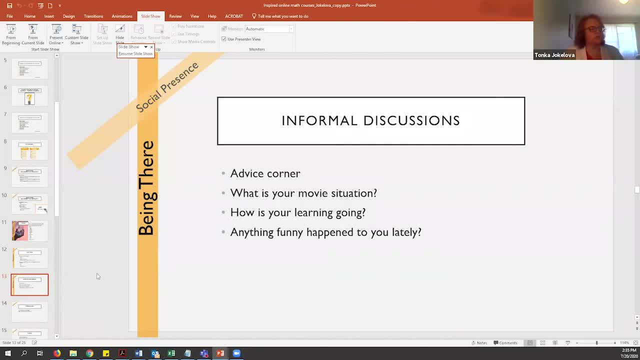 um, especially when somebody has a question, there is a lot of students who answer that question. some other things, um, completely unrelated to course, because again, uh, you are trying to mimic that before the before the class starts time, when students talk about anything under the sun, or after the class, everybody goes to have ice cream to this ice cream shop. next, next order. 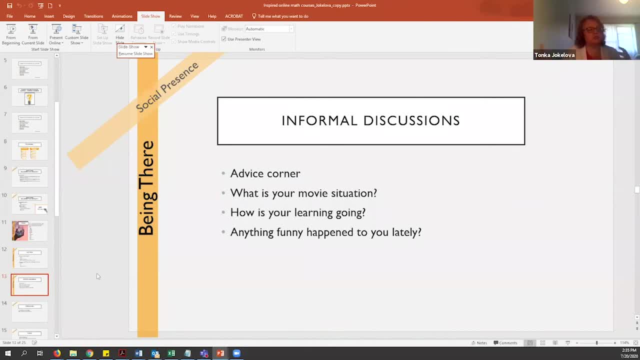 to the college, right? so you're trying to mimic those situations. so, having something related to the subject matter of your of your course is okay, but it's not as great as if it's completely nothing related to your subject. so how is your movie situation? well, obviously, we're not watching. uh, we're not going to movies, right? 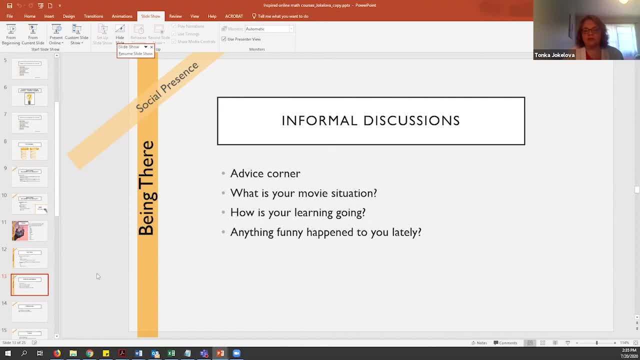 now. but have you read any book? uh, interest, any interesting book lately that you would like to share, something that will be completely um, out of the subject, but social, where students can engage in the course, they don't even have to add an instructor, or a teacher can pipe in. 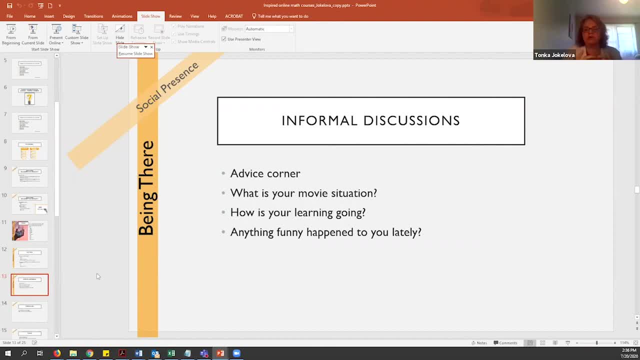 don't have to just give them the opportunity to socialize. and once they're engaged, when they have buddies in the course, they're more likely to stay in the course. when the getting, when the getting gets, when the going gets hard, there we go. so they're more likely to persevere if there is 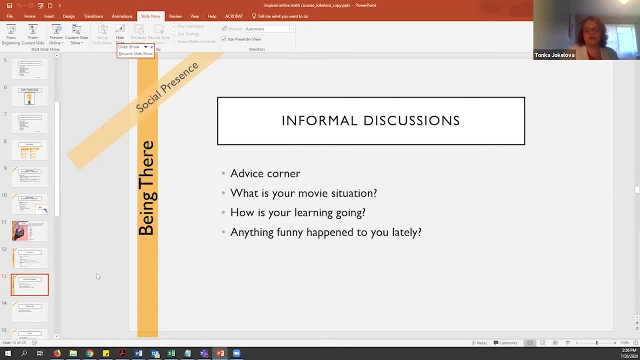 this assignment that they just don't know how to, because they have. they have network of buddies in the course already and you, you kind of establish be um the basis of that. so um are great, are great to have. Let's go to the poll, The poll I was telling you about and the 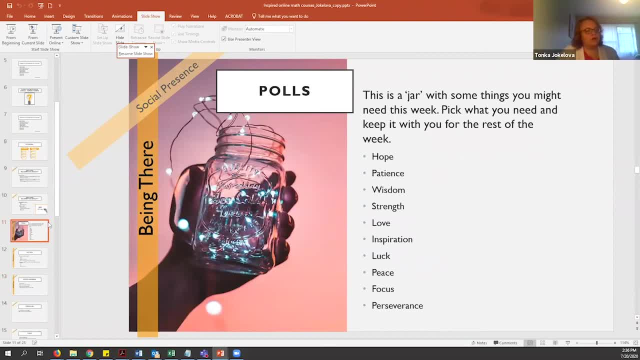 poll that you took at the beginning of the webinar. I have in my course and I have it in every week. So my modules are one week long and in every module I have this poll and I'm starting the poll fresh every week. So I'm clearing all the answers and every week we're starting fresh. 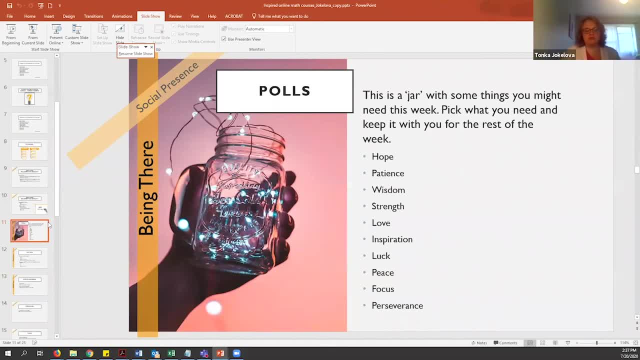 because every week we might need different things, right? So I want to make sure that they have that ability to choose different things And I looked at my courses with this particular poll and without the poll and the discussions that were graded In the courses. 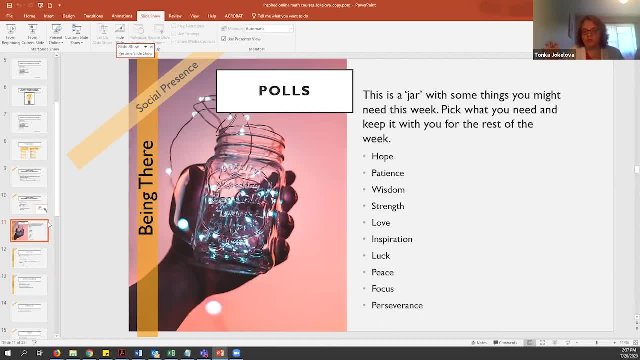 with the poll. I had 20% more participation in the graded discussions- not in this one, but in the poll, in the graded discussion, and this is where it matters right. this is where the students are getting their grades from. they're getting from being graded. 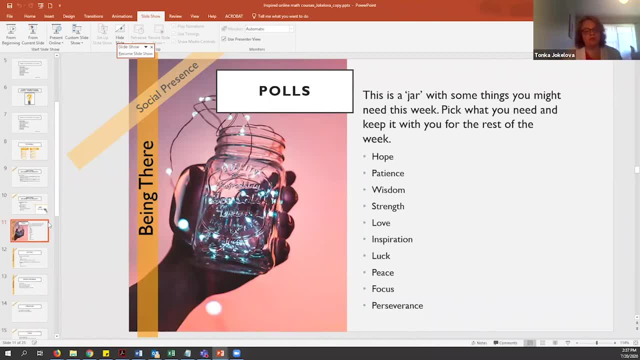 discussions. so what happened here? I'm assuming what happened here? every week the students come into the course and they will pick whatever it is that they need from their jar and while they in the course they look around and they participate in the discussion. and oh, Suzanne posted this. let me see what she 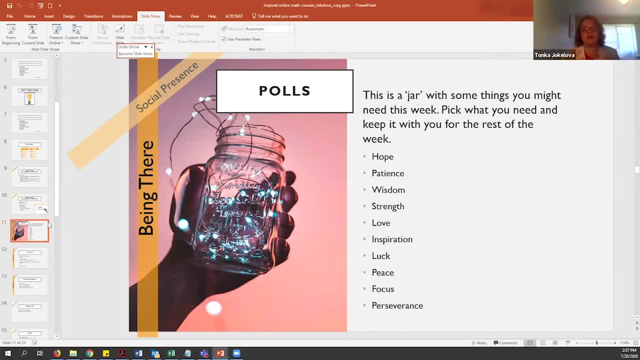 posted and now I'm posting to to answer to Suzanne. so I am as a student, I'm engaged with the course, with the materials, but I'm also engaged with your, with my instructor, because my instructor wants to know how I'm feeling emotionally. and I'm also engaged with other students because I'm already 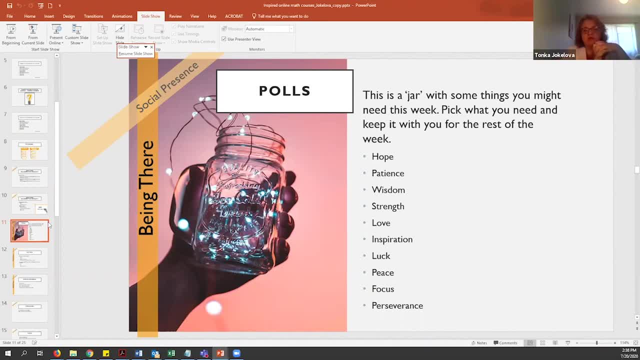 discussing with other students in the course. so there is a very good attention-getter. and one other attention-getter that I found is posting funny pictures at the beginning of the course. now, they don't have to be funny, funny, but they're just gonna be, you know, somewhat interesting and the 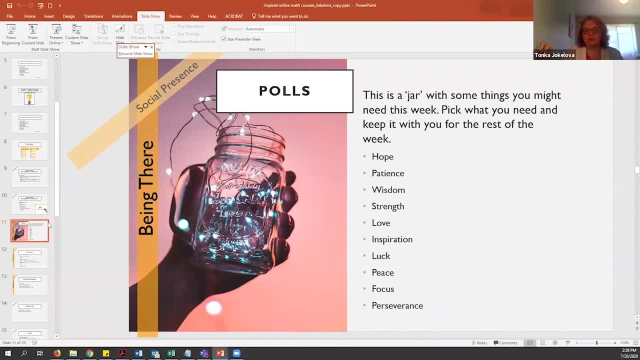 strategy here that I have is I only posted Monday morning, so it's not there until Monday morning. on Monday morning I post the picture and, what is funny, I actually had feedback from some of the students saying I cannot wait from Monday morning to see what kind of crazy picture he posts this week. and this is: 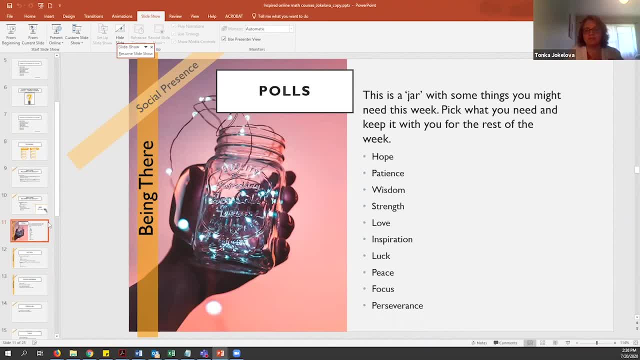 what I'm trying to get. I'm trying to get information from my students so that's get them into the course, and I'm trying, once they're in the course, trying to engage with others, right. so Monday morning they know that some crazy picture is going to show up in their course. they come into the course and 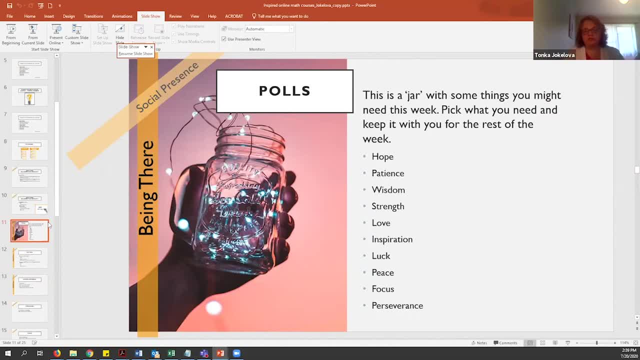 they stay and they look around. just like I said, with this poll, this particular poll, I saw 20% higher engagement in graded discussions than in a course without this poll. and, what is also funny, I asked my students to comment on anything in the course, at the end of the course and if there was ever any, 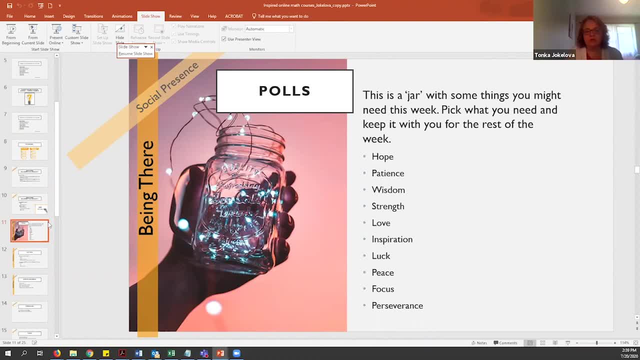 comment on a course activity. it is a comment on this particular poll. I mean, as innocent as it looks, people love it. it sounds cheesy. and what do you want to keep? you want to keep hope, you want to keep patience. it's so cheesy if you want to look at it that way, but it gets students engaged and it gets students to. 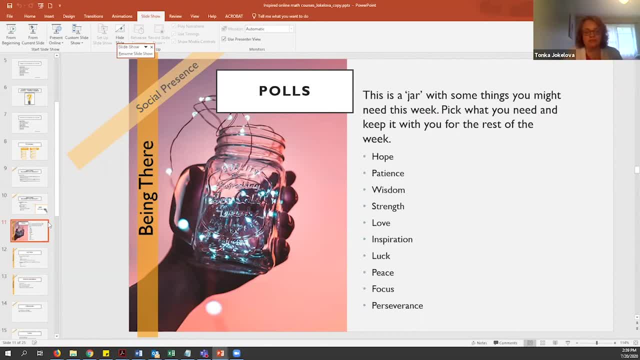 feel that they are supported by, by the community, and that's what. that's definitely what you want. I got the idea from a, from a pastor, I don't know what college and I don't know anything else about this- this, this pastor, and just know that during the midterms he posted an ad, remember, like: 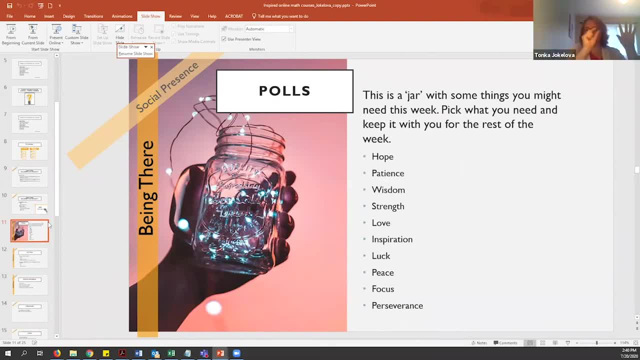 old-fashioned ads. if somebody's selling in a car, they have little strips cut out at the bottom of the paper and everybody with the phone number, and everybody will just just tear off that one little strip and take him with them so that they have the phone number. so he got the idea and that's what he did. he. 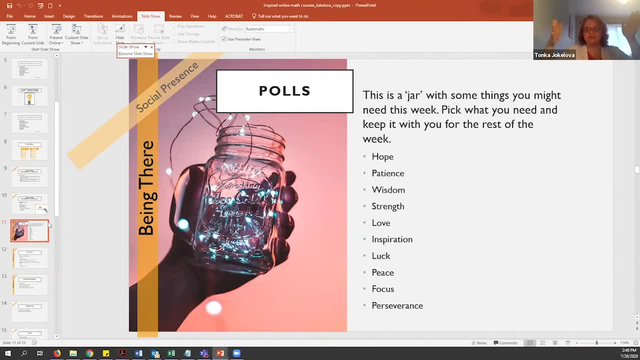 posted, posted those ads like: hey, take what you need. this I know it's going is getting hard here because we're in the midterm and you have to study, so take what you want. and I saw it I was like there is no way I cannot duplicate that. 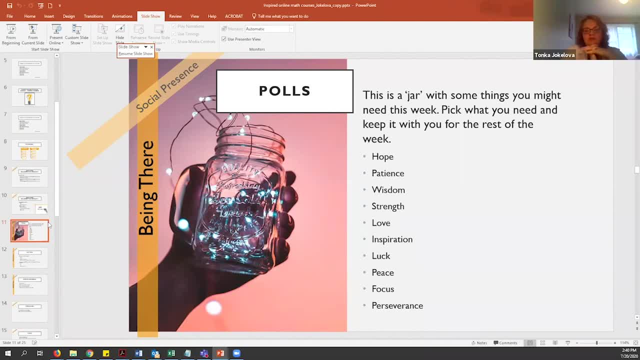 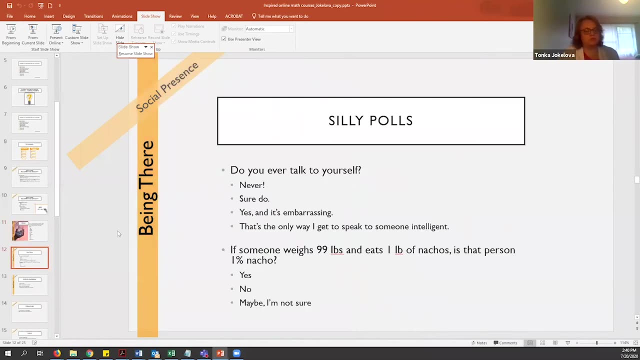 in an online course. so I did- and this is one of my favorite activities of my course- because it's just so, so easy to create, yet it has such a has such a humongous, humongous impact on your students. now, some other polls that you might also want to use are some silly polls, for example. I love 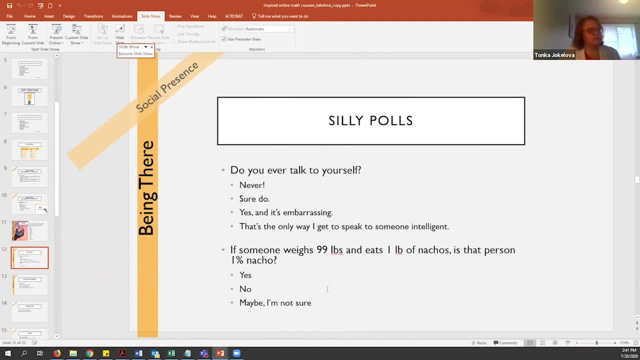 this one, and I think you like that too as mathematicians: if someone weighs 99 pounds and eats one pound of nachos, is that person one percent nacho. so just silly polls, something to engage them, something to get them into the course, something just to brighten them that they their day for a minute. so 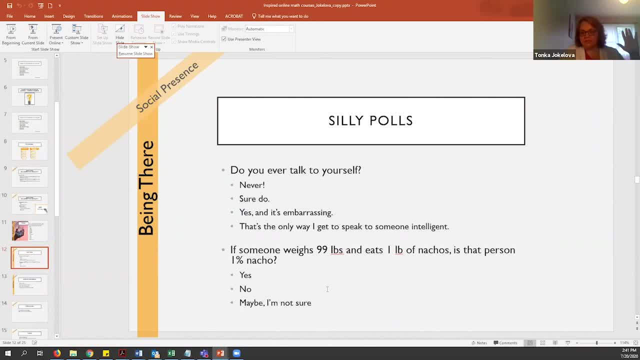 something silly. those work as well. they do not work as well as the one the jar. I did get good results, but not not the 20% range that I had that I had in the jar the jar activity. so emotional connection is definitely what students crave when 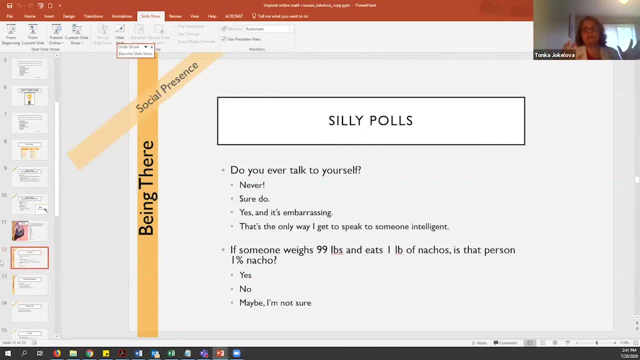 they are in online course because it's such a such easy thing to just let them be on their own in online. it's just not what they want, though. all right, do we have any questions? did I need to stop for? no, okay, all right, so let's move on. we already talked about 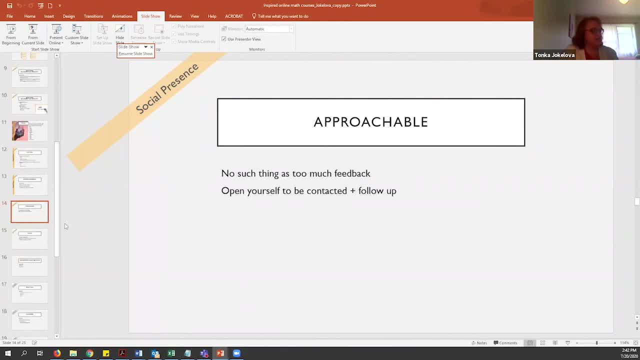 the formal discussion. the second, second topic in the social presence, in the social presence column that we know we saw, was make yourself be approachable. but not only be approachable, but also show them that you are approachable so that it's easy for them to ask questions, is easy for them to be engaged with you. 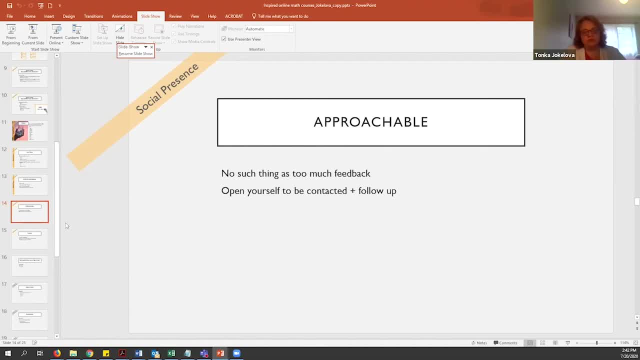 it's easy to touch when they are approaching them. they can simply put something just at their desk over the desk when they want to useよ. please come to my office hours or please let me know and we'll schedule a live session on the topic, something that will open you up to to being contacted many times. students, especially in large. 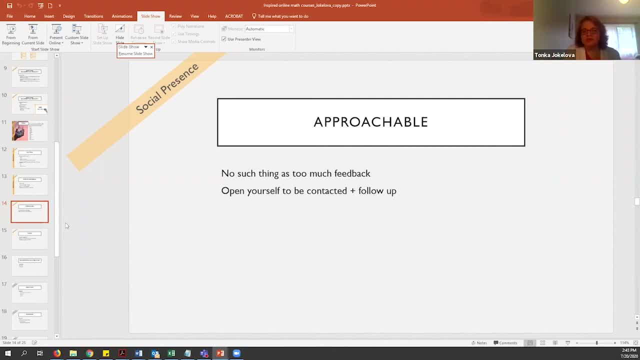 classes are not comfortable contacting their instructor because they feel like instructor is somebody very foreign, somebody who is very on the other spectrum of things and I'm just not comfortable talking to that kind of person. but if you open yourself up to to being contacted, if you open yourself up to to making sure that you are giving the student the right explanation of, 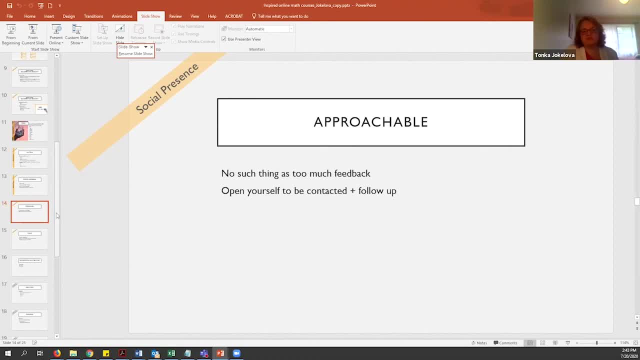 things. they will. many times they will take you up on it. so make yourself approachable and also show them that you are approachable and caring as well, which is our last, last portion. so some of the caring, the message of caring, was in that, in that poll that I showed you when I when I said that after you see some trends in the poll, in 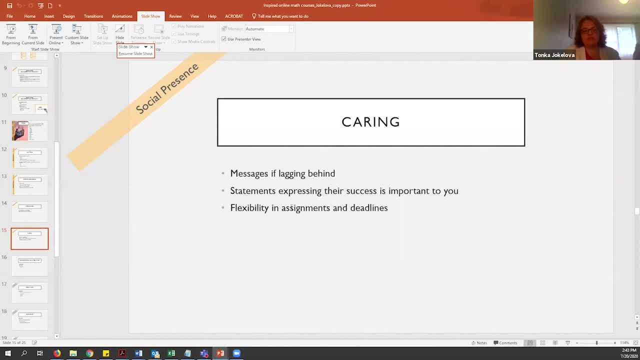 the jar. only when you see some trends, you can address them in an announcement and then you will perceive them as a caring. caring instructor came first because you're seeing that all of the students- a majority of the students- need strength right now, so you care how they feel. also, if you 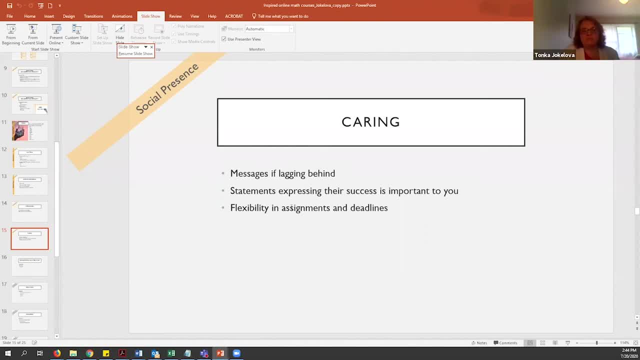 are seeing that somebody's lagging behind. message them if you are seeing that somebody was doing a lot of work and they're not doing a lot of work and they're not doing a lot of work and they're not doing. wonderfully in the first part of the semester and they were getting all A's and they were. 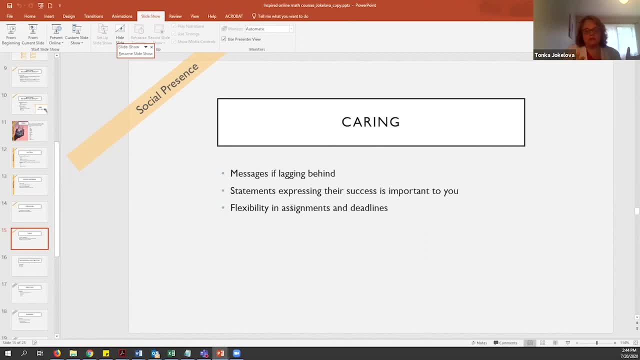 getting getting the content and you felt confident that they understood and suddenly they're not doing. they're great. show them a message like: hey, I'm noticing a change here in your, in you. is there anything I can help you with? is there anything you need? you need maybe tutoring on or something. 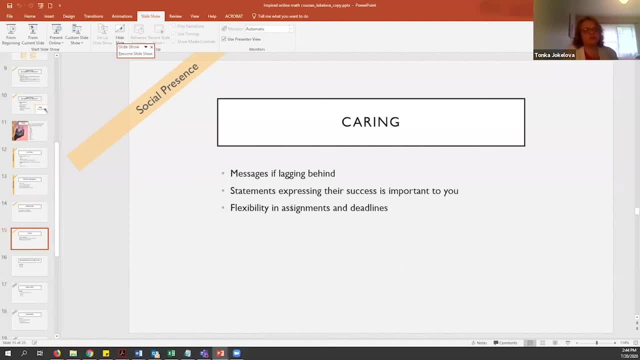 like that right. so always make sure you message if you're seeing somebody, somebody's performance change and if somebody is not engaged in the course, because, again, the instructor of student relationship is the most important relationship in an online course or course with online components. we have a question from Moira McDermott. she says I believe that there 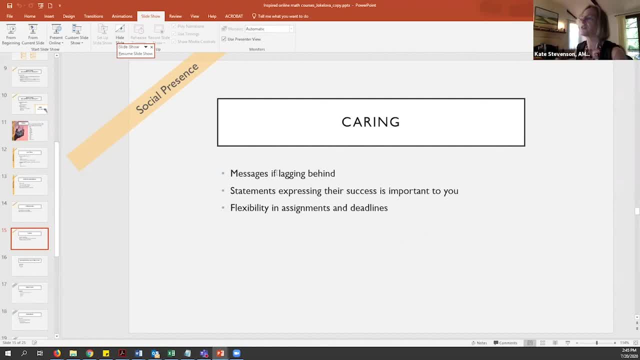 is research about how students expect certain things from women faculty more, including caring. how do we navigate through the online environment? and how do we navigate through the online environment, those expectations- Wow, that is so interesting but so making sense. absolutely I didn't think about that, but, yeah, I will have to look into that. so I think how you would navigate it there. 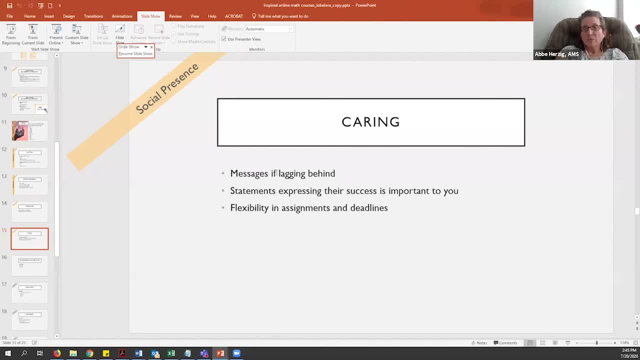 is a research that this happens quite a bit in face-to-face interactions. there is a research that this happens quite a bit in face-to-face interactions. there is a research that this happens quite a bit in face-to-face interactions and that women faculty sometimes end up getting overloaded by all the students coming to their 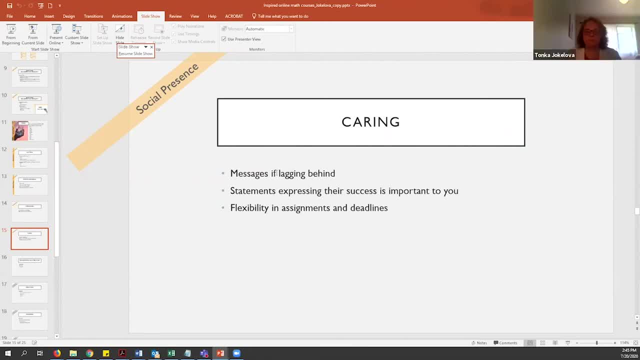 office for advising and for other things, because they've just greater caring. I wonder if that's an issue online because they, the way they have access to you, is different. that's, it's a very interesting question. you know what's funny? um, before I have a video in my course and um, but it's. 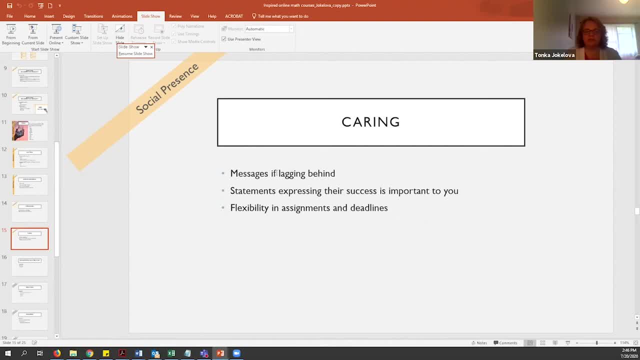 interesting. you know what's funny? um, before I have a video in my course and um, but it's interesting. you know what's funny? um, before I have a video in my course and um, but it's it's kind of late that I added it and before I didn't have a video in my course and some students told me towards towards the middle, towards the end of the course, they thought I was a man because of my name, because my name is so unusual. so you can just kind of kind of pick gender because you know my name is not really a female or male, I guess. and I do get a lot, of, a lot of messages, but I don't think I can be very. 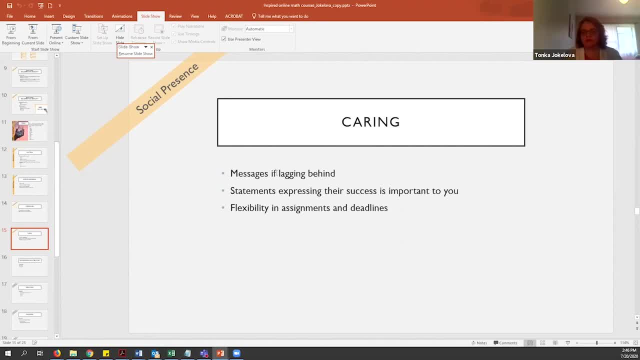 I do get a lot of a lot of messages, but I don't think I I can be very um meaningful and research-based on this topic because I have no research in it. so unfortunately I don't have answer. but I think if you, if you have guidelines, uh, what you are really? 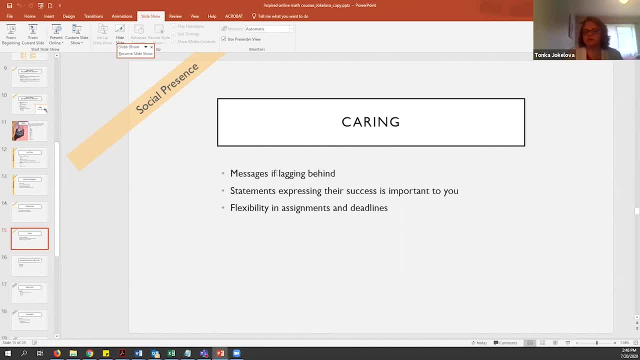 you are not willing to do. maybe that will help and just post those um in the course beforehand. you know the extents to to what you're you're okay going and to where it's just going to be. uh, maybe we will need to talk to somebody else and just spread the wealth. i'm not sure, i'm not. 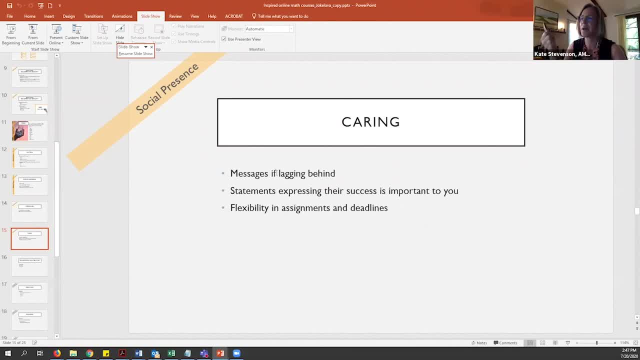 sure that is the- i think that seems to that sort of matches what moira is uh following up with. she says that also evaluations depend on how far you are from their expectations. so what i'm hearing you advise- and i i think i agree with it- is that it may be even more important for women to set 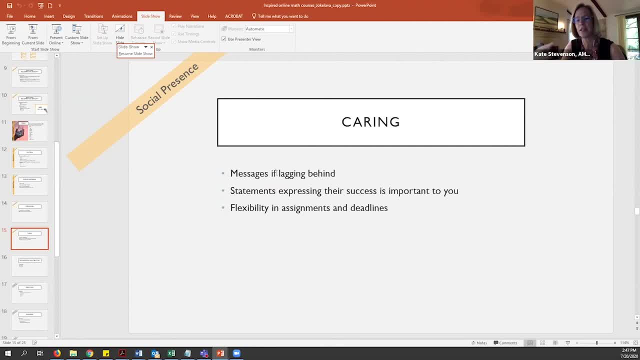 those expectations at the beginning of the class, so sort of be very clear about how available you are, how much you do care, and then also some boundaries around that, so that you're meeting an expectation that you get to define, uh, in the beginning of the semester and it's probably good. 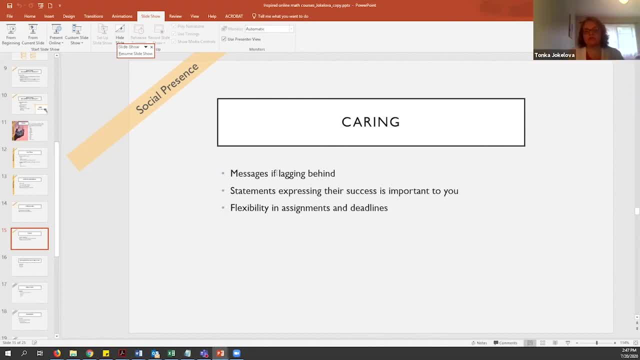 advice for anyone, right, sometimes what i do do, um, when i get a lot of especially uh from international students- and i wonder why that is especially from international students- i get millions messages at the beginning of the course about everything under the sun and, um, i try, i try to always try to respond as quickly as i. 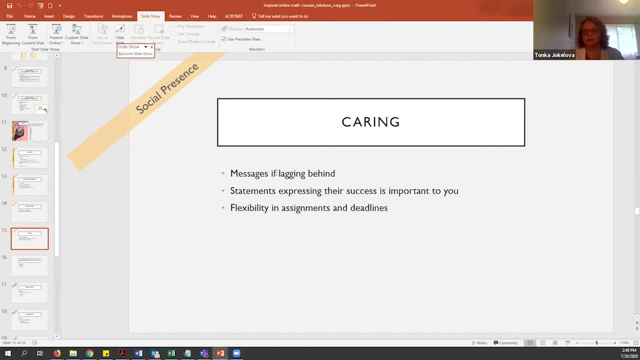 can. but then, when the messages started to be overbearing and it was just nothing but messaging with this one person, i- i got to the point where i said: okay, so okay, here's what we're going to do going forward. you aren't going to first read the syllabus. 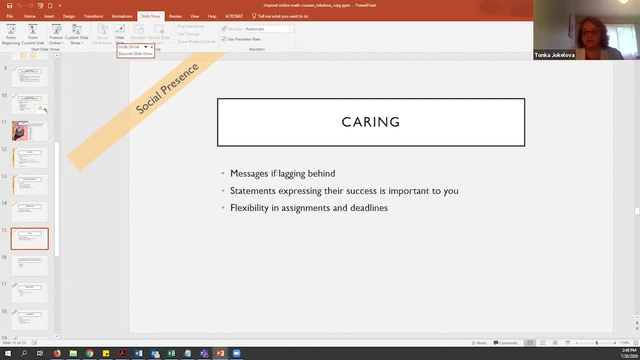 and if this, the question that you have, is not answered in the syllabus, then how about you wait half the day and then compile several questions and then shoot me an email, because unfortunately i have 24 other students and i'm not able to only respond to a million of your messages and nothing. 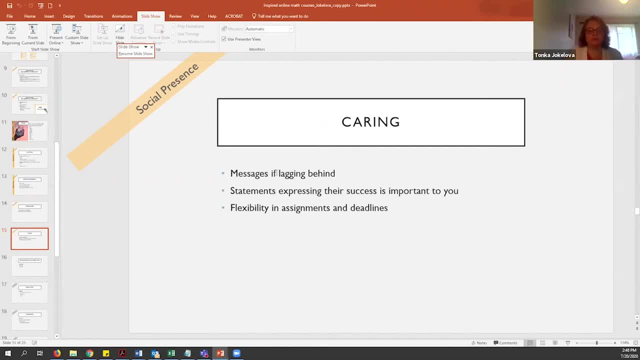 from from other students. well, also what i do when i have questions. um, i teach lower level, lower level course, so other questions are quite multiple in that in that course i post and ask a question. discussion: i haven't asked a question at the beginning and many times student posts to. 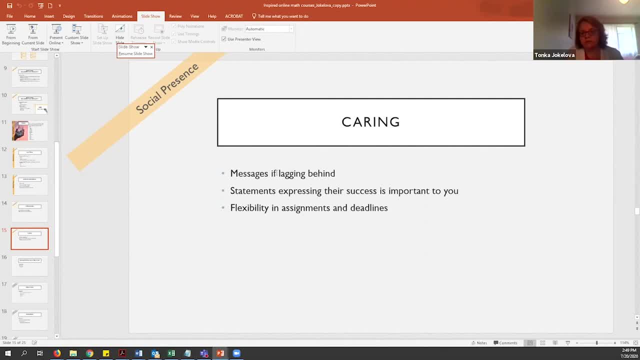 that discussion and then other students who already read the syllabus and who already know the guidelines they answer to to the fellow students, right? so it's uh, it's kind of a gateway thing to the student to answer questions in that way. so i have a few questions. 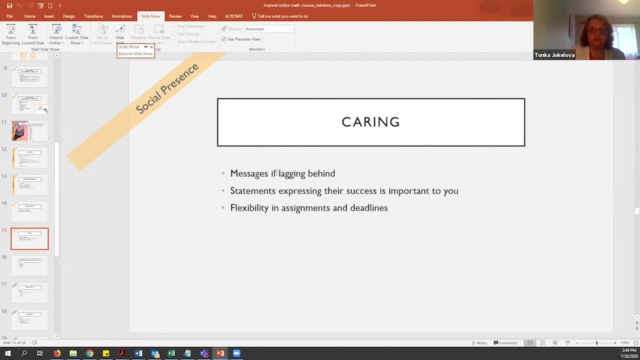 that they have for me about how i see the three ways that you know, i've seen students respond to the three measures i have. one is what is the need for student interaction and the other thing is what is the need for student interaction by using the three measures with students. 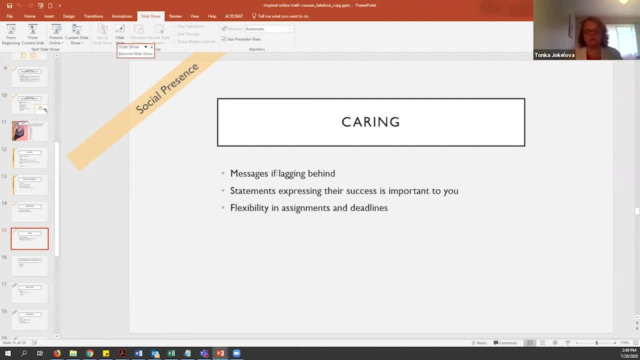 and so, and i have three questions for you about the right way to respond. i have a few for students, but i have a few questions that you need to answer first. of all of my attention is on one student, then it's not benefiting the others, so for 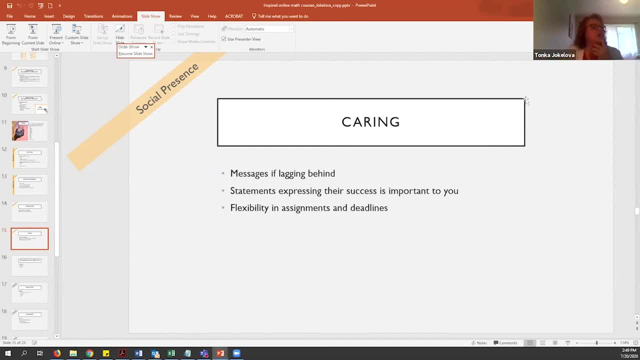 sure, I draw them. I draw the line in messages. all right, all statements that express that, express that their success is important to you. many times an announcement if you just sneak in little sentence like: hey, it is very important to me that you finish this course, it is very important to me that you learn what? 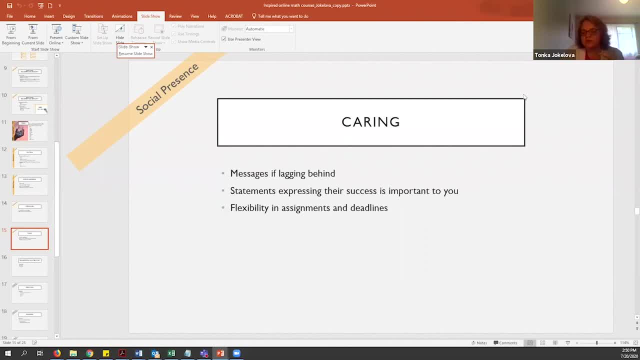 you came here to learn, so please, if you are, if you are seeing something that is not clear to you and you need more explanation, let's shoot the email out to, or the message to the entire course, or email me if there is anything I can help, and then we'll see if there is an extra tutoring session that we need to have. 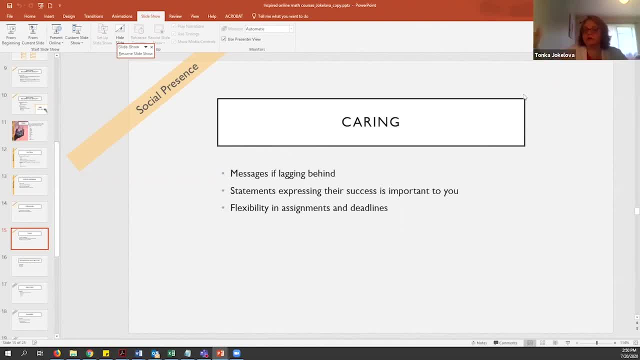 not just probably a student with the instructor, but maybe a group. as a group I have, I have APA sessions quite a lot. you know, I have APA sessions quite a lot in my course because, for some unknown reason, students have very difficult time with APA and I just say, okay, well, I'm seeing a couple of students emailing me. 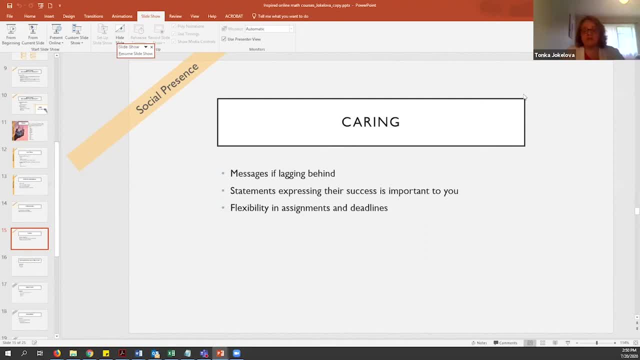 about, about difficulties with APA. so let's have a live session on APA. so we have. we have one hour session where I kind of show them the basics of APA. so just make sure they understand that they're not just a number and you let them know an announcement in messages in any of your communication that it is. 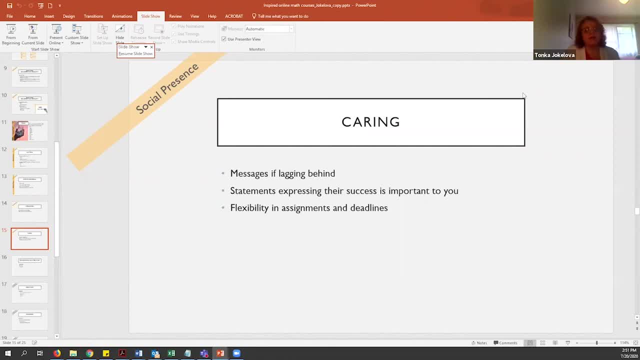 important to you that they are successful in in this course and also be kind to yourself and to your students. everything will be new for a lot of us coming fall. we don't know what. we don't know yet because the fall will be such a different animal for anything else that we have experienced. so there will be. 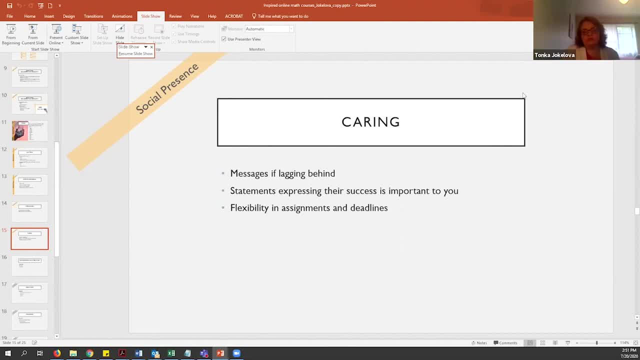 issues, just like we already talked about. there will be issues with Internet, there will be issues with with devices. there will be all kinds of issues. so try to be flexible in the deadlines. try to be flexible in the silence. just show the. that's one of the ways of showing that you care. 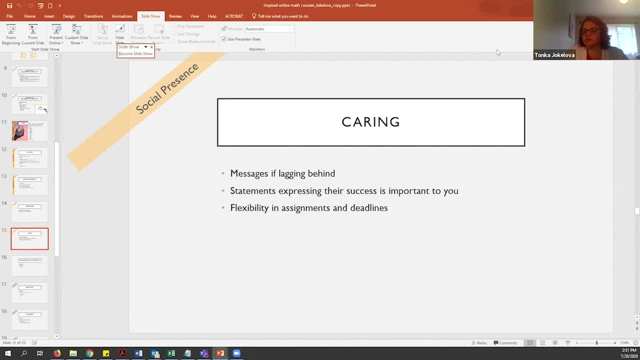 when you are flexible And if you are able to have students pick their own topic, then that's great, If you are even able to let students pick their own assignment. So let's say you have a selection of assignments. you have, let's say, five assignments. 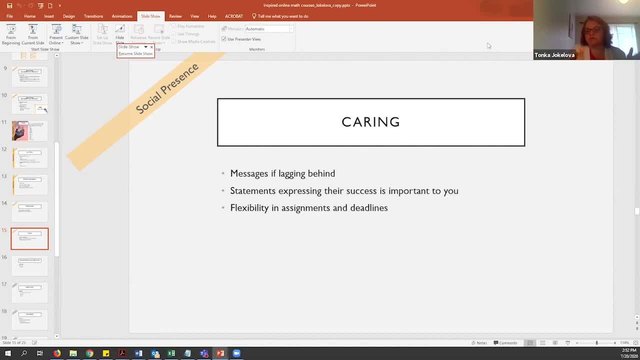 and out of those five students can pick three to complete. So there is a little wiggle room and a little flexibility, which makes the learning more relevant to the student, because you always want to engage more with the content that you're interested in. 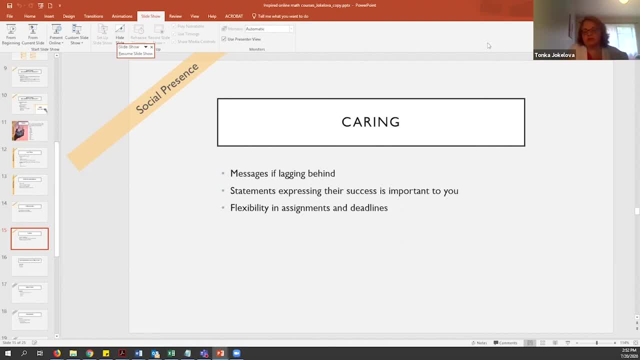 So if somebody is making you complete an assignment that is kind of lukewarm to you. when it comes to interest, you will put the lukewarm type of energy and effort into it. But if it is interesting to you you're more engaged in it and with it. 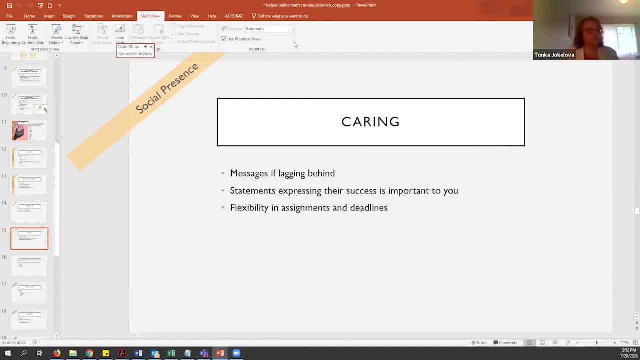 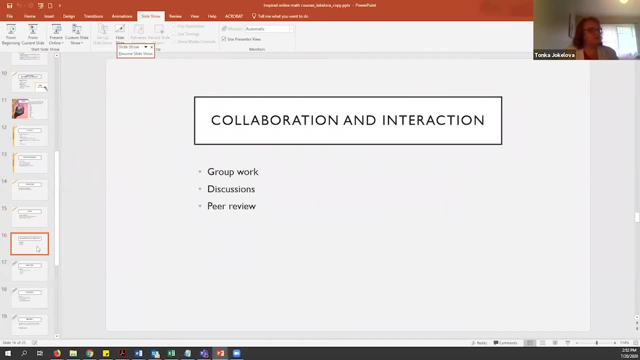 So, if you're able to- I know not everybody is able to select different assignments and different topics, but if you are, it's definitely going to work for you. Now let's talk about the group work and the discussion and the peer review that I promised you about. 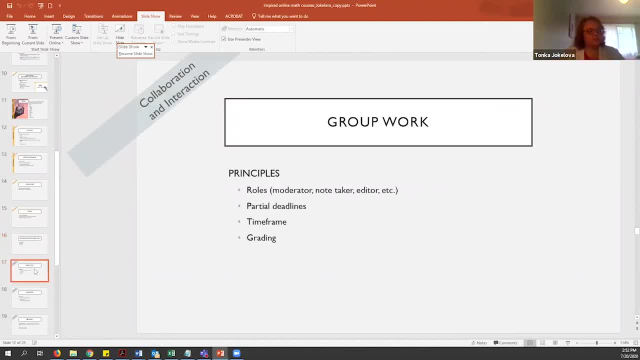 So group work: very important thing in group work is to be very structured in a group work because if you just tell them, okay, now working groups, they have no idea who's doing what. who's what is the function of me? 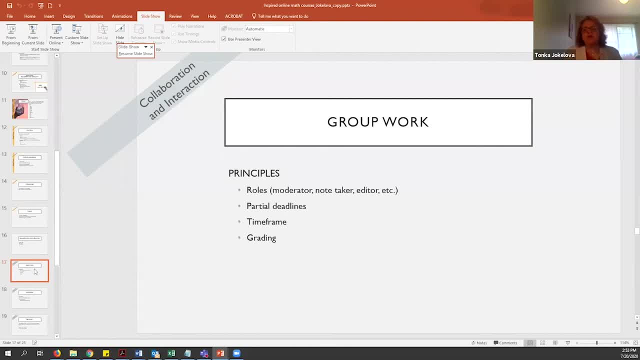 What are we supposed to, even? what's the purpose of this research? So, if you have very structured rules when it comes to end guidelines, when it comes to group work, especially in online environments, it will be very helpful to you. So, also, what is helpful is if your groups 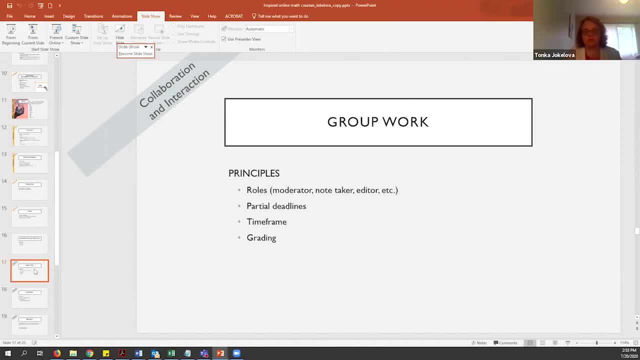 have different roles, So you can select who is going to be in what role, or they can self select in groups, excuse me, So it's very important to have a moderator. If the discussion is going off the deep end somewhere, the moderator will jump in and bring it back into. 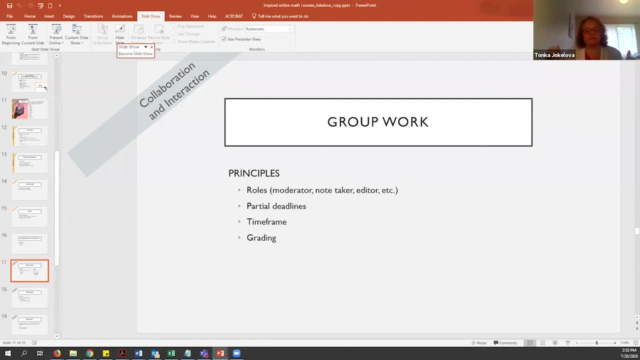 to the topic, If there is any. if there is any disagreement about the position that the group will take, the moderator again can jump in and kind of make sure that we are in in the limits. within the limits. The role of a note taker is important one. 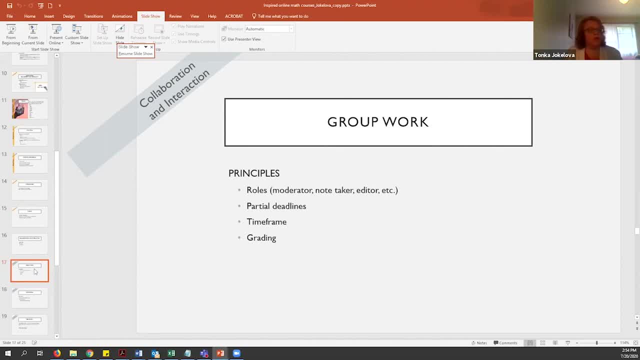 who is going to take notes, What is going, what is discussed And also, once the final paper or final product, or final whatever it is that we're creating, once that is finalized, who is going to be editing it? Right? So, if there are any other roles that you find, 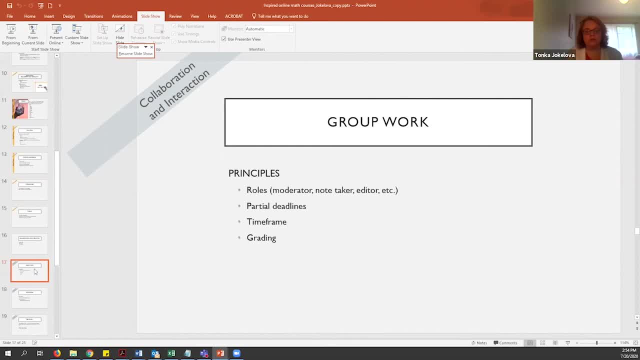 you find interesting and important for the group work, for sure use them, but at least those three are always good to have. So you can, you can- teach students. we will have those three roles And before the end of tomorrow I will need names for each group. 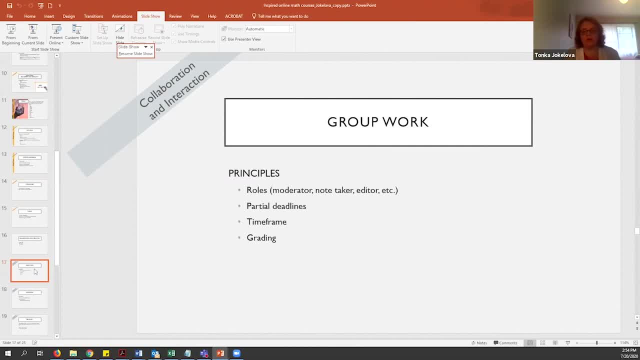 who those people are for those roles, so that you know who to contact. even So, if you want to contact the group, maybe the best way to contact the group is through the moderator right, Because they they are the ones who are going to be. 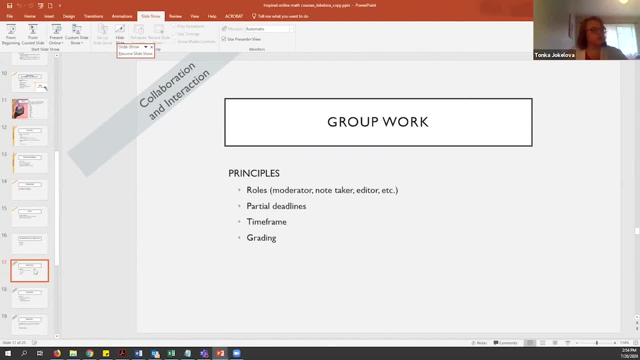 right Because they are. they're kind of holding the group work together. So roles are very important. Partial deadlines are very important. You cannot just say we're going to, as a group, you're going to create a 20 page paper. 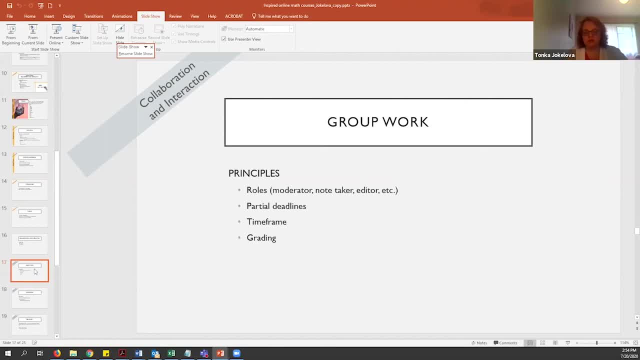 and it's due September 1st. It's, it's. it's not that helpful. What is helpful is if you have the project divided into several steps and then the first step step will be due- I don't know- August 12th. 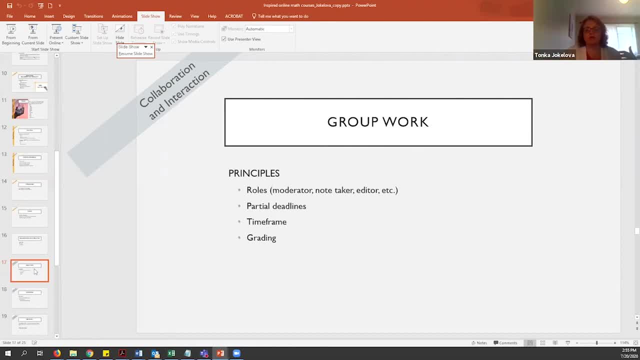 And then the next step will be due August 17th. until you get to the final, you know- project, you will get better results And there will be more of a engagement happening and more of a learning happening. Time frame, of course, is very important. 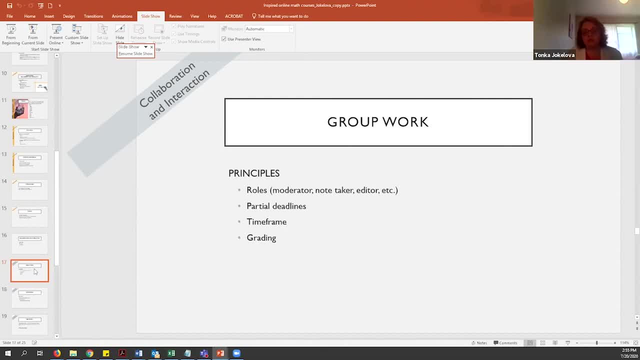 Scheduling time frame, And what you need to decide before the group work starts is how are you going to grade it? Are you going to give everybody in the group the same grade? Are you going to grade based on their contribution? And if they are going to be graded, 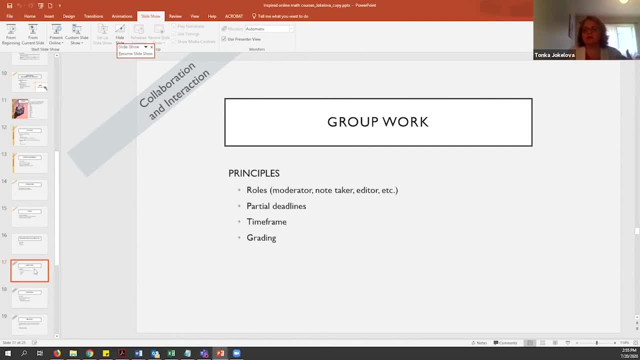 based on their contribution. how are you going to get that amount of contribution that everybody, everybody, had? So are you going to, are they going to submit? submit any kind of statements stating that this person was contributed the most? this person was lacking? 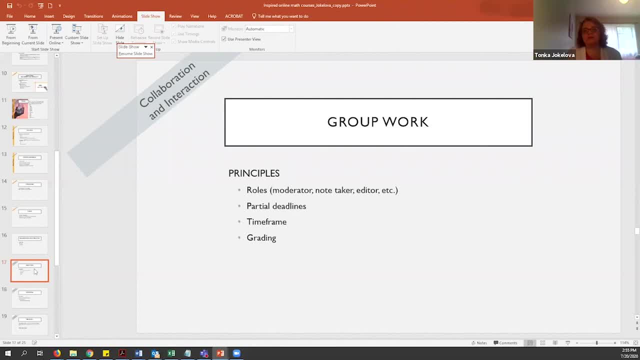 this person something or another. how are you going to deal with that? And again, there is not right or wrong answer. There is just what is your preference and where you are when it comes to your teaching. I've been in groups where everybody got the same grade. 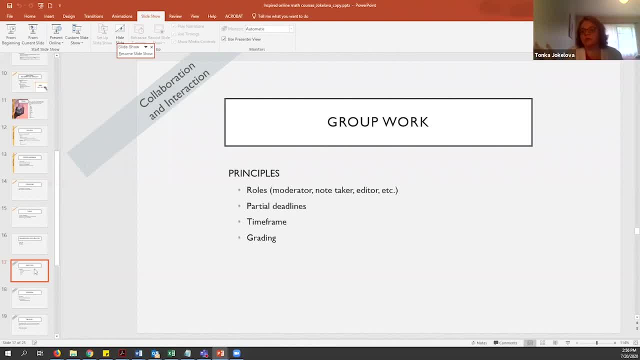 and I've been in groups where everybody had the grade they deserved So and I was fine. Well, so it's really up to you to decide. just know that you need to know that beforehand so that, so that you're not stuck. 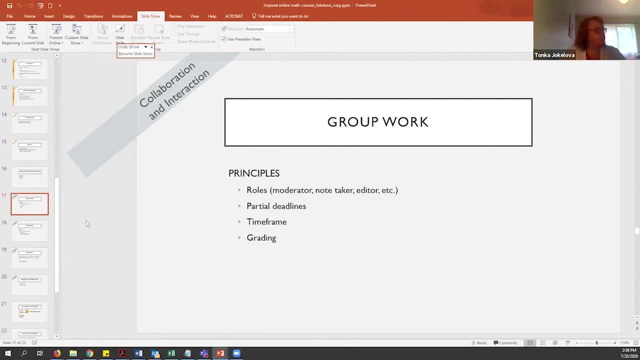 towards the end of the group work, not knowing the grading, how they're going to be graded, So I'm just going to give you a warning. We're about five minutes from three, Thank you. Thank you, So we do have only two more things to talk about. 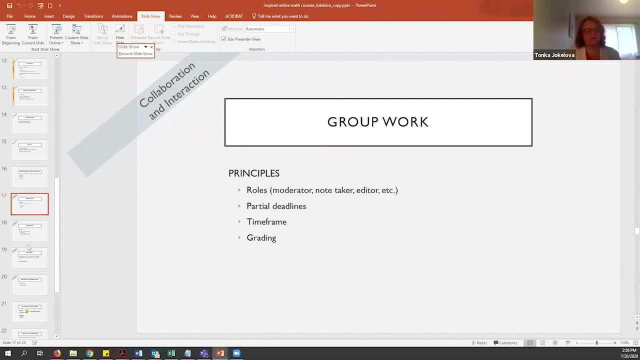 before we run into the grilling and egg and the whole thing with with, with the grilling. So let's talk about the discussions. Discussions, I know you're going to say: well, in math there is no such thing as discussions. 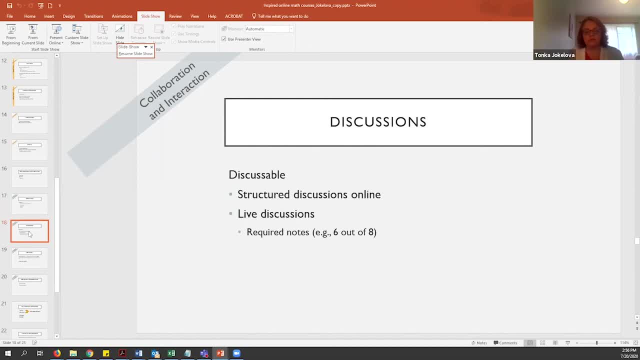 Well, they can be. there can be for sure, And they can be. discussions in math are probably need to be more structured than anywhere else, Because if you are discussing- Abby gave me an exact, a great example- You have four people at the dining, dining table. 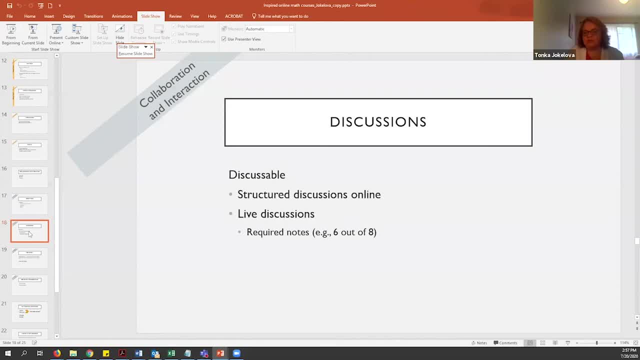 What are all the combinations that can be seated in and what combinations that can be seated right. So if you have a, a problem that is only a numbers problem, you can translate it into real world and make it a discussion. So the post, the first post, can be create a scenario. 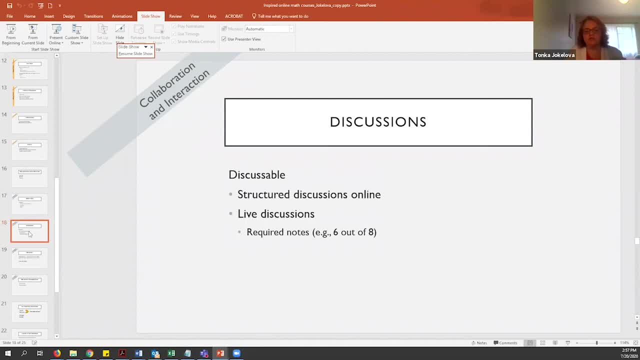 So somebody can create, as, as your student can create a scenario for for the class. The second post might be okay. so now tell me exactly how, how, the how the people are going, what is the combination, How the people are going to be seated. 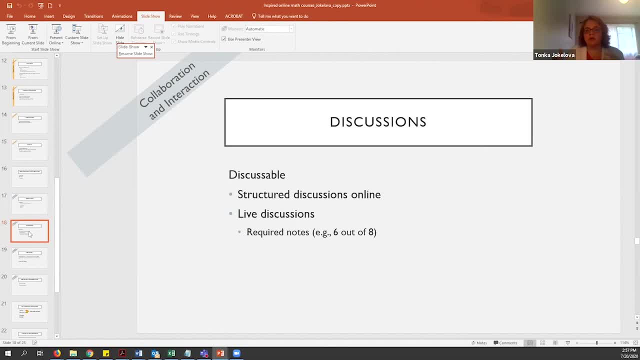 And if you have mathematical calculations, we need to know exactly how you came into into the result. So it's not just there are 1200 different, different options. That's not. that's not good enough. I need to know how you came into this conclusion. 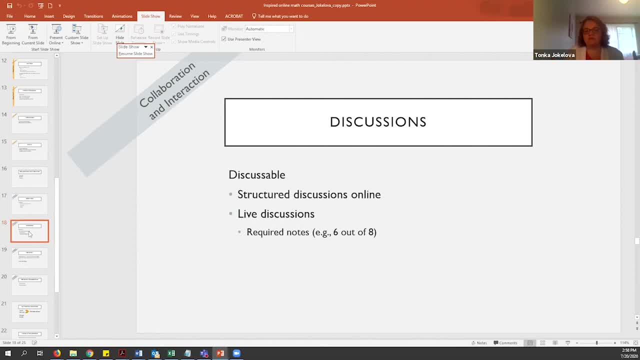 And then post number three can be. so, now that we have this, this problem, solved, what are other uses of this particular technique or this particular strategy, or are there any other spin-off problems from this one that you can come up with? So so, for example, the first post can be due by: 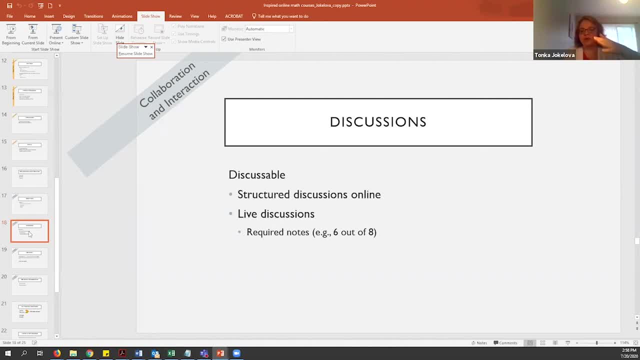 I don't know- Tuesday night, And then the second post can be due by Thursday night, And then the last post can be due by Sunday night. So here you go. already you have the discussable discussion for for an online course. 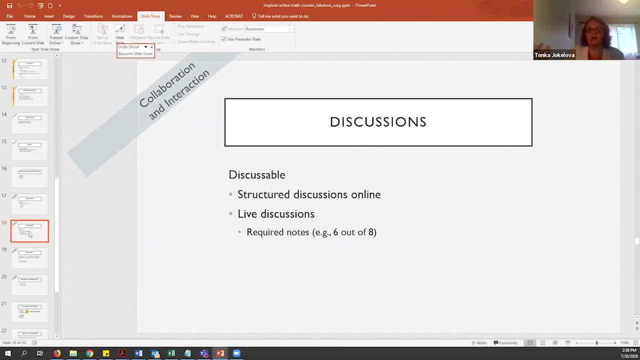 So always think about some practical ways: how to how to get students to learn, whether you're trying them to, when you're trying to make them learn, I guess- And also what is good to have, and we already touched on it a little bit at the beginning. 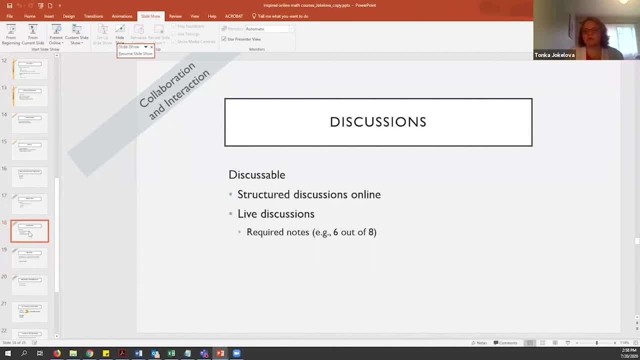 have live discussions if you're able to. I know some colleges already have their modalities figured out. some probably do not. If you are able to and your college is allowing you to, online synchronous sessions are a great engagement tool for your students. 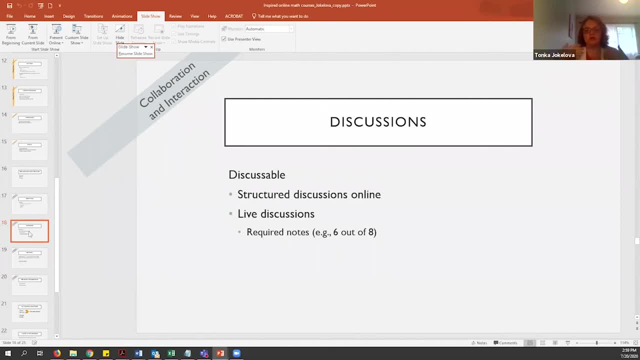 The student is able to ask questions to you. They see you as a human being, They see you in person. So if you are able to do that, please do that and do that often. Sometimes also, what I heard- one mathematician actually was saying that she has 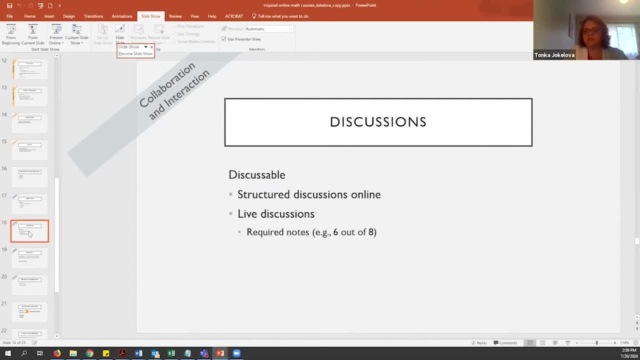 she has the live discussions and she's requiring the students to take notes during those during those live sessions, And the students are then required to submit certain number of those notes. So let's say we have eight live sessions during the semester, six you have to take. 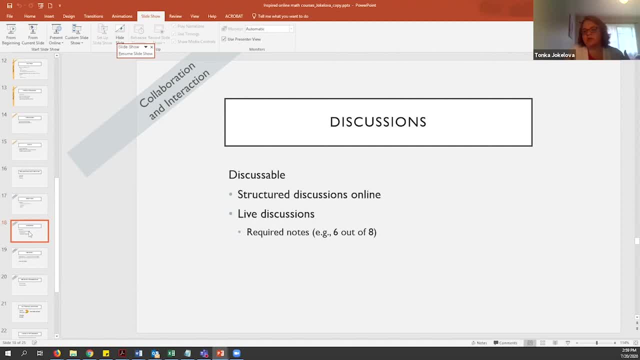 You have to submit as as notes. So that is also some motivation that they will attend And it's also learning learning tool. just to just to note what happened in in the live session And what we learned what was discussed: 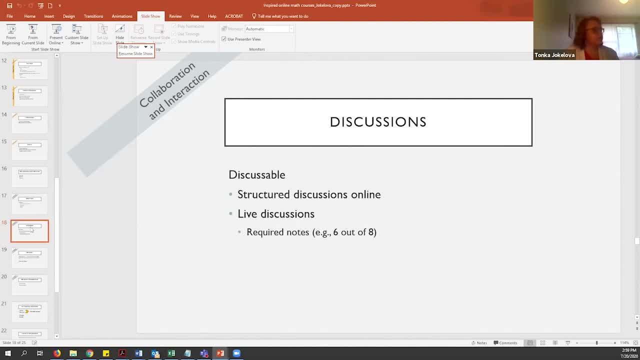 was there any problem that was discussed? How was it solved? So all the discussions that that have that can happen in math really should happen in math because, just like I said that that engagement with your fellow students and with your instructors are two most important things. 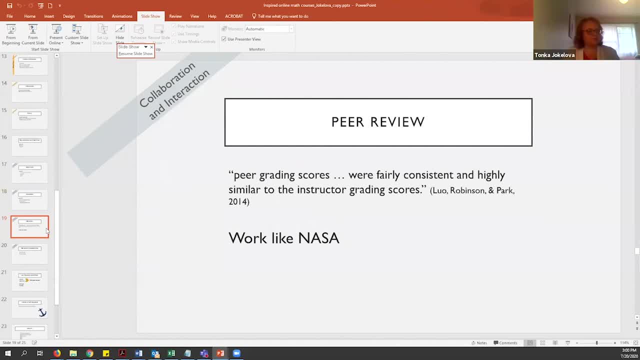 that can happen in an online course. And the last one and I get, I have another, another little research tidbit and I'm going to be, and then we're going to talk about X and then we're done. So a little research tidbit is sometimes. 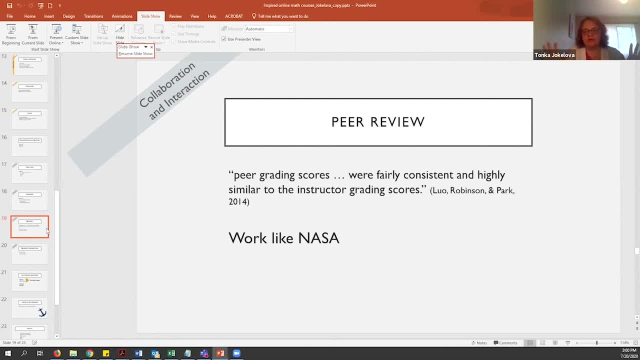 even I sometimes look at peer review like, well, students don't know how to grade And I cannot just ask students- you know students- to grade other students because they don't know. So I looked into the research and I looked into literature. 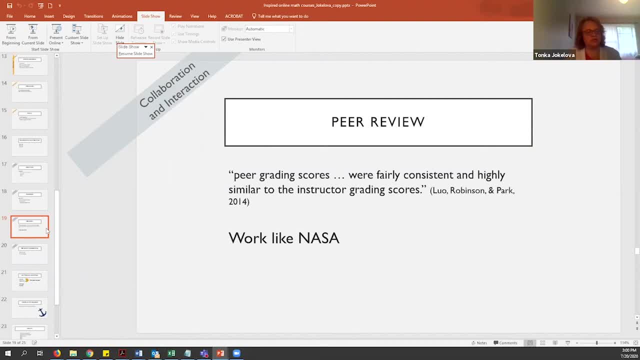 and I found actually quite several studies saying that scores that peers give to peers are actually fairly consistent among each other and are very similar to the scores that the instructor would give to, would give to that particular activity. So, peer review some, some strategies you know. 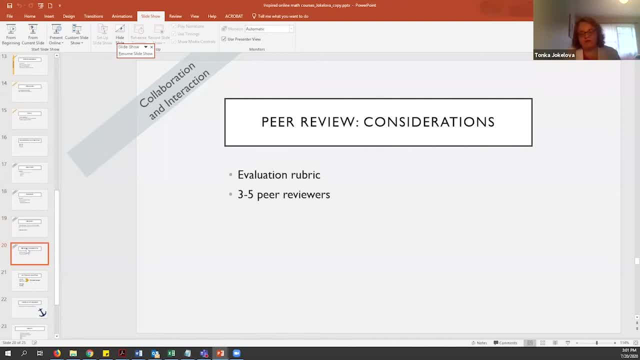 for peer review. uh, that you have to have considered before you before you create a peer review assignment is: have a rubric. the rubric has to be very specific so that the students have something to grade it on. if the student does not have rubric, there's no telling what they're going. 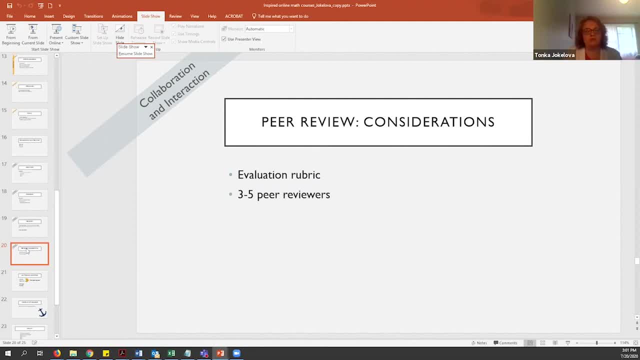 to grade on. so if there is a rubric, that is very good. good tool is the rubric for for the rubric to be fillable so that the student submits not only the final grade but also the rubric that goes with that assignment. so evaluation rubric has to happen before before there is any good peer. 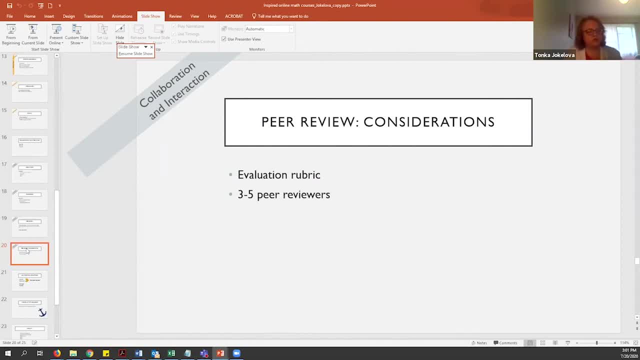 review, and a good amount of peer reviews, will be three to five per student. uh, if one student peer reviews one student, it's not not as reliable as when you have three to five students grading or peer reviewing um peer reviewing another student. so have those and just like in nasa. um, we are not. 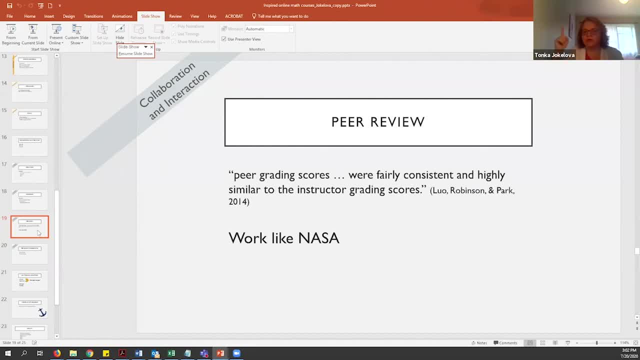 sending people to to space just based on one calculation right. everybody calculates and recalculates, others calculation. so i work like nasa. i have students work like nasa. have somebody calculate and recalculate and also when you recalculate it can be a part of an assignment. the recalculation can you come up with. 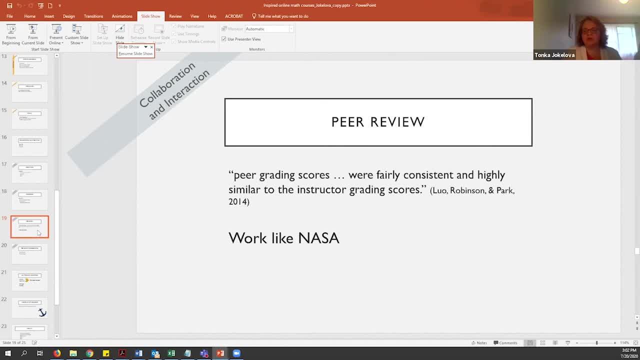 different technique, how to get a strategy, how to get to the final answer. so that can also be working in your discussions. you know, just come up with different strategy on on solving the particular problem. and not only you have. you have content sharing, not only you have content learning, you also have. 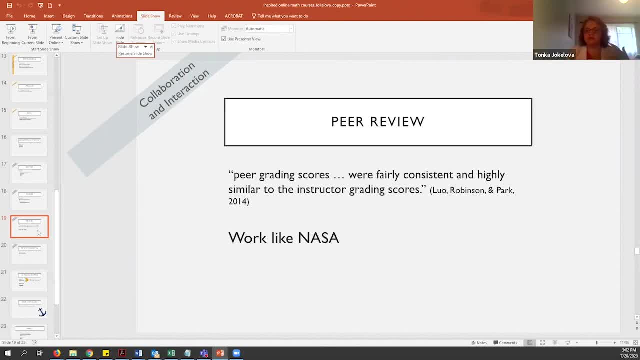 peer mentoring. when it comes to peer review, you are you as a student, are mentoring your other students like, hey, did you think about, about solving this problem in this kind of way? what about different problems? so do you think that will work with that problem set, so you can create you. 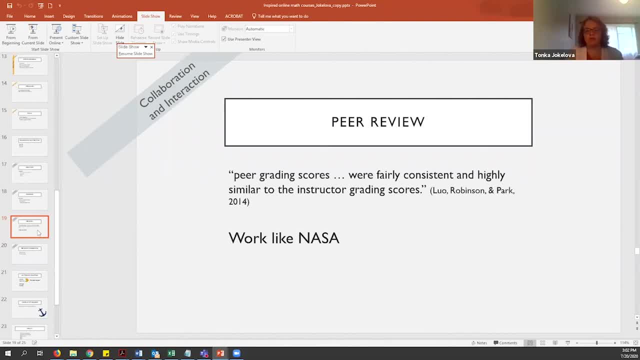 can create discussions with peer review combined, where students are helping each other and, uh, staying engaged- number one and learning well, not number one- learning and staying engaged in um in the process. so, uh, peer review, discussable discussions and group work are definitely great engagement tools when it comes to, when it comes to online online course and 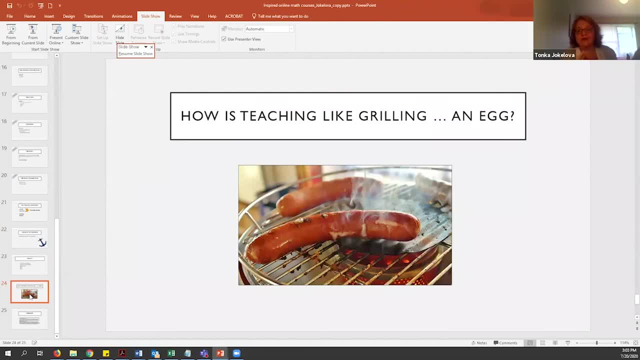 before we, before we wrap up, i want to come back to to my grilling experience. so how is teaching like grilling an egg? so you cannot just bring an egg to the grill and just kind of pop it on the grill and call it a grill. that you cannot. if you open the gra, the egg, and it's uh, you try to grill. 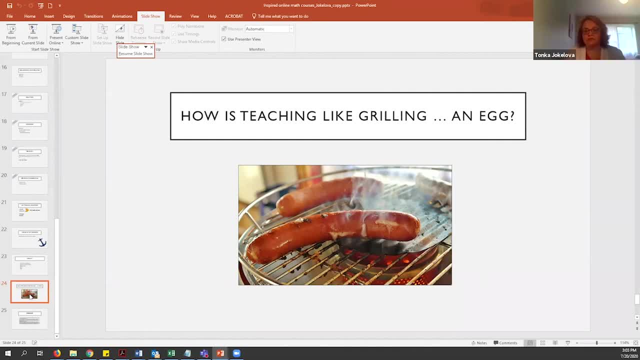 it that way, it's going to run through the, through the grill, onto the, onto the charcoal, and no good. so you're trying to grill an egg. what you need to do, you still can't do it, but you have to do it on an extra pan, right? you bring in a pan from the kitchen with you and that's where you crack the. 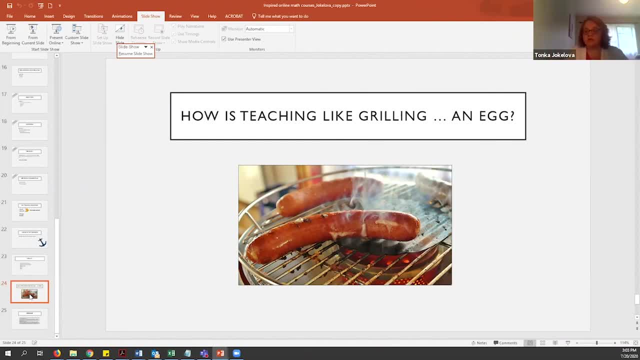 egg and for the pan on the grill. so, yes, you can. you can grill an egg. however, you have to have a special tool, not special to, not special to a pan, but you have to have special tools to grill an egg. You have to have a tool that is appropriate for the process. 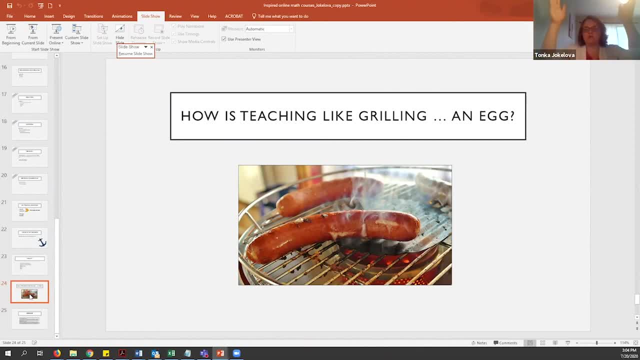 And teaching is very much the same. You know where you're going to, You know what you are supposed to be teaching, You know the learning objectives that your students are supposed to arrive at, And will every single strategy work for that? No, 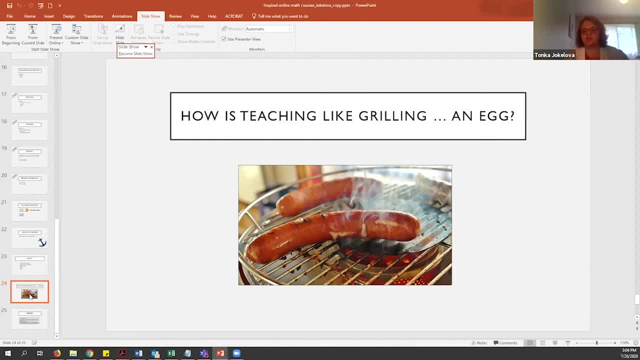 You will have to choose what will work for a particular problem that you have in your course. So again, always have the learning outcome in your mind, Always know where you're going With the course, And you do because you know what to teach. 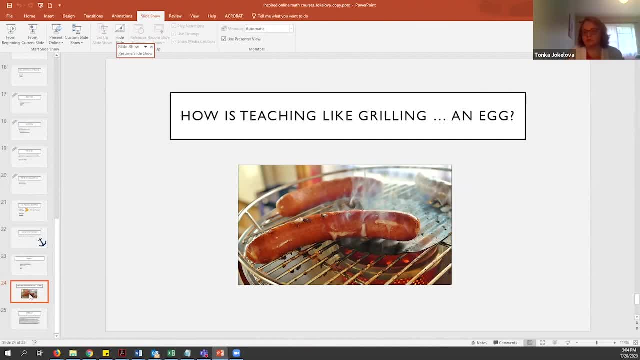 But then again, there is a magic in choosing the right tool, And the right tool might be live sessions, just like we talked about. The right tool might be: if your students are not that engaged with each other, might be some boost in social activities that we mentioned. 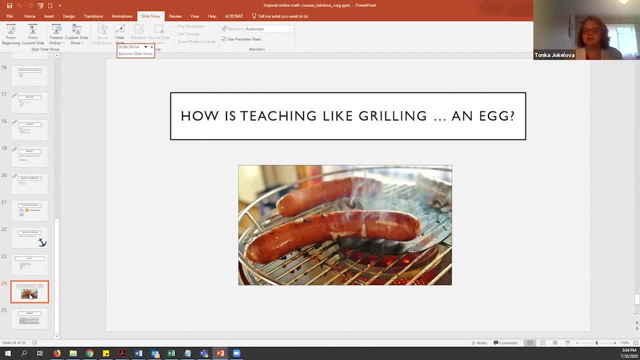 It might be some discussions, It might be other things that you're going into. So when you, as an instructor, think about how you're going to approach your course, always think about, When you are teaching, what is the best way to teach that and how you are going to engage. 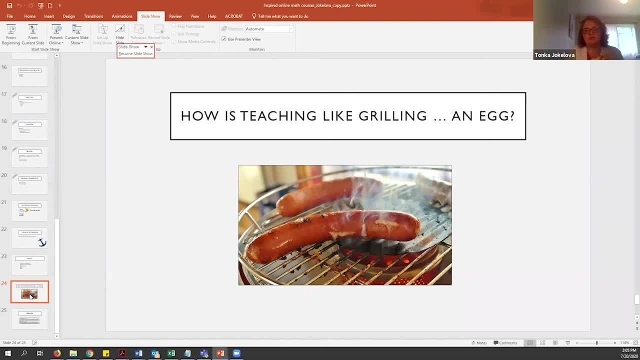 your student and how you're going to show them that you care, Because, remember, student-instructor relationship is the most important, especially in an online course. All right, What questions do you have that we haven't. Thank you, Tonka. 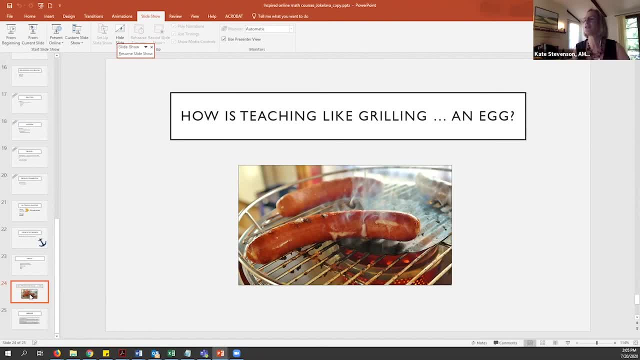 So we've got one from Heather. So, due to reduced classroom capacity, half of my students will be attending in person and the other half will be watching it synchronously. Do you have any Any suggestions about how to split the class into groups, given that division? 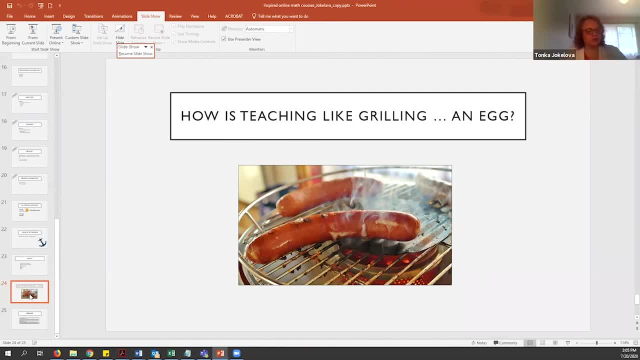 So I've heard different things, that people are doing different things. I've heard of college who is doing And everything has pros and cons. So one college is doing cohorts. They have two cohorts and they're switching them around. So one week one cohort is in person. 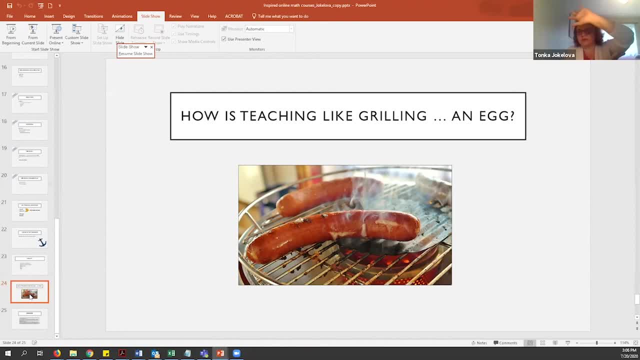 The next week the second cohort is online And then the cohort that was in online is now in person, right, So they're switching, They're switching them around so everybody can have their fair share of online and in person. Then I've heard another college is doing sign-up system. 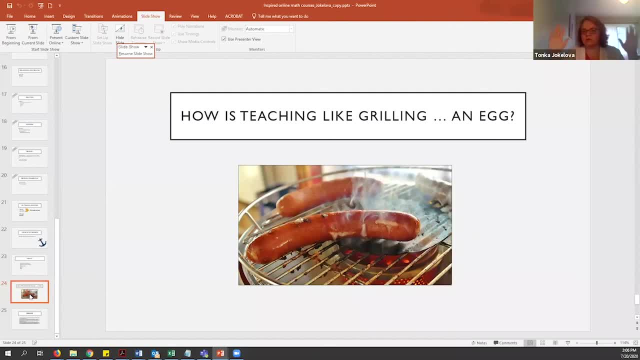 So they have a sign-up and there is a certain limit on classes in the classroom, And whoever signs up to be in the classroom first comes, first serve kind of situation. So they work there too, Then we're, Do you have? 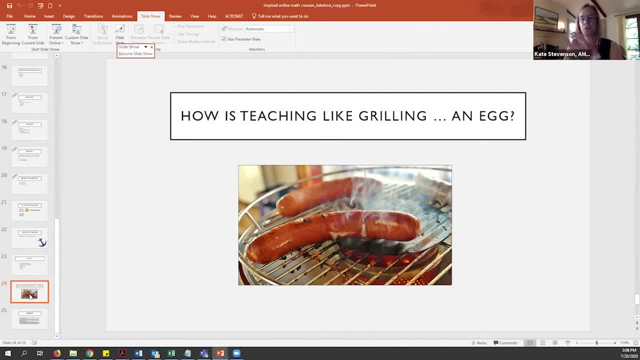 I think she was talking about. given that you have these two different groups that are coming and going, do you think you should? Do you think you should blend them in creating group work or do you think you should separate them in creating group work? 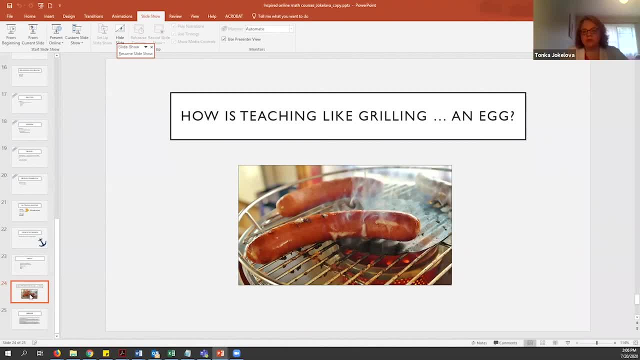 I would definitely blend them and I would use online component of the course to do a lot of that, because many times they're not going to be seeing each other- seeing different groups, members of the other group- right, They're not going to be seeing the other person. 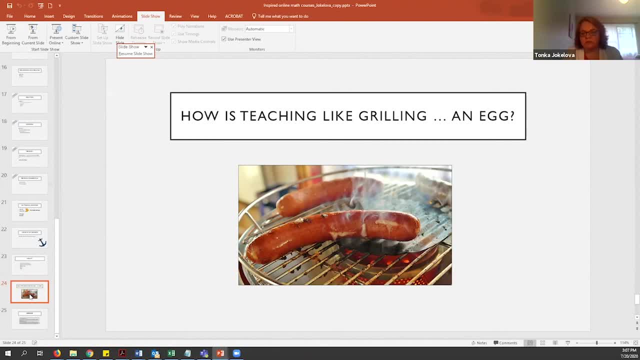 So I would definitely use online to do that and I would definitely blend them, because then you, If you don't, then you are creating really two classrooms within one classroom and you don't want them to be together. And if you're teaching in a flex or high flex- what we call high flex environment, that's. 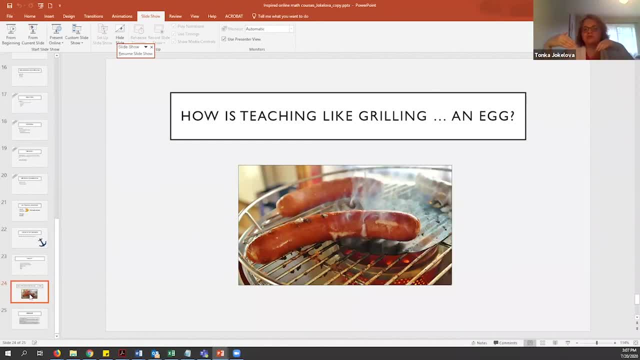 the same thing. High flex is when students are able to choose how they're going to receive the session. Are they going to be in person in the classroom? Are they going to be streaming it? Are they going to be watching later at night? 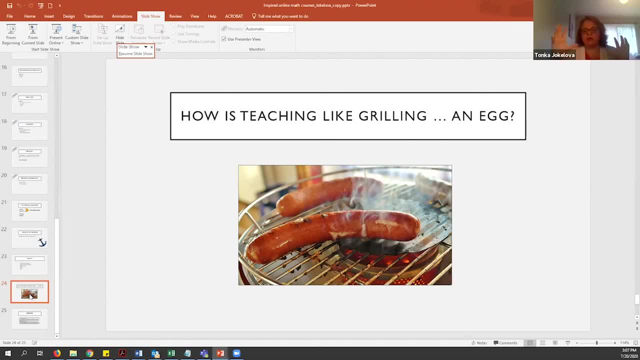 So they can choose. They can choose, And In that situation I would group them as well, I would make them work together so that there is this cohesion, There is this: I belong to this, And I don't only belong with my four people, but I belong in the entire classroom, for 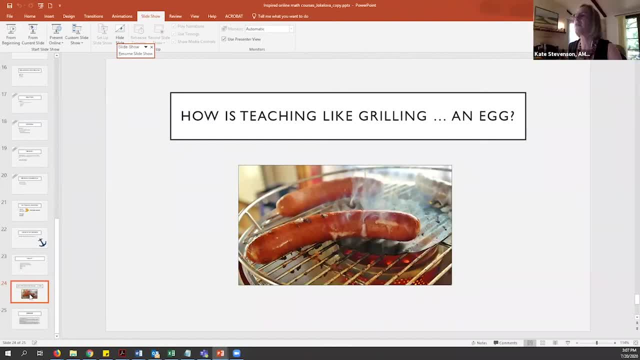 sure, Right? No, that makes a lot of sense. I think that we've hit all the other questions, unless there's somebody who would like. Oh, there's one more. There's a thank you. If there's somebody from the audience that would like to ask a question, I can. 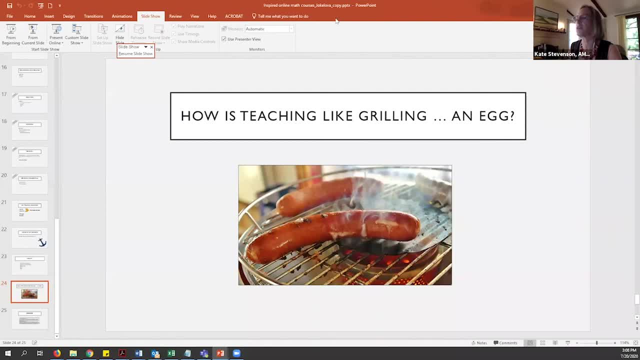 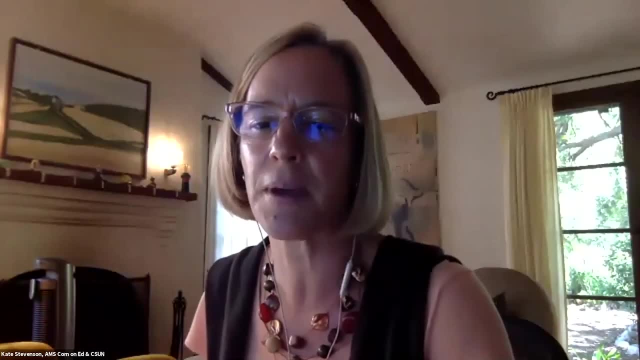 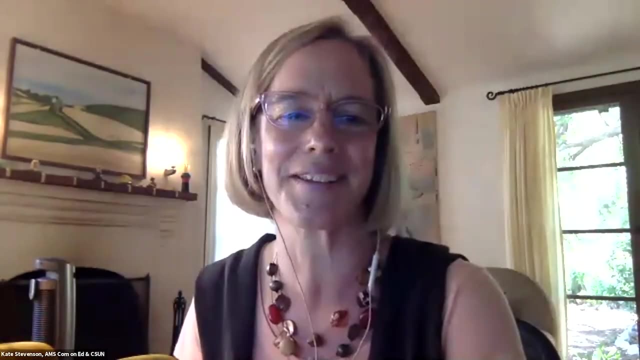 I can hand you the microphone if there are any questions, or you can type your question into the Zoom. Otherwise, there was one question about avoiding Zoom bombing that I actually answered, but maybe you have a better answer. The answer we get is: use a password and use a link that's not your open Zoom. have one. 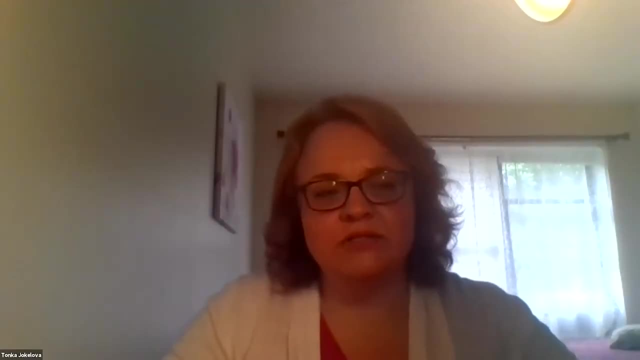 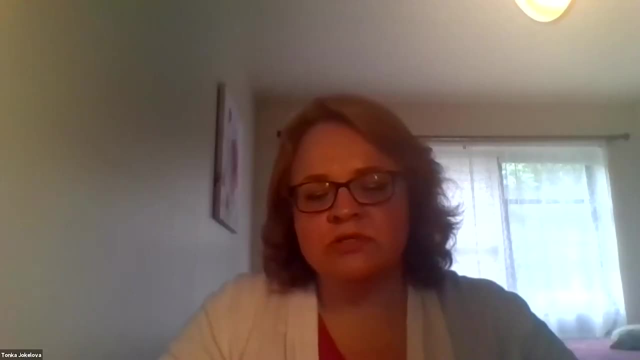 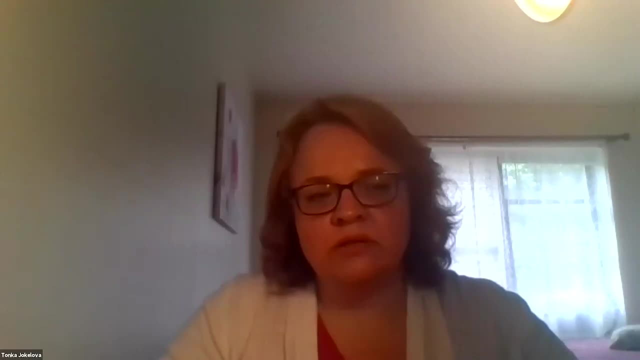 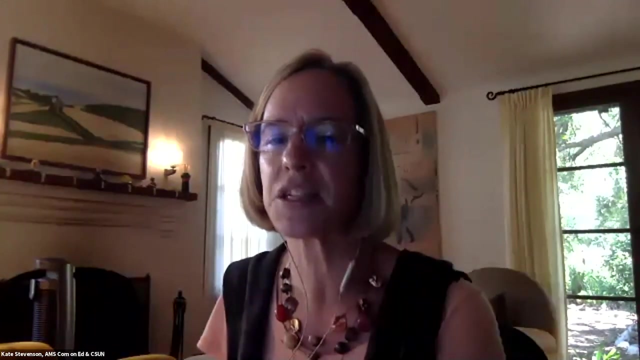 Right, They also use Teams, so there is no issue with that either. But for Zoom: yeah, password is fine. yeah, Okay, I think that may be it. I don't see any more questions in the chat and we are past time.